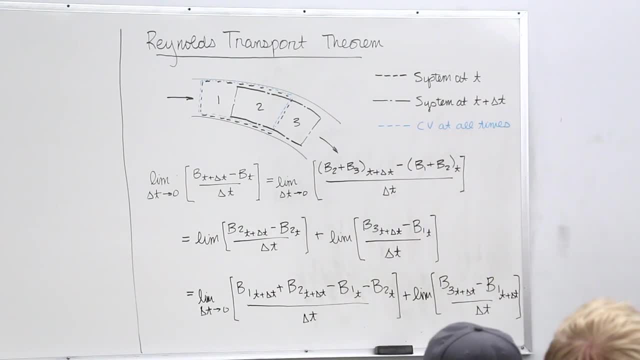 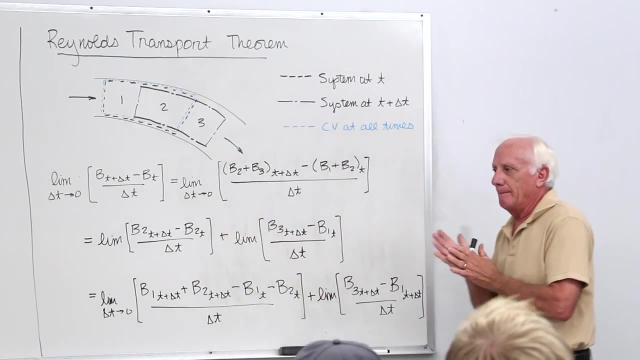 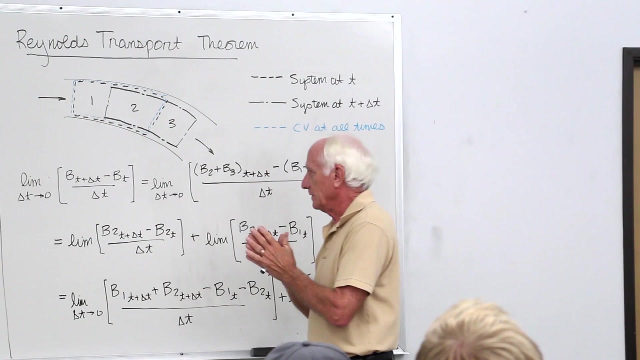 is a fixed region in space, the blue dash lines And this should be in your notes. We're looking at any variable B. B can stand for energy, It can stand for momentum, It can stand for mass capital, D It's some variable. We're following the system at time. delta t. 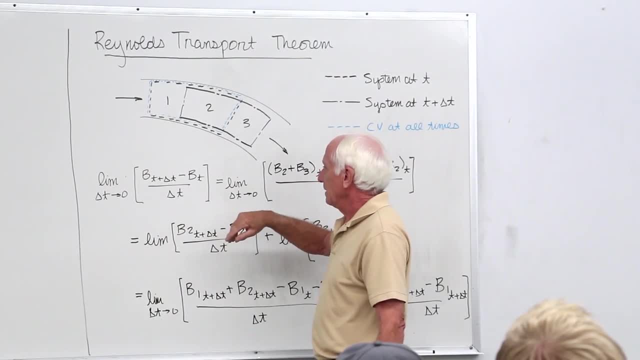 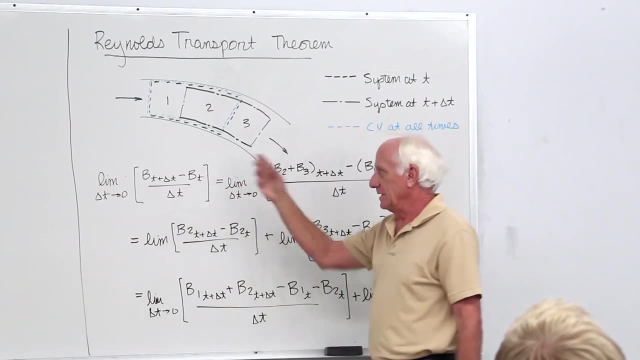 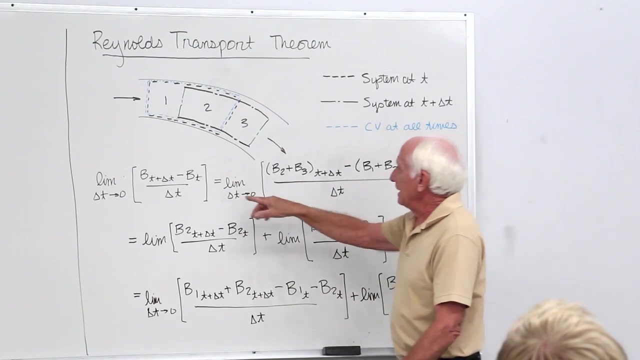 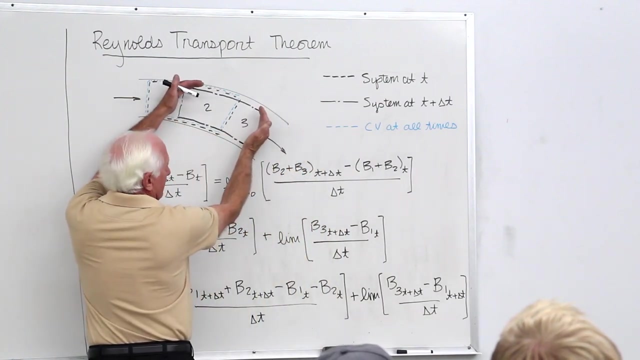 So we want to know how B changes. So it's B at time t plus dt, minus B of t over delta t Limit bit delta t goes to zero. That's how B changes with time in the system. So we break that down: The amount of B in the system at time t plus delta t is two plus 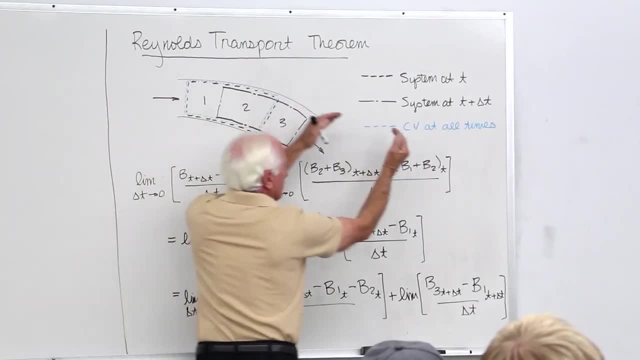 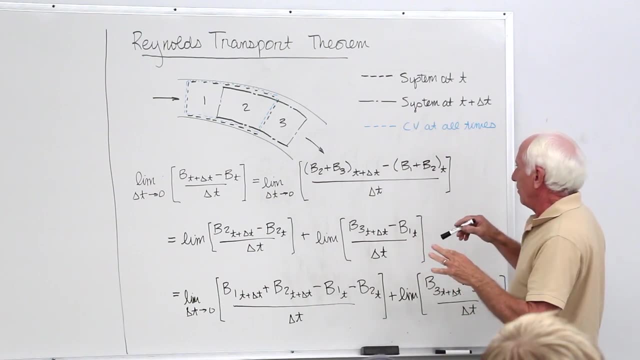 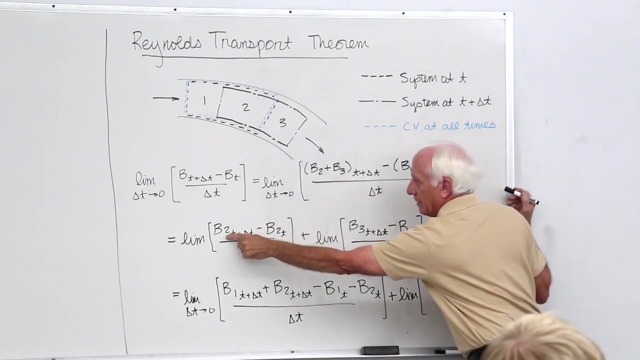 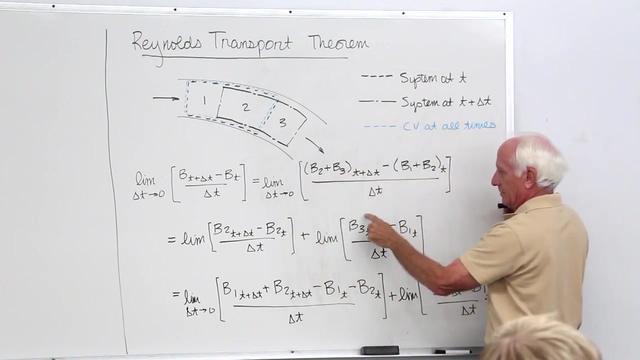 at time T is this 1 plus 2 here. Now we arrange the terms: This is a B2, here is a B2.. So put that B2 down there. put that B2 down there, That B3, right here goes. 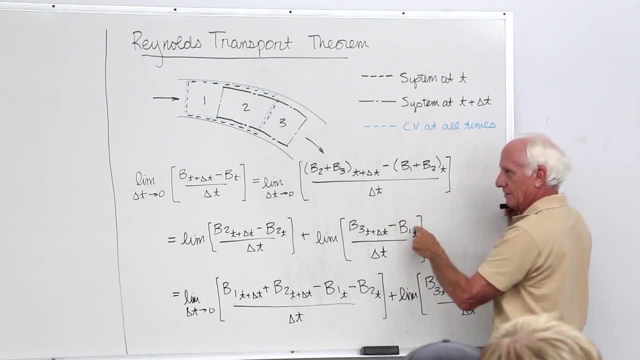 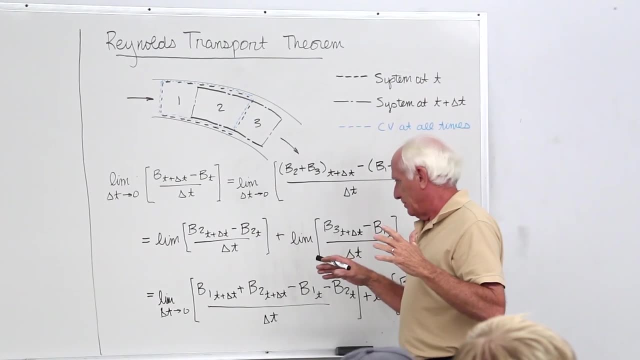 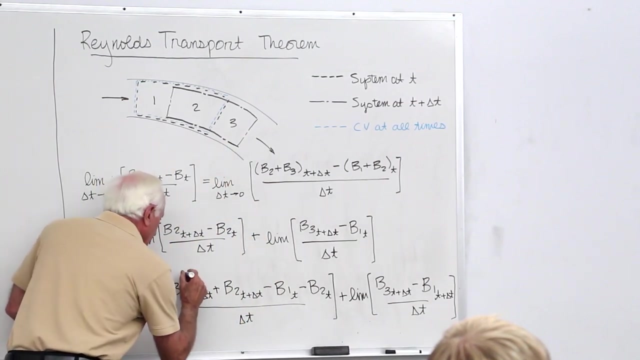 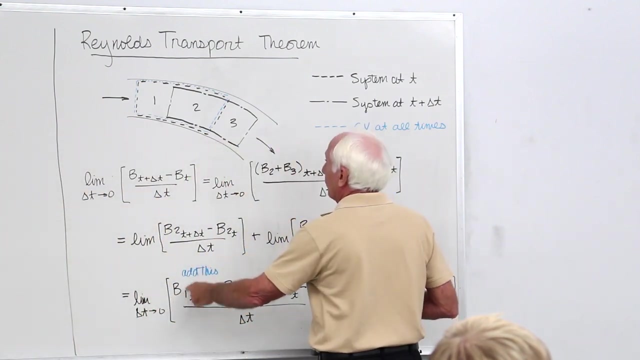 down here. This B1 here goes down there. I just move the terms around. I think this is a step I did for the board for the last time We're going to add this term, add that term B into 1 at time, T plus 1 to T. Now, if we add it, we're. 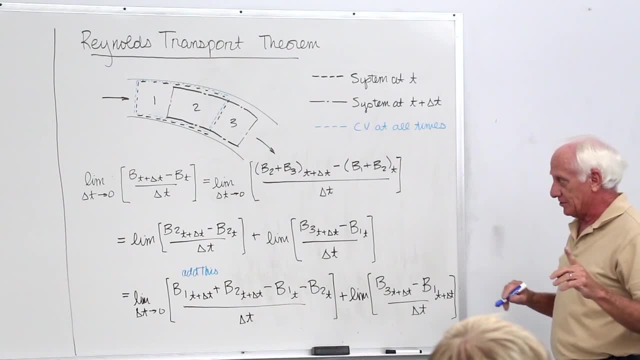 going to subtract it. We have to subtract it or the equation will change. So we add that term here: B1 T plus 1 to T. We subtract B1 T plus 1 to T. We didn't change the equation. We add this and subtract this. So we didn't change the. 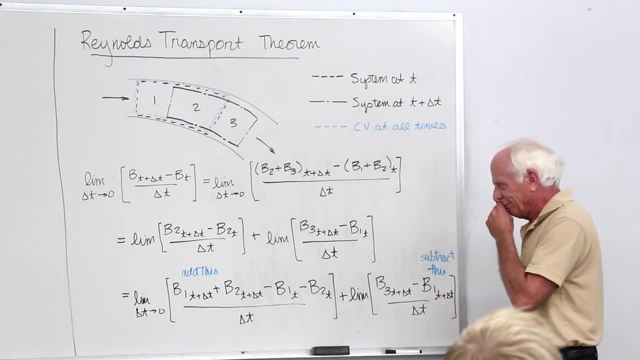 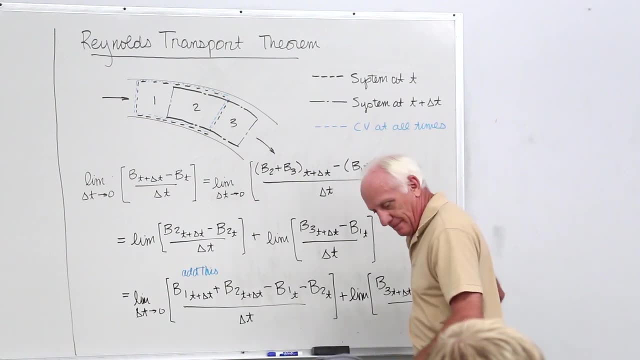 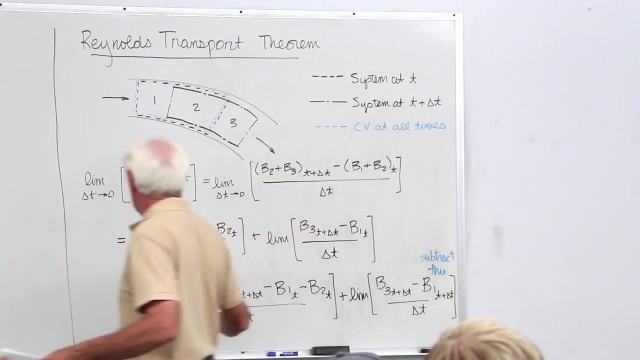 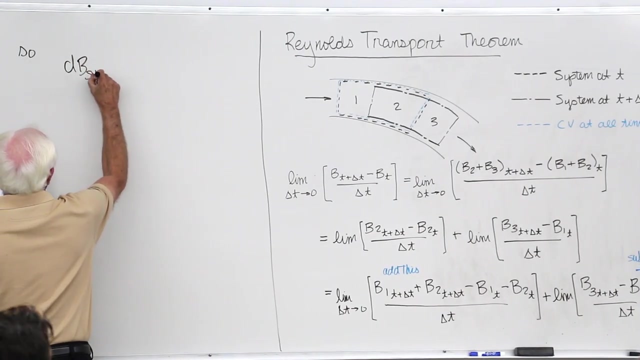 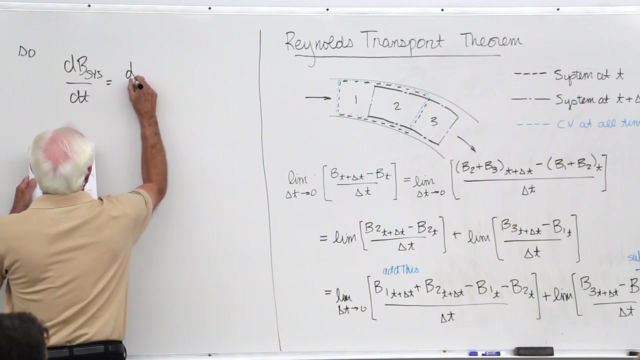 equation, We added and subtract the same thing. Then the next step, which is the one that we ended up with, is this integral here this first one- We have G B system with respect to time- is equal to D B time integral control. 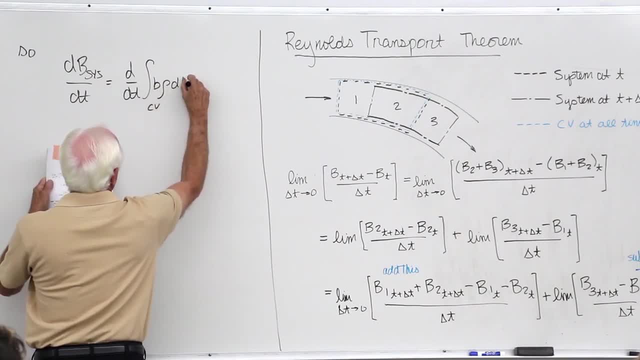 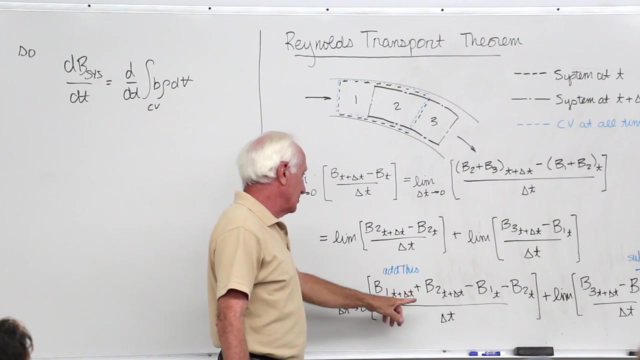 Subtitles by the Amaraorg community volume little b, rho dv. This is how the quantity v shades with time in the control volume. control volume of the gluon. okay, That's this term right here. Okay, how much energy, how much b was in the control volume at time t, at time t? 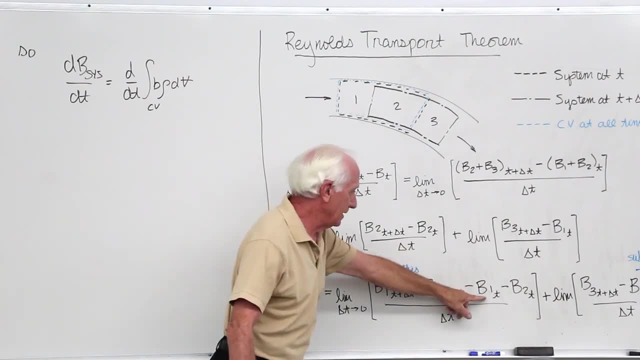 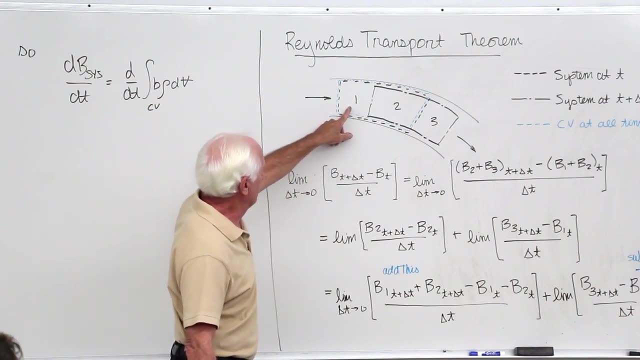 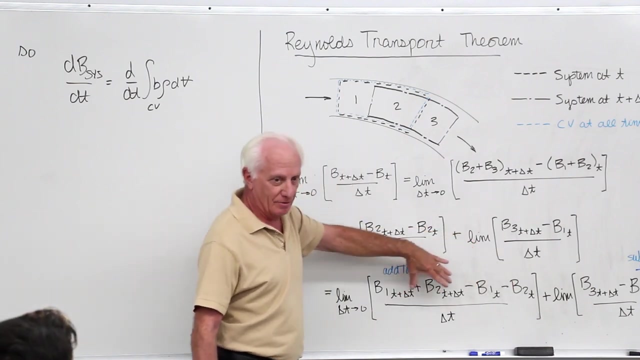 B1 plus region 2 here at time t. okay, At time t plus dt, how much b is in the control volume? B1 plus 2 at time t plus dt? This is the change in the amount of b in the control volume between times t plus dt and time t In the limit as delta. 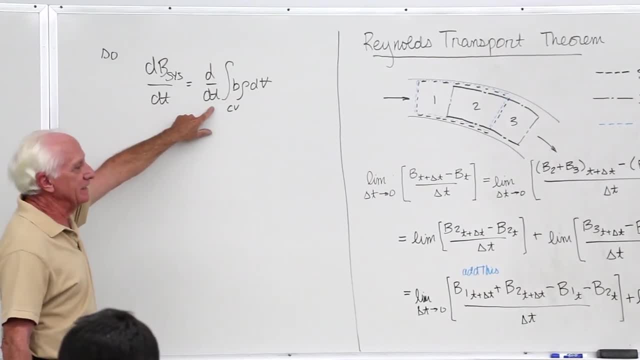 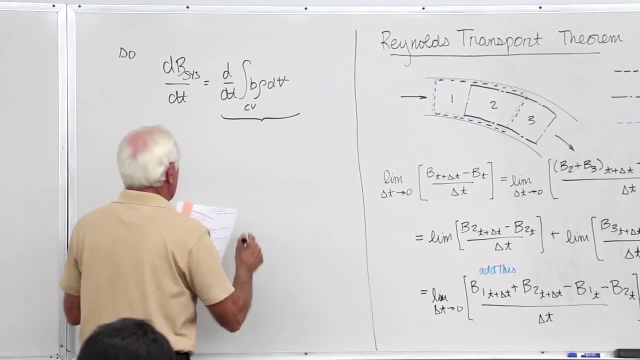 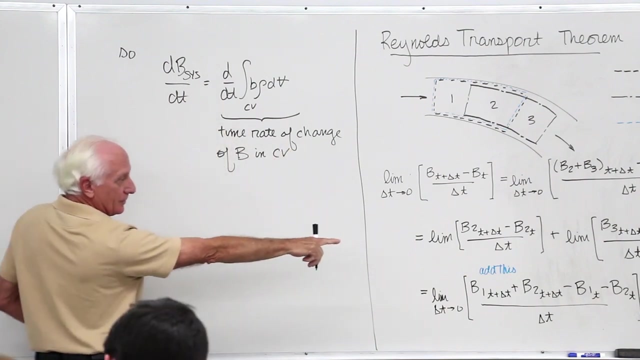 t goes to zero, we get the derivative d, dt. So this, then, is the time rate of change of b in the control volume. So time rate of change of b in the control volume. Now there's another term, that term over. 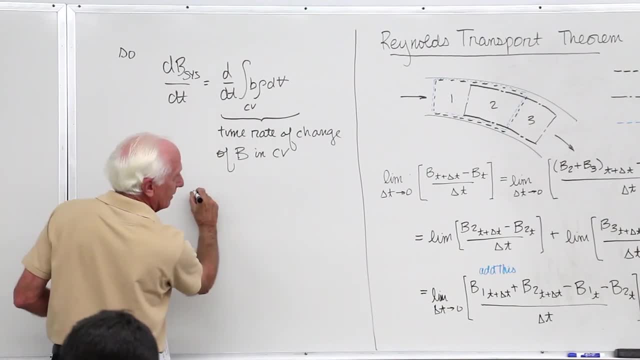 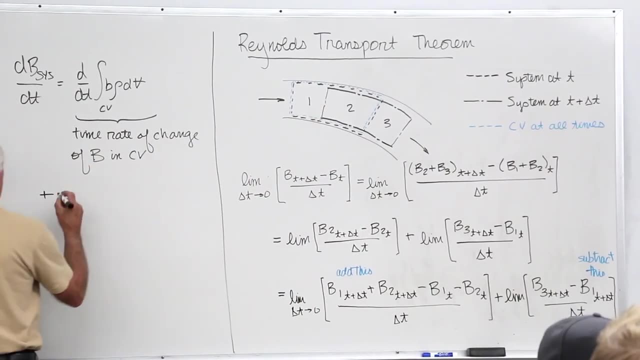 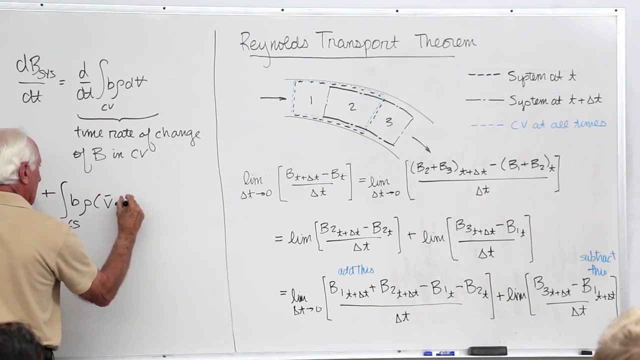 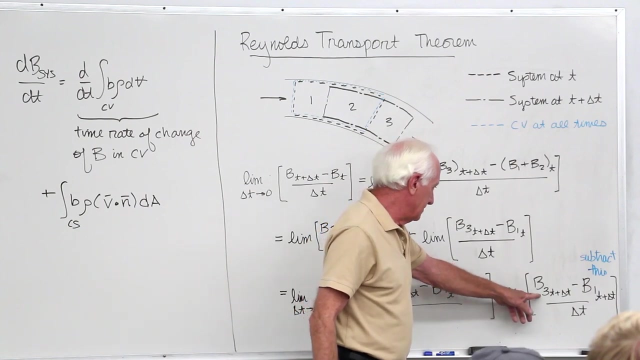 there. So we'll put that one down here, Plus this term right here, and that term here is integral- over the control surface: b, rho v, vector v, dot n, dA. Let's see what this term here is. Okay, this is the amount of b in region 3 at time, t plus dt. That's right. 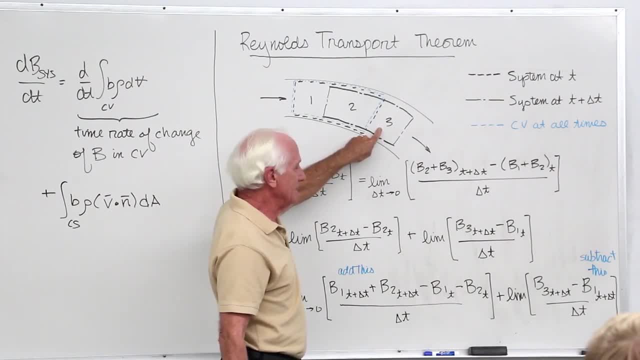 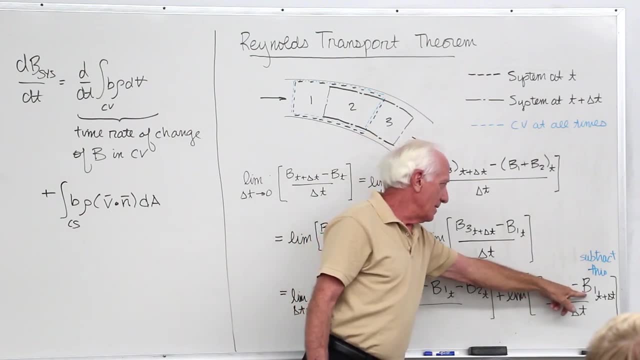 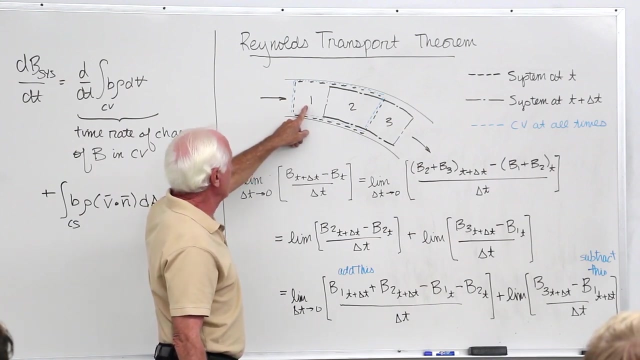 here. Look at my control volume. That's the amount of b that came out of the control volume. Okay, take this term here: The amount of b in region 1.. Okay, that's right here in the control volume. Where did that come from Here? What's in here? control volume? 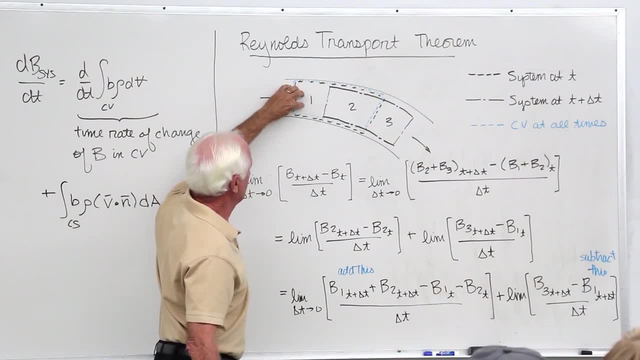 came from here. It's going this way, So this is the amount that came in. This is the amount that went out. That's called the net outflow, Out minus n the net outflow, And we've talked about this before. This is the amount that came in. This is the amount that 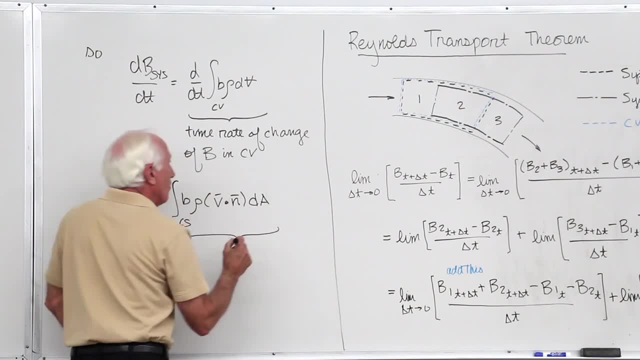 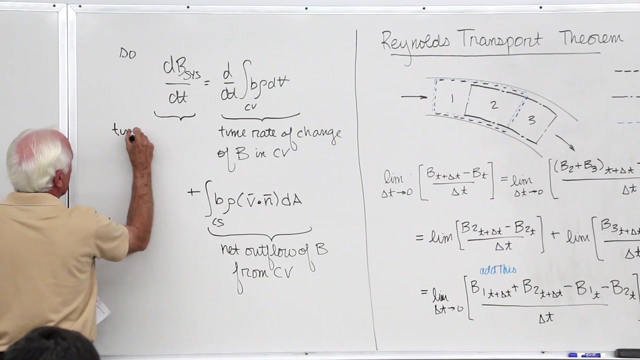 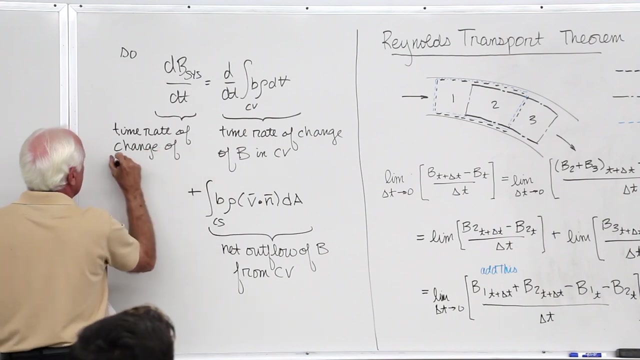 represents the net outflow. This is the net outflow of b from the control volume Or through the control surface. take your choice. Okay, left-hand side equation is the time rate of change. Right-hand side equation is the time of b in the system. So I'll just say it again This: 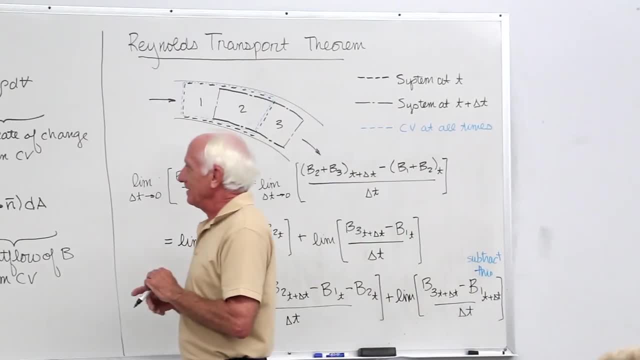 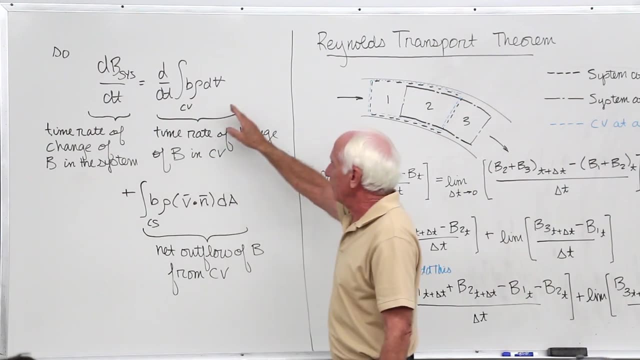 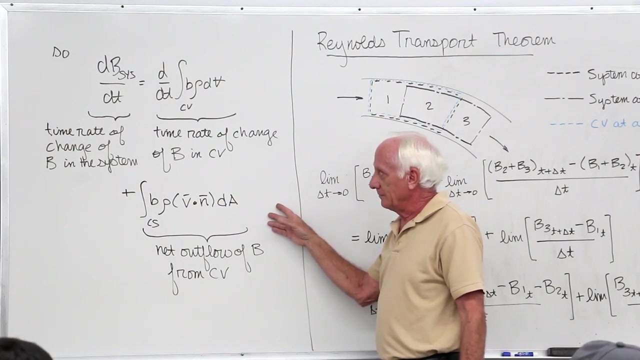 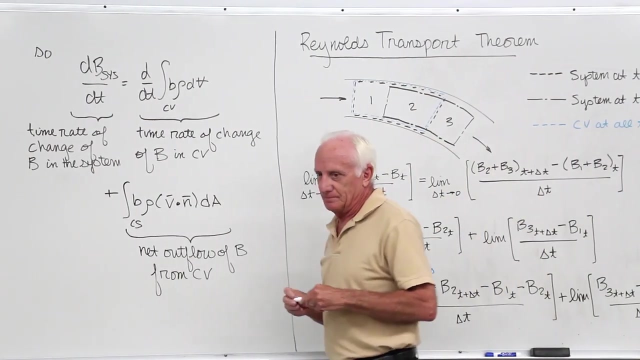 is the missing link equation that allows us to write the basic laws of physics and engineering, which are written for a system in terms of a control volume and control surface, which we generally like to use in engineering. Okay, And we did that last time. We let capital B be the mass. Let me just check and see where we left off. 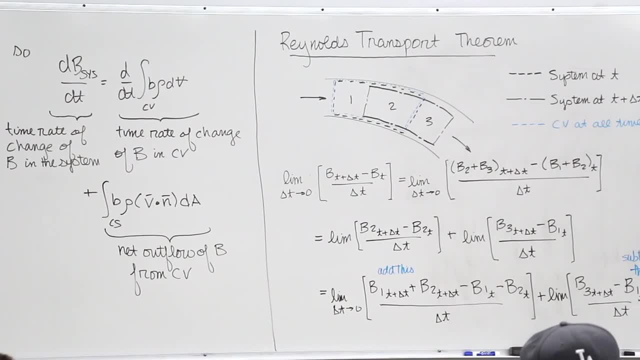 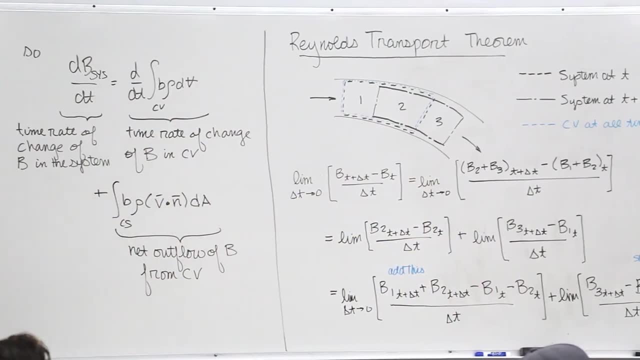 I'll tend to see if I left off at that particular point. Yep, there it is, Got it. We got all that. Yeah, we put last time. we put that in there and got the. we let capital B be the mass, Just to remind you. 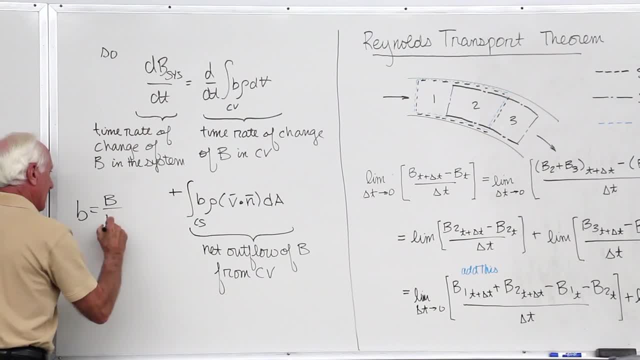 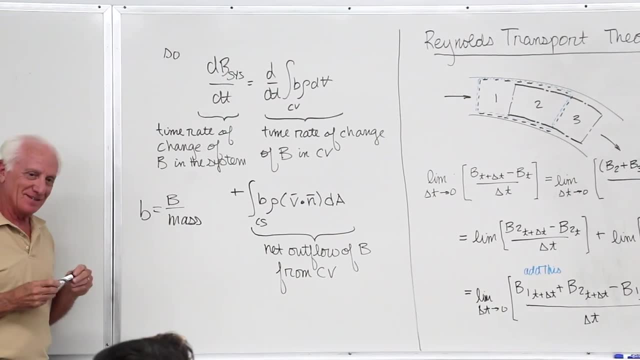 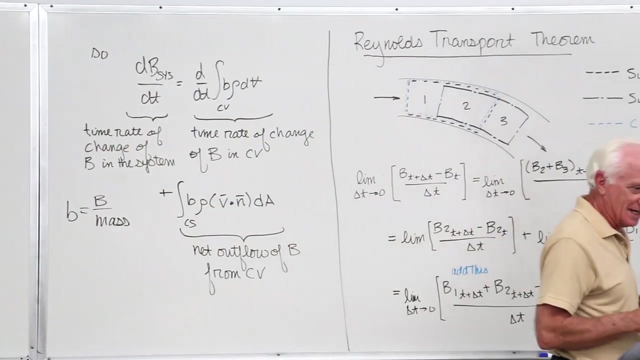 little b is capital B over the mass. If you let capital B be the mass, then little b is the mass divided by mass or 1.. So little b is 1. when we derived the continuity equation last time, And I'll mention what we did, Well, let's just go ahead and mention what we did last time. 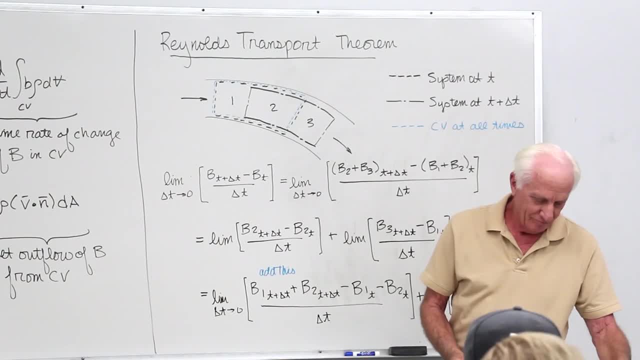 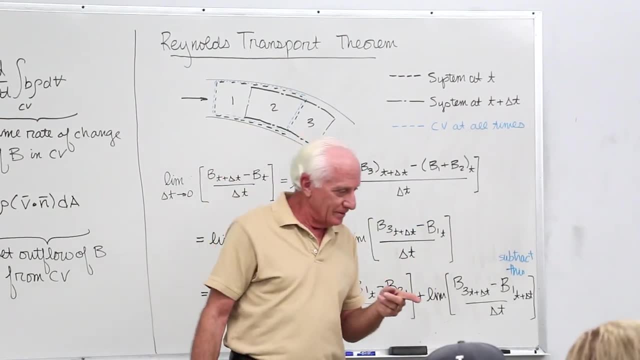 based on that. No, I'm going to wait and come back to it. Okay, Homer's going around now and I think that's the one with the problem of Problem 3-6. to start with right First, problem 3-6?. 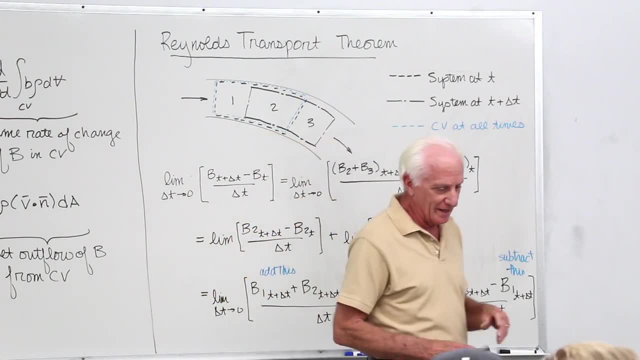 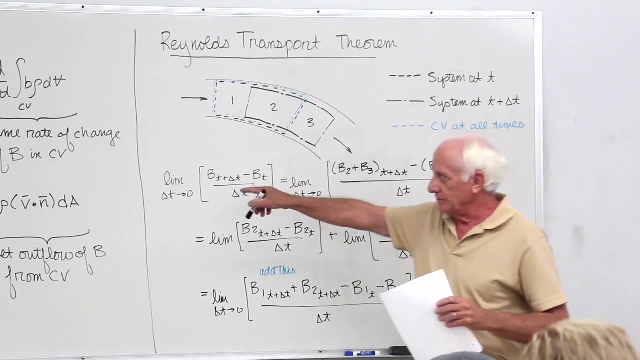 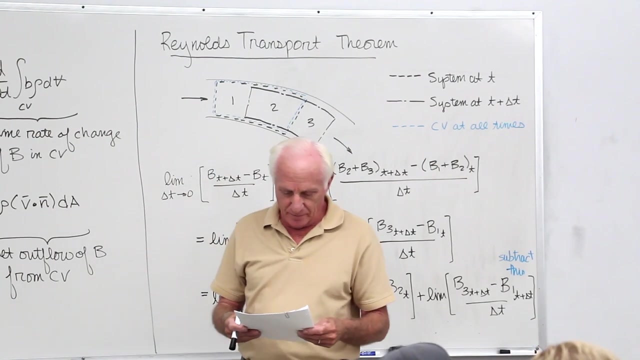 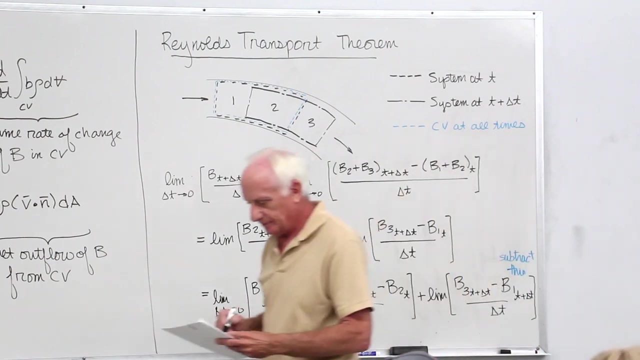 Yeah, okay, We're going to go over a couple of problems that Homer said that I have questions on after class and office hour, So we'll come back to this. We'll save this right now. come back to that, So I'll put this over here. Let's take a look at problem 3-6.. 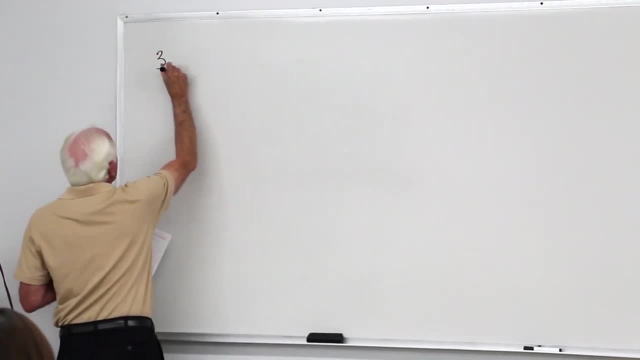 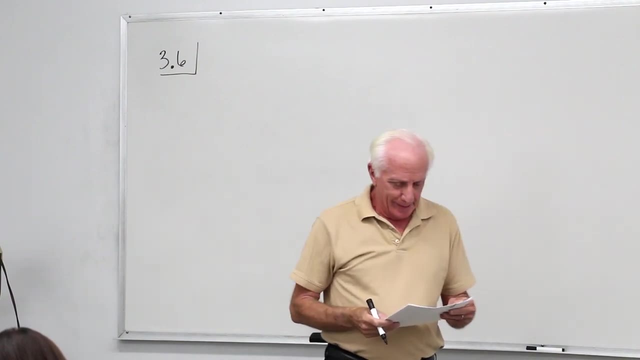 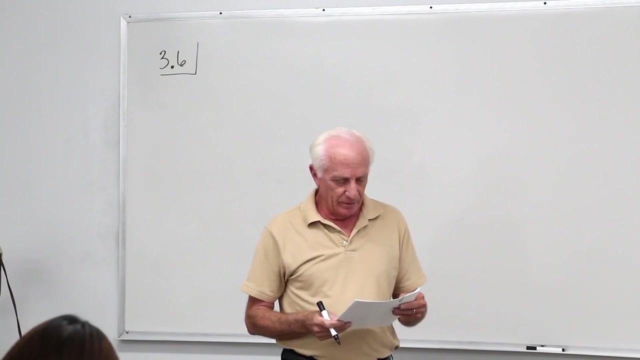 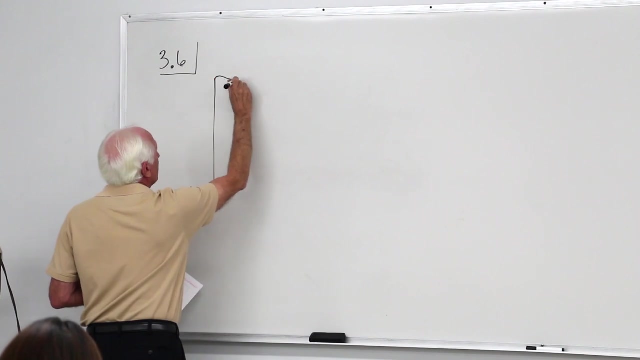 Okay, Let me read problem 3-6.. We're looking at flow along a streamline. We're trying to accelerate water upward in a vertical pipe. We're trying to accelerate water upward in a vertical pipe. Okay, We want to accelerate it at the rate of 30 feet per second squared. 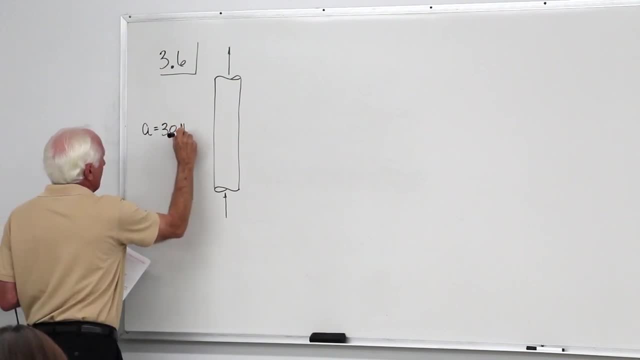 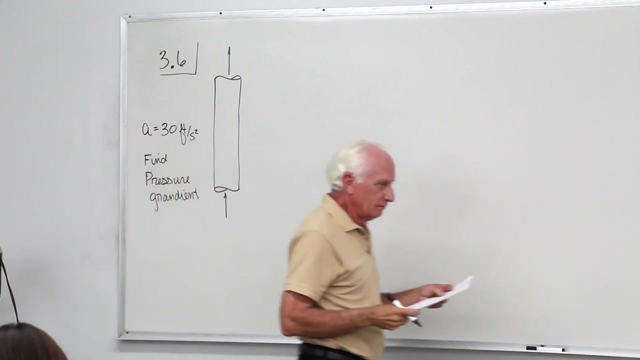 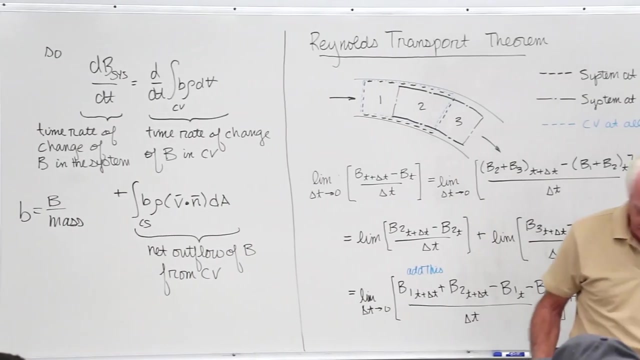 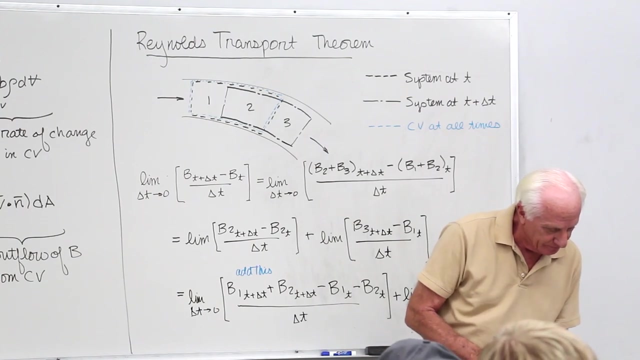 Okay, What pressure gradient is required? Okay, What pressure gradient is required? Okay, Let's see Equation 314.. Keep this here. Equation 314.. Equation 314.. Let's see. Oh, there, it is right. there, It didn't fail. Let's see. 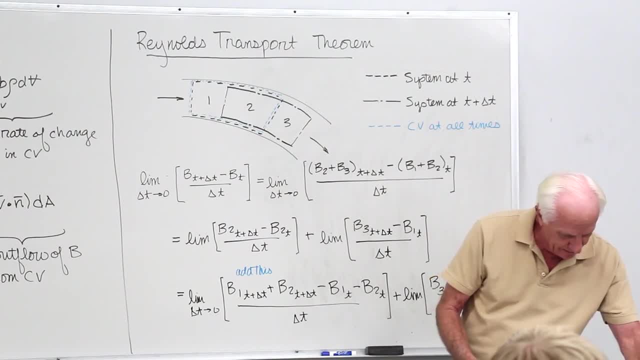 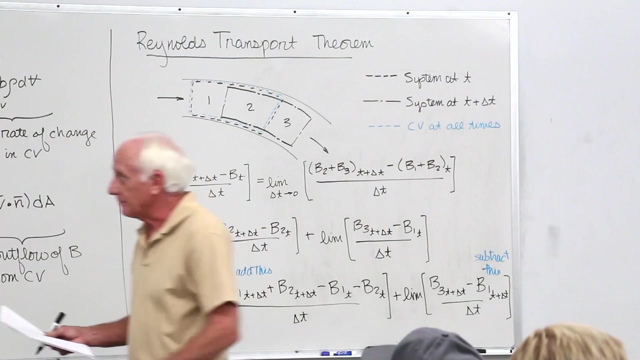 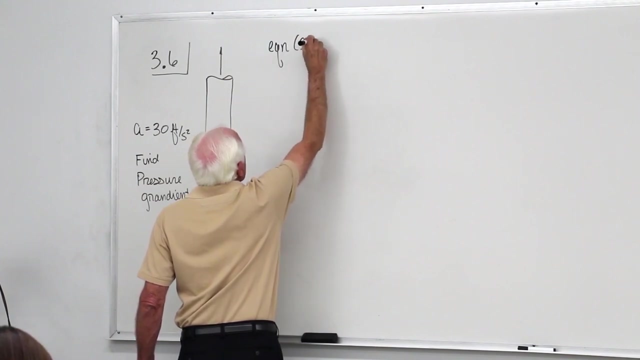 Equation 316.. Acceleration in the 1 and 1.. Go backwards. Equation 316.. There it is 314, not 314.. 314.. Equation 314.. This is applying F equal MA along a streamline. Okay. 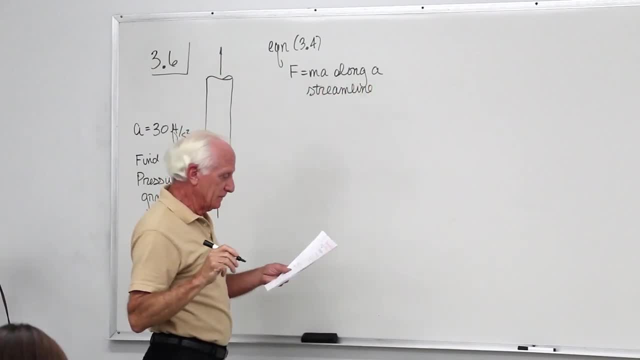 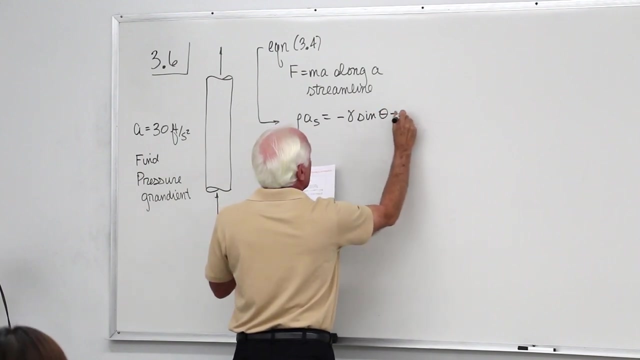 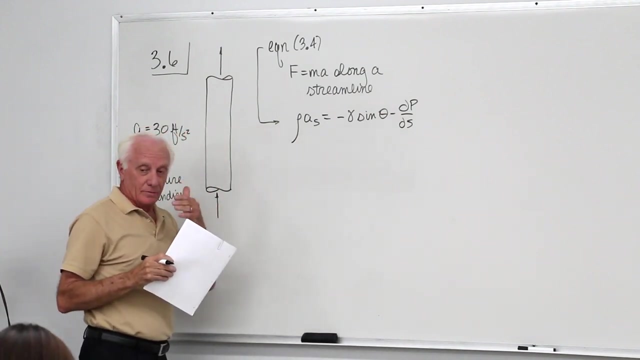 We went through it in class a few class meetings ago. You end up with rho a sub s. This is equation 314.. Rho a sub s equal minus gamma, sine theta, minus dp ds. What's their history of the terms? This one looks like gamma. 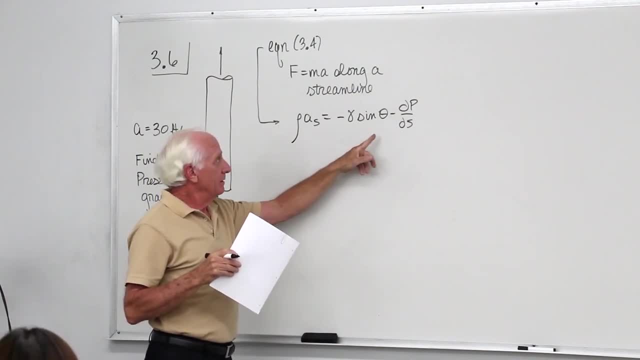 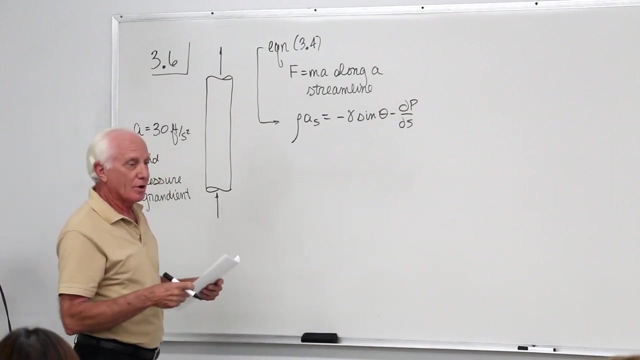 It looks like the weight. Yeah right, It comes from the weight. This one, of course, comes from the pressure change. This is the acceleration. Okay, The problem said water. I know it, I know it. He gave me AES 30.. 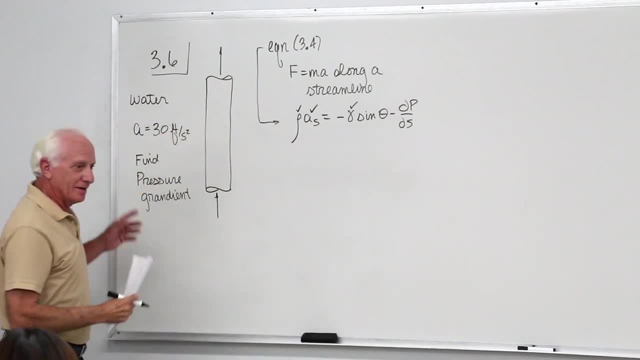 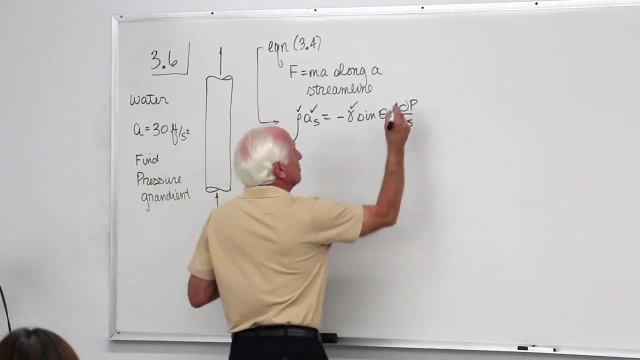 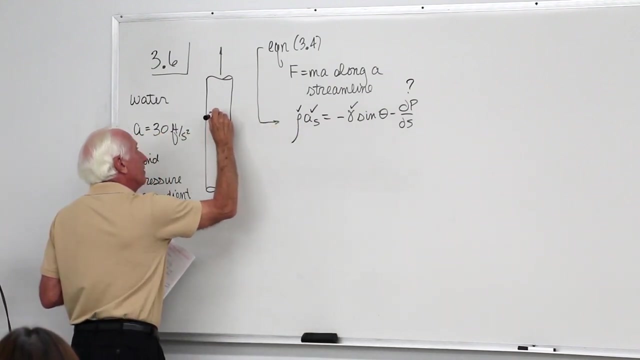 I know it. He asked me to find the pressure gradient. Pressure gradient is how pressure changes in a direction. Okay, There it is. That's what we're supposed to find. Okay, The flow is up. This is flow up, Yeah. 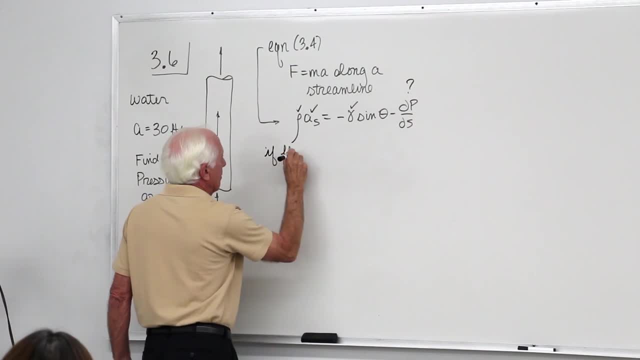 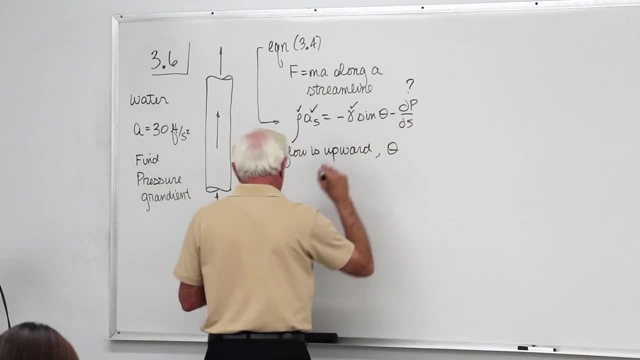 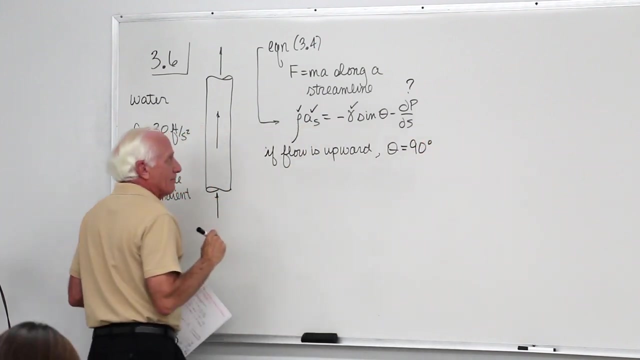 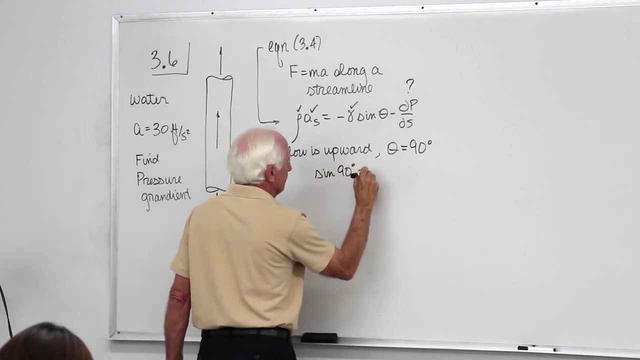 Okay, My theta for the flow up is 90 degrees Sine, 90 plus 1.. And so I get dp ds. Okay, Okay, So I'm on the other side of this. This is equal to this is the guy right here. 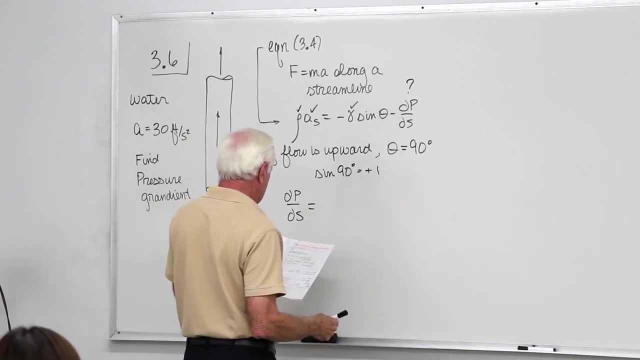 Put him over there And bring the other one on the other side. That's the mighty dp ds. This guy here is not written correctly. Let's get this guy right. It's gamma. And then this: this should be a plus sign here. 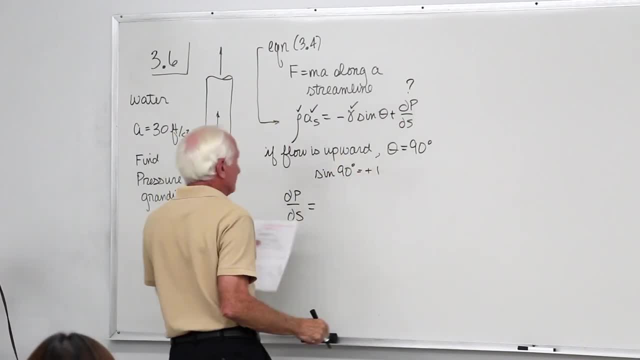 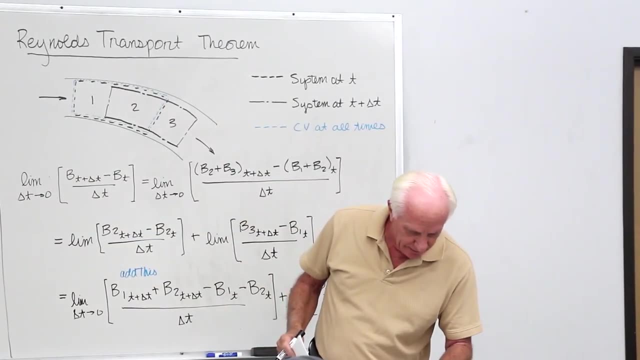 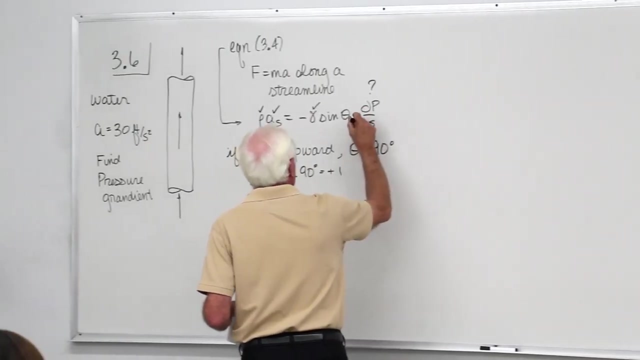 Pardon me. Okay, that's a plus sign. Let's verify and make sure that's right. Let's see: Yeah, that's a plus sign. Go back to the first one. Okay, I'm going to contrast that. Let's do these. 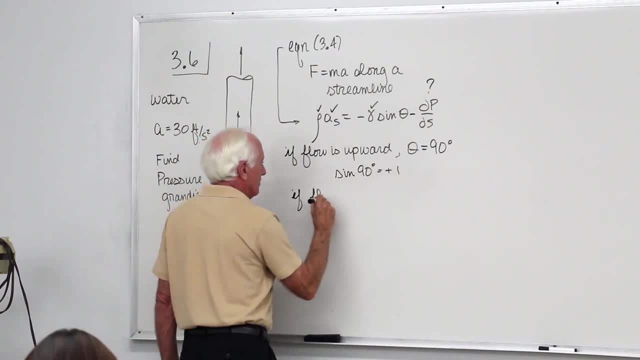 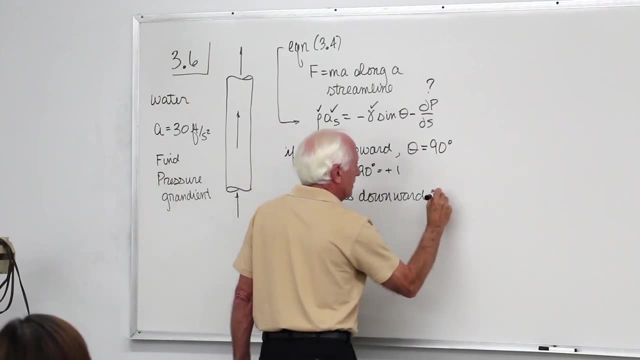 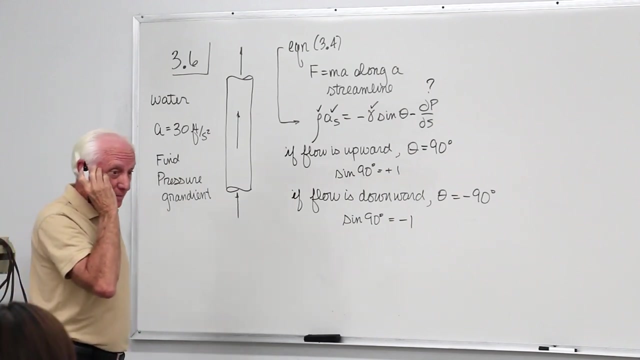 two contrasting ones. If flow is downward, there's two parts to the problem, Part A and part B: Theta equal minus 90 degrees. sine 90 degrees equal minus 1.. The question I had in office hour was what y is theta plus 91 case and minus 90 other case, If you look. 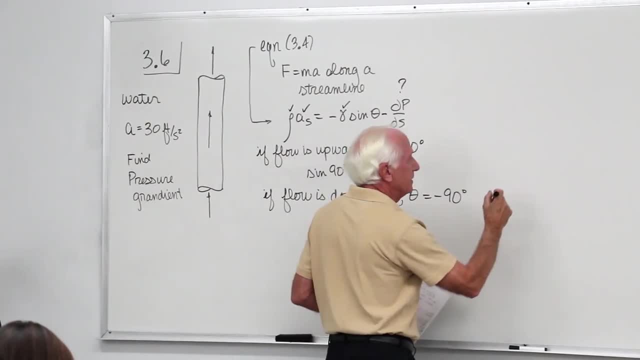 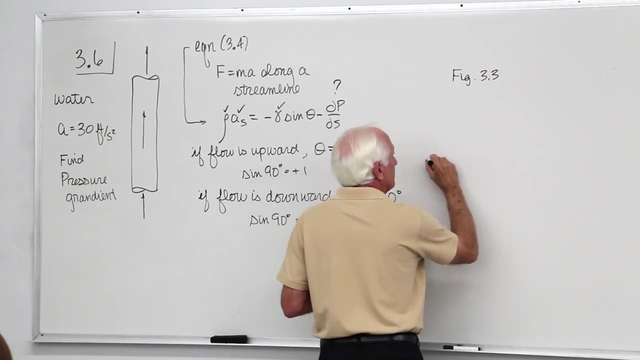 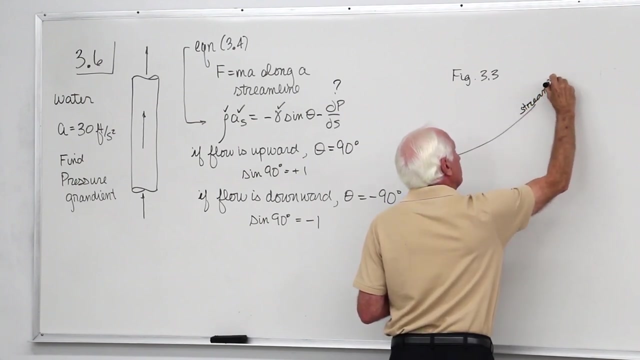 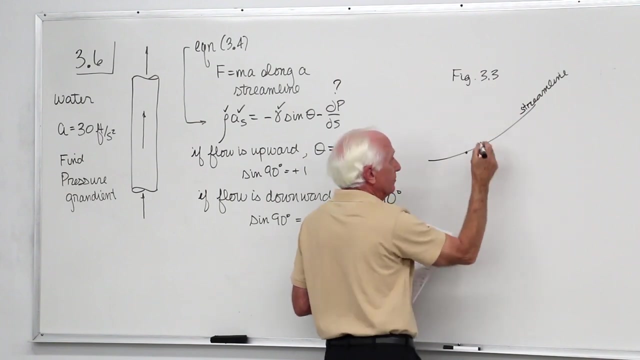 at the picture that goes with this derivation: figure 3, 3.. This is what it looks like. Here's a streamline. This is the S direction streamline. This way, The angle theta in figure 3, 3, that's where it's defined now- is there and there. 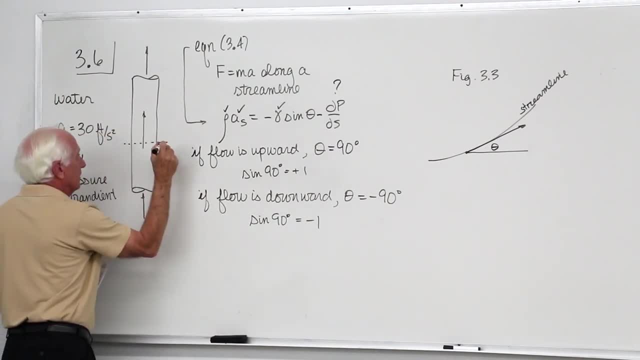 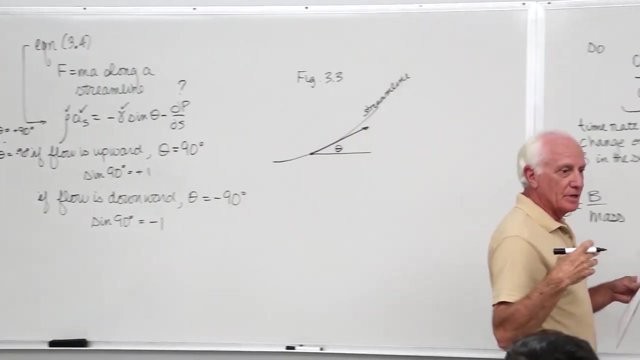 So look over here: If the flow is upward, theta is plus 90. If the flow is downward, theta is minus 90. So I just wanted to mention that fact of where that comes from, where you get the plus sign and the minus sign. Let's go back to that picture, the figure. 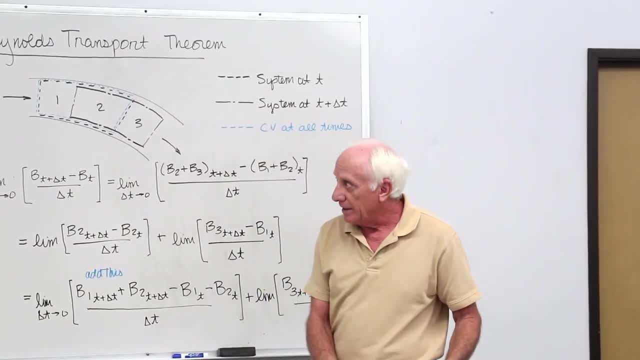 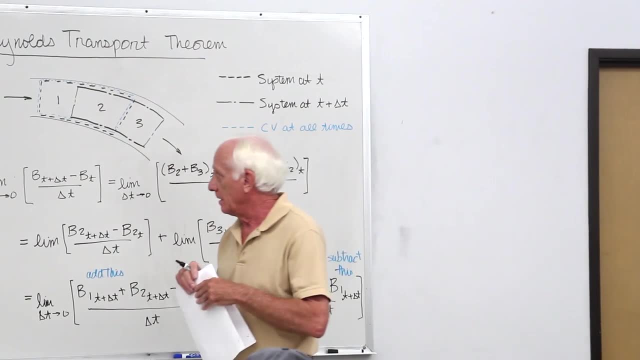 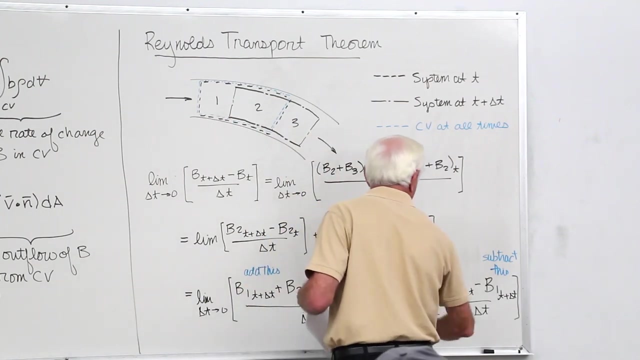 where it's derived from figure 3, 3.. And from there in the picture you can see what that angle theta is. One is positive and the other one is negative. Okay, now I'm going to save this middle panel, but I'm going to erase this one. 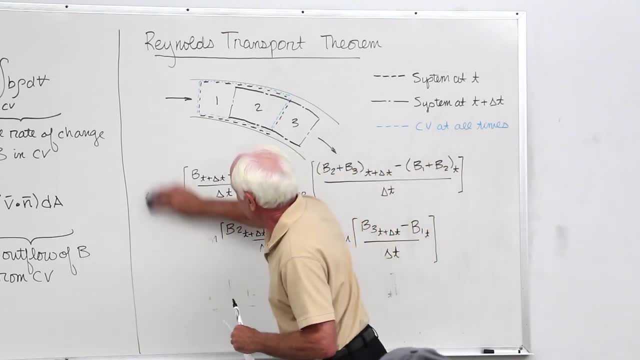 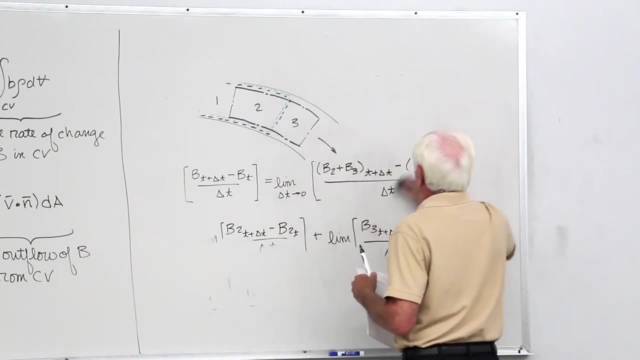 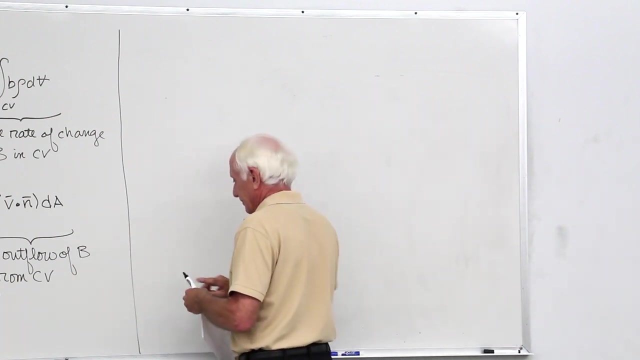 Any other questions on that one then? Okay, Now we'll do problem 312.. Okay, Water flows around two vertical, a vertical, two-dimensional bend. So water is flowing around a bend like this, And this is four-meter radius. 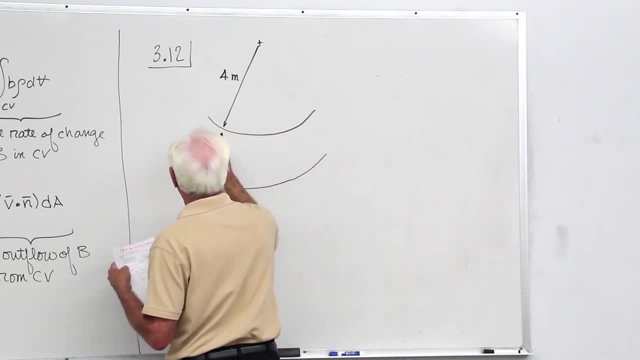 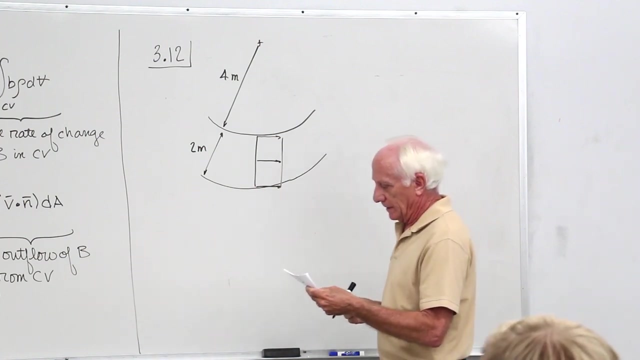 And this is two meters from here to here, And the velocity profile is uniform. like this, The velocity is 10 meters per second, And I guess that's it for right now. Okay, Yeah, Okay, let's read the problem. 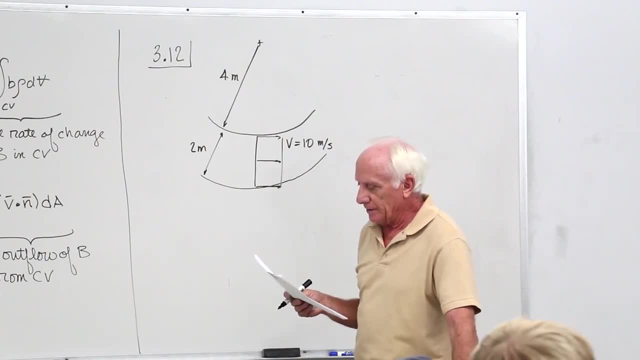 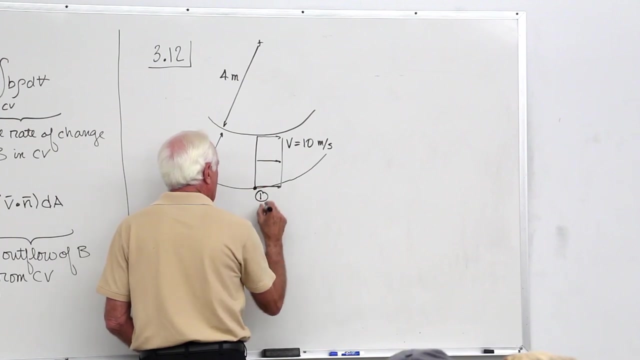 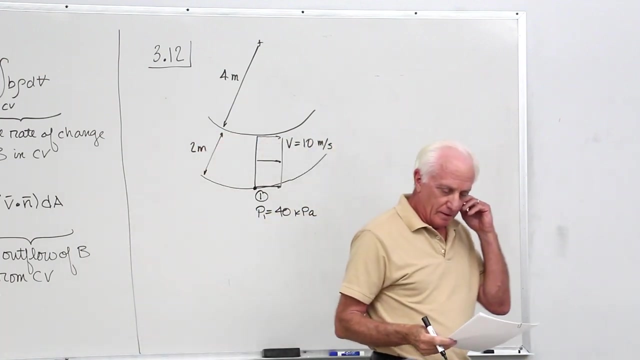 Water. it's water. Water flows around the vertical two-dimensional bend with a circular streamlines. Streamlines are circular And a constant velocity: uniform flow. If the pressure at point 1 is 40 kPa, It's point 1.. 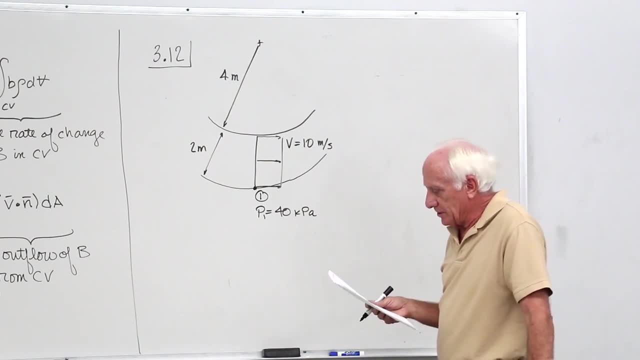 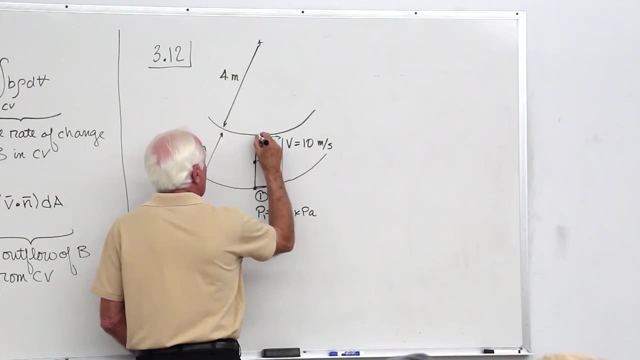 40 kPa Determine the pressures at points 2 and 3.. Point 2,: point 3.. The distance from here to here in the picture in the book shows that one meter. Okay, I don't think I'm going to need this derivation on this. 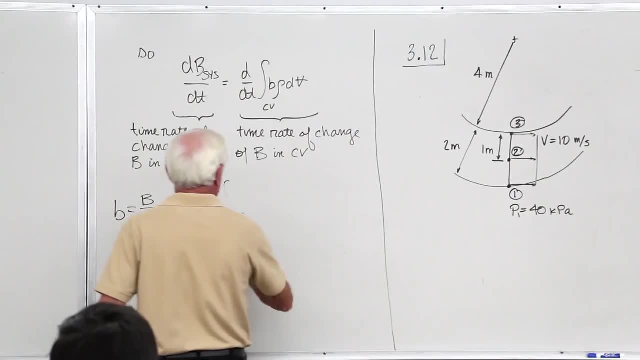 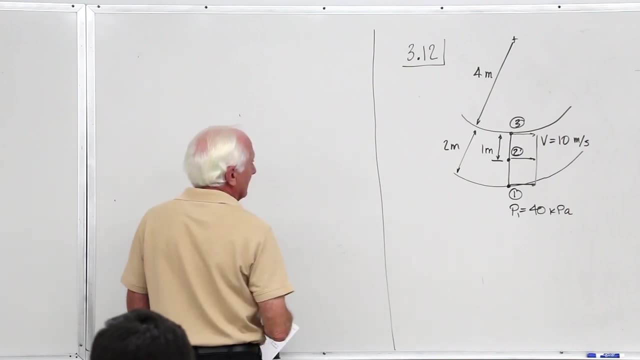 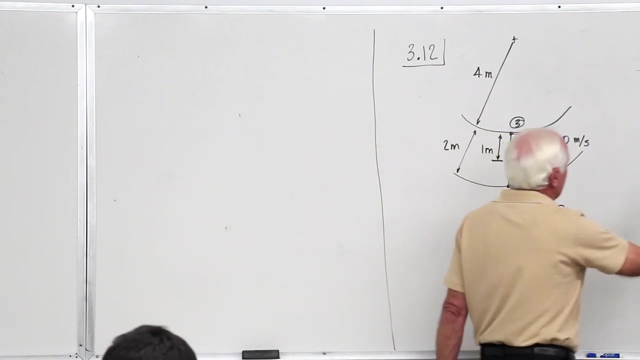 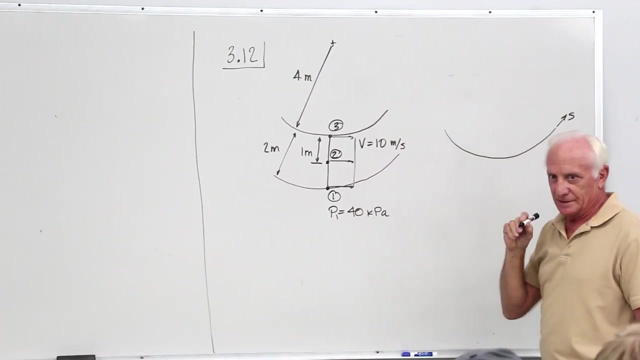 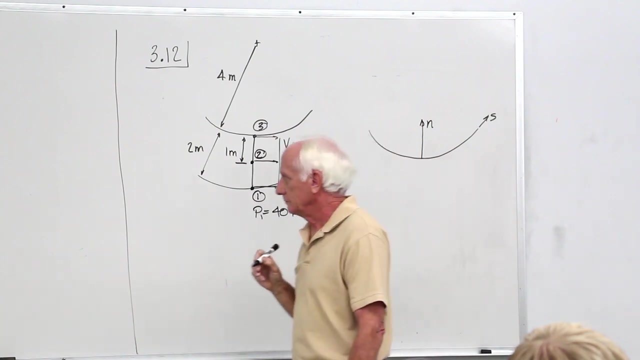 I'm going to erase this panel here. Okay, And that's. the can be divided into two, And there's a streamline And there's the s distance. Remember where the n distance is, The n is the normal, And this is: do we want to go along a streamline or do we want to go normal to a streamline? 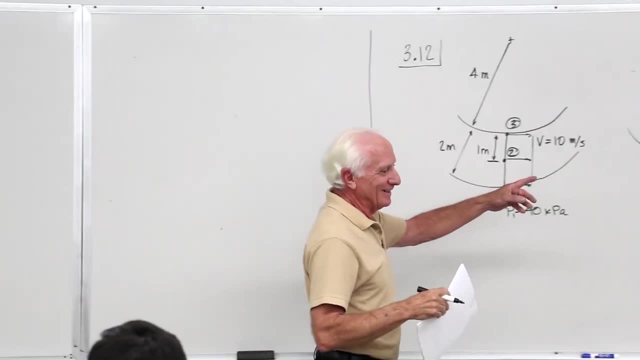 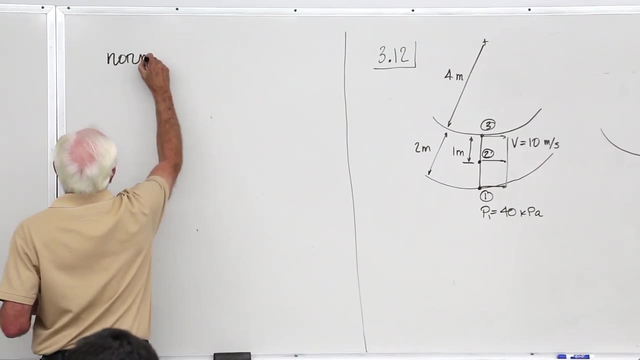 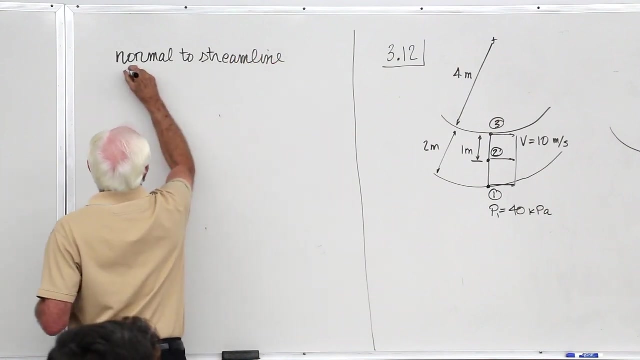 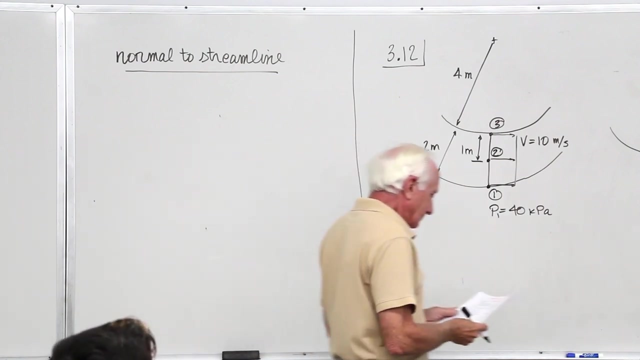 Okay, Obviously, we want to go normal to a streamline, Okay, So what is the distance now? So let's do this. We want to go along a streamline, So what's the distance? Okay, Let's see Normal to the strength of 1.. Let's find that equation. There it is. 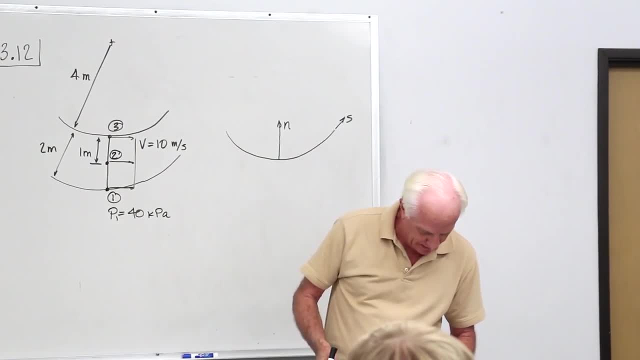 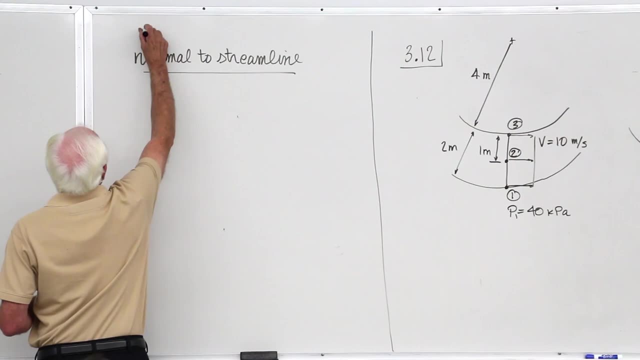 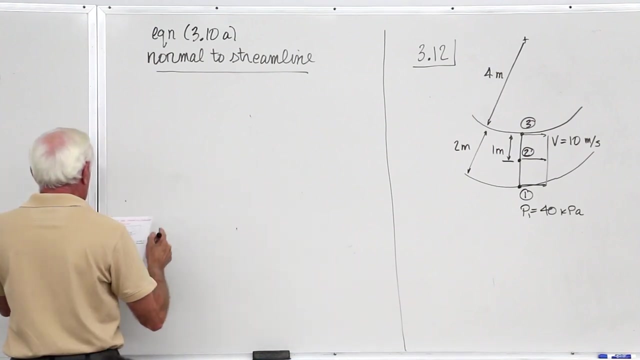 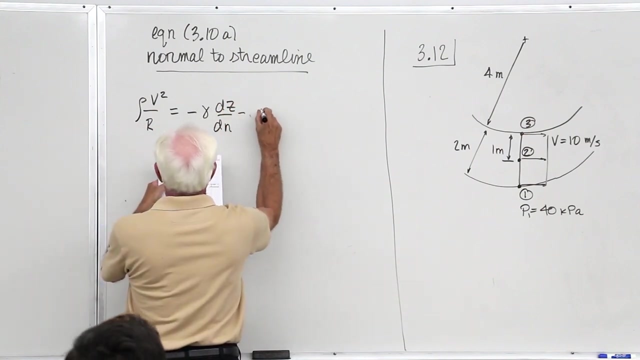 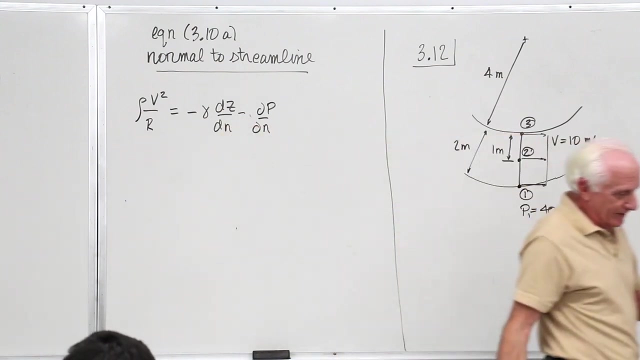 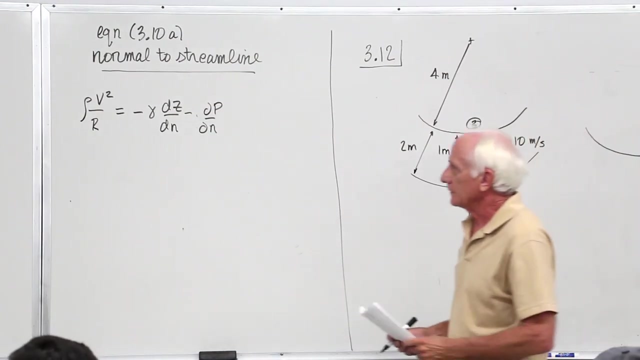 3.33.. Okay, I think it's yes down there at 3.10.. Yeah, 3.10.. Okay, let's write that one down then. Okay, Yeah, okay, Okay. here they are, Along the streamline, parallel to the streamline. 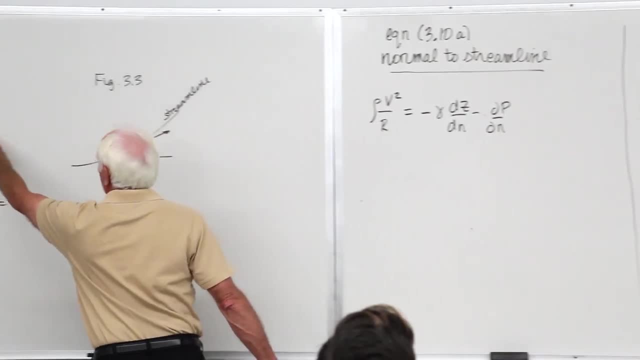 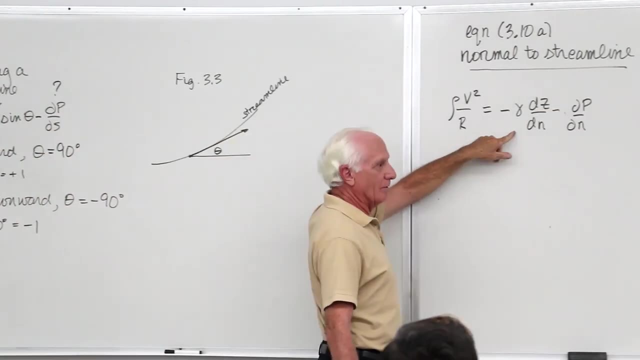 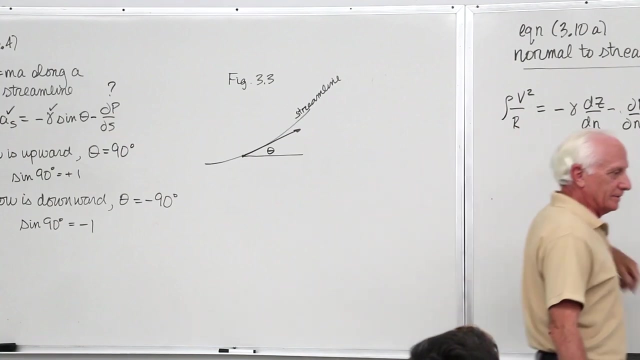 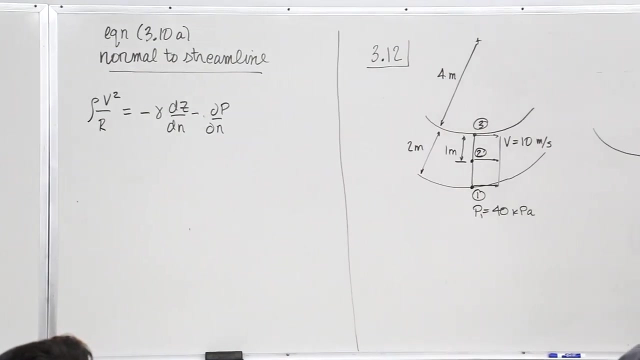 normal streamline and long streamline dp, ds, dp, dn And this is normal. this is the longest streamline. Okay, Looks like Gantt is in both, Gantt's in both, So I'm going to streamline This. is b squared over r, r, okay, r. if I'll look at the picture, Guess what r is at 0.1?. 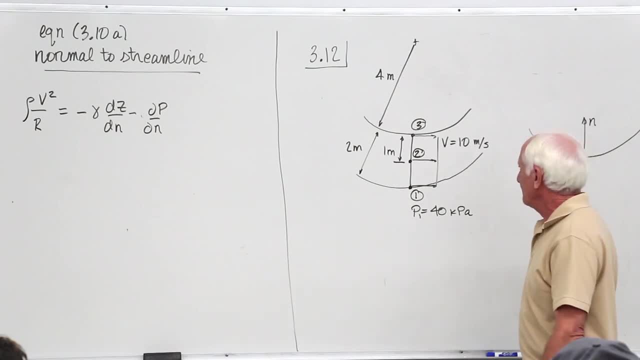 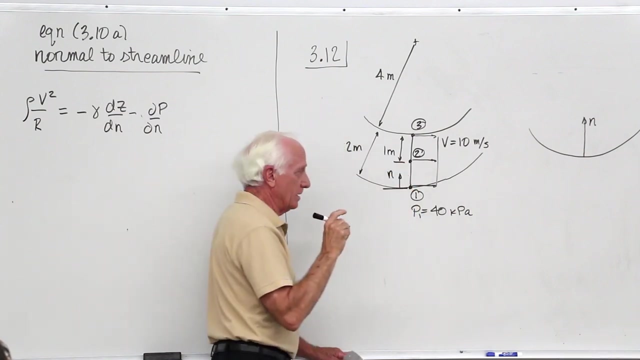 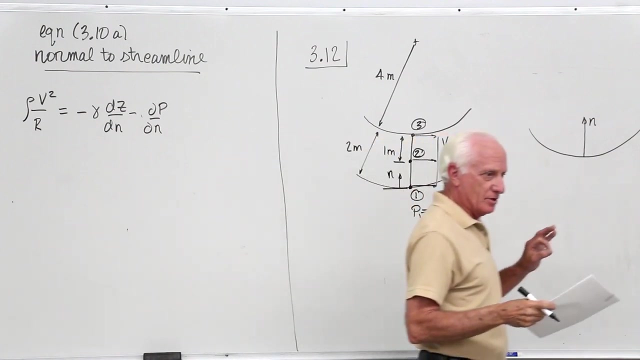 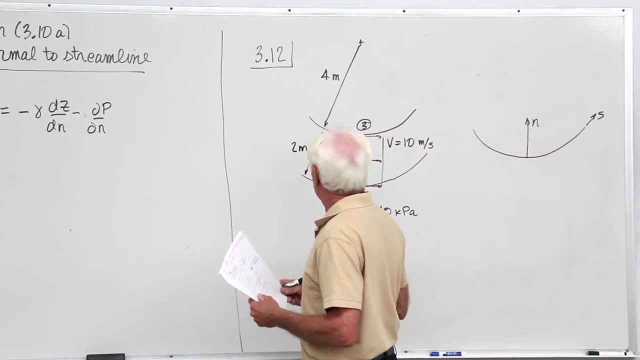 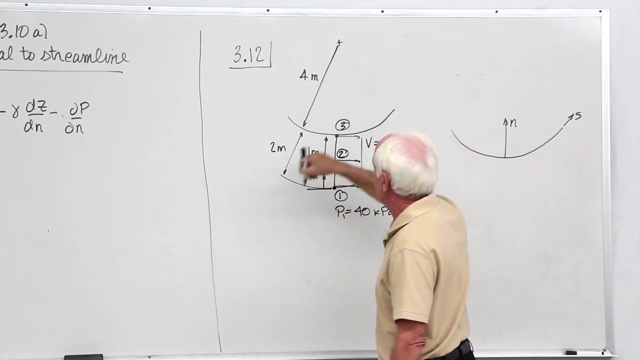 Okay, 4 plus 2, 6.. Okay, Guess what r is right here? 6 minus, by the way, is the B at 0.1.. And we said: if 0.1 is 0.1, it's probably going to be 10 to the power of 10.. 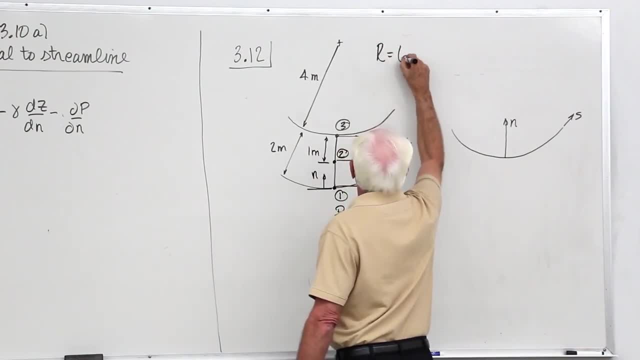 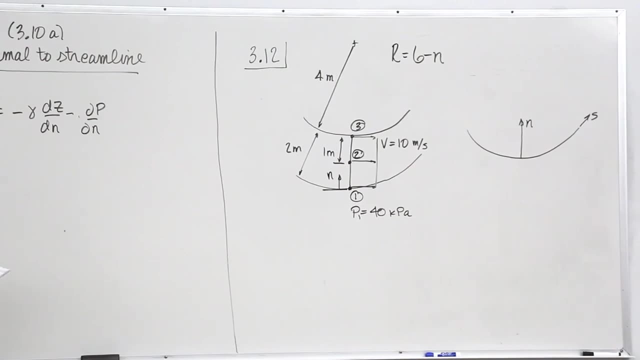 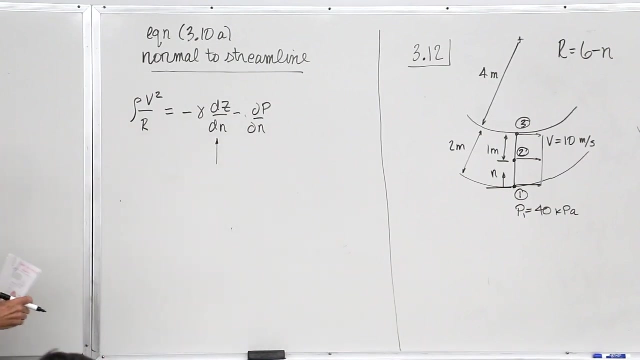 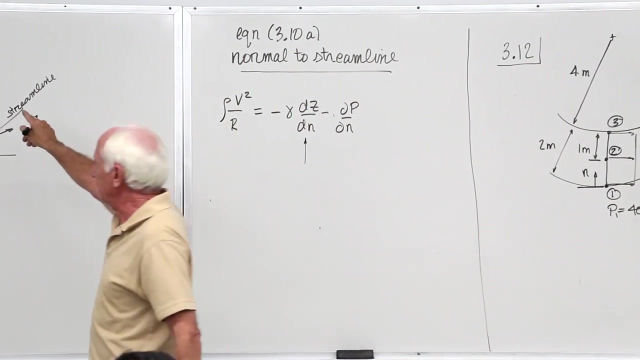 So number one R: okay, that goes in here. okay, so let's see what can we go. okay, question on this one is the question, this one is: what is this guy right here? okay, and here we go again back to figure three, three. always go back to figure three, three, go back to figure three. 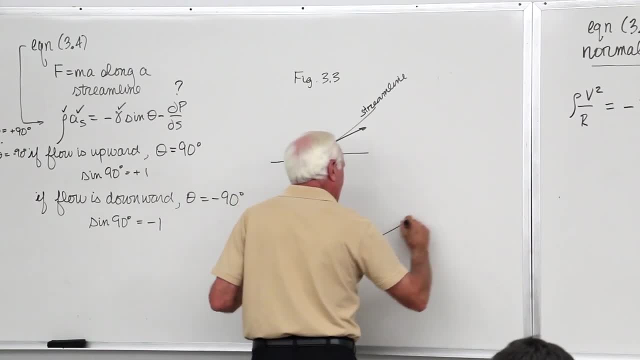 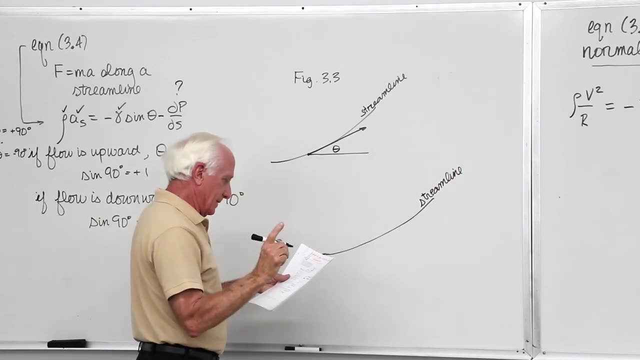 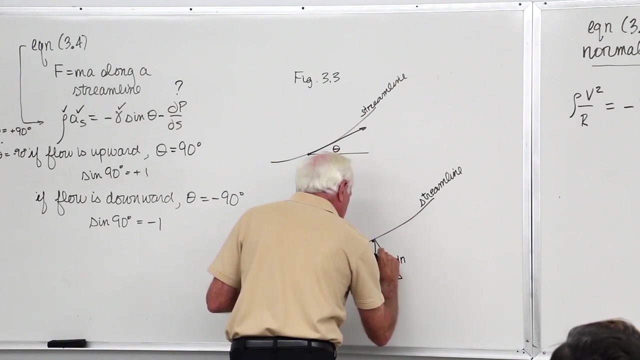 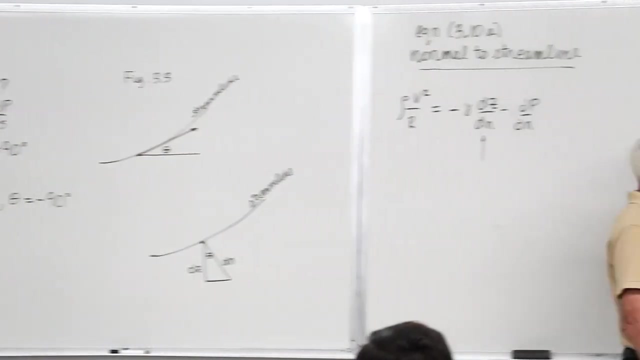 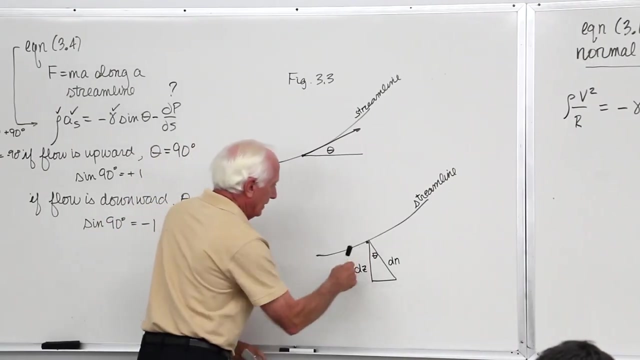 three. here's the stream one they show in that picture. this is easy. he calls them Delta. this is DM. this is the angle, theta. okay, the same as that theta. the same as that theta. this picture is in there, the sketch. okay, right here, at this point. right here, theta is zero. okay, I'll draw. 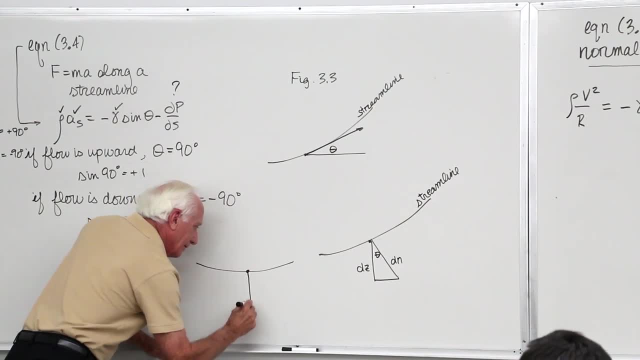 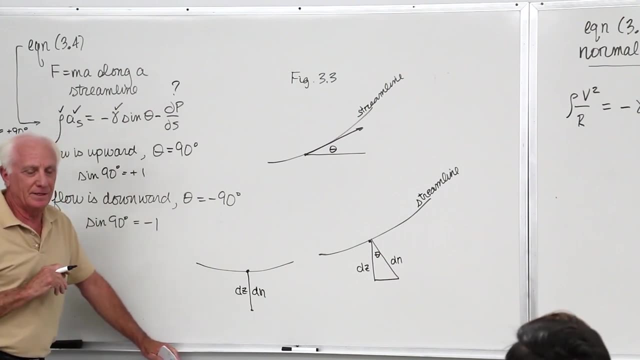 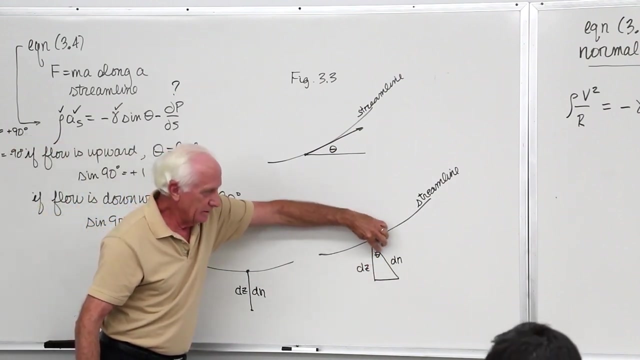 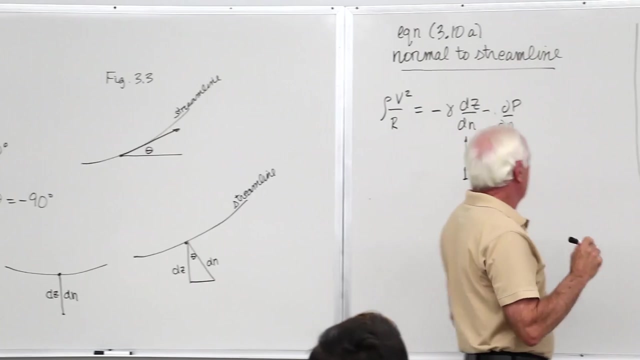 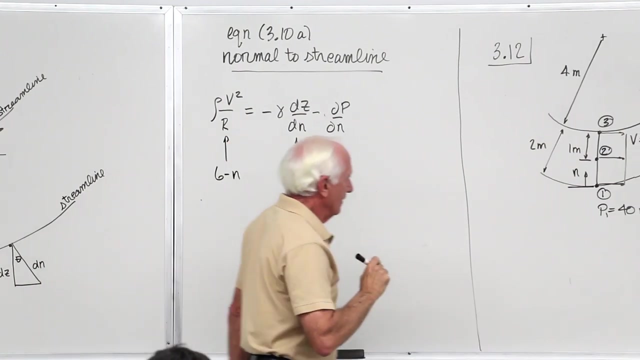 this at this point, right here. here's DZ, here's the end. guess what is easy? divided by DN is one, because when the same zero DZ people DM, so we go up here you replace that with one. over here, we put in six months and- and I'm not gonna do the rest- you go ahead. 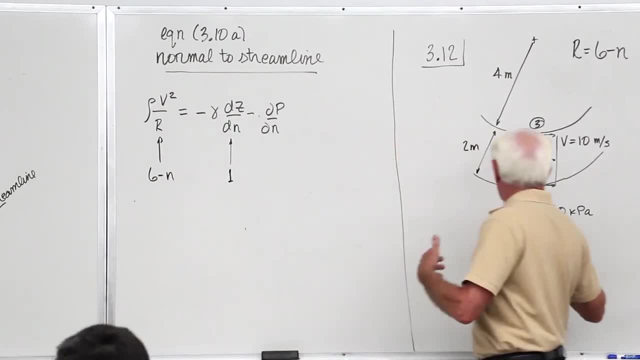 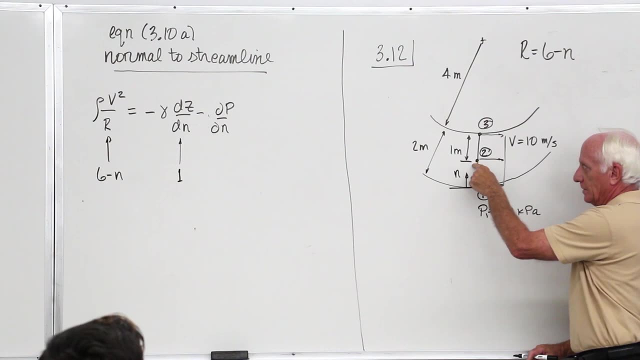 and you integrate from the bottom here to the point here. okay, from here all the whole Ц here to here. When you do that, you're going to solve for the pressure of 2.. Then you integrate from here 1 to 3. And that's going to give you P3.. But this is. 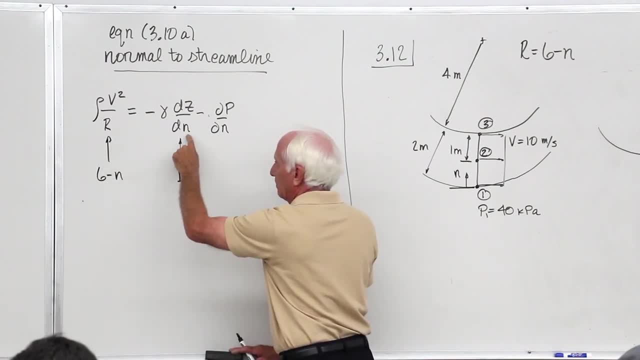 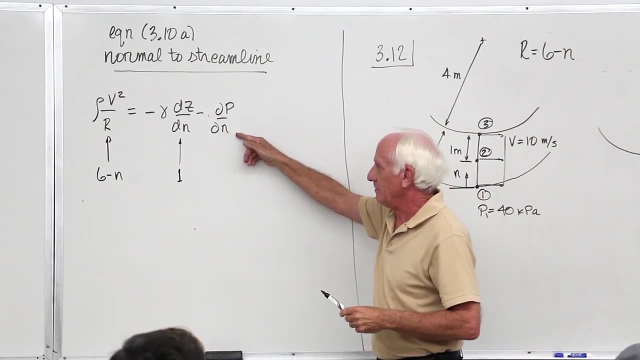 where people are getting hung up what to put in for R and what to put in for DZDN. What are you solving for? Well, you're going to integrate what you're looking for. how P varies with N, N is 0. down here, N is 1. right here, N is 2. 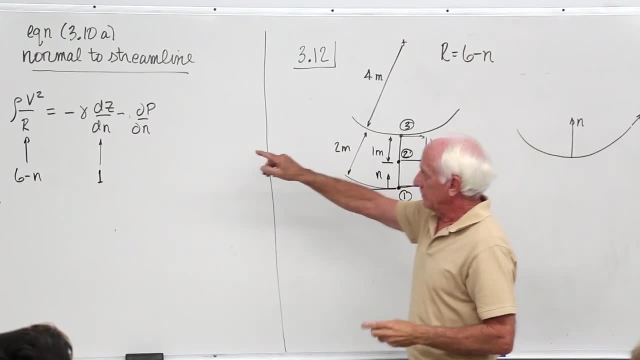 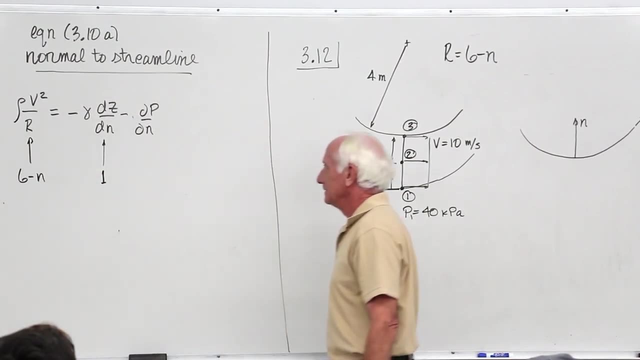 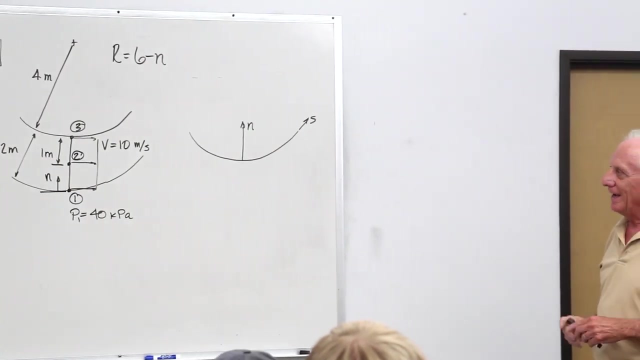 right here. So integrate with respect to that. You've got a 6 minus N downstairs here. It's going to be a natural log, but I'll let you play with that. We've already done it, so you know. Anyway, that's a couple other questions. 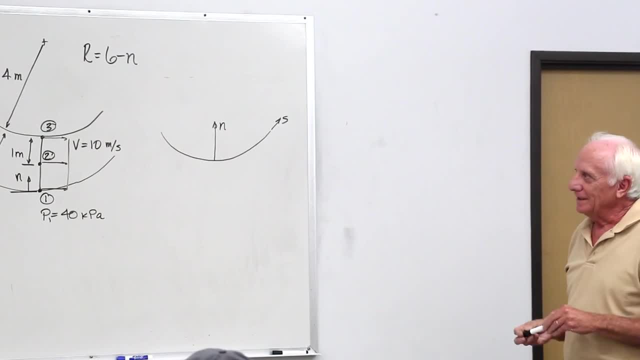 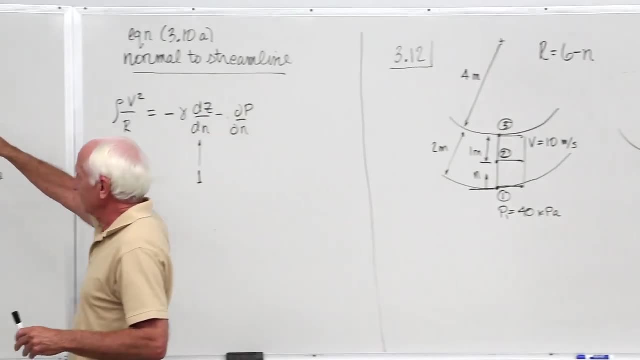 I had about those first two problems on that homework set. Yeah, it's not easy, I know, But mainly you know I was going to say for both problems you have to go back to figure 3-3.. And I assigned them because this one is a problem which is. 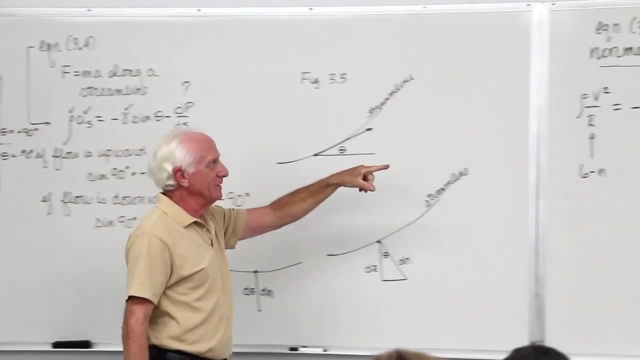 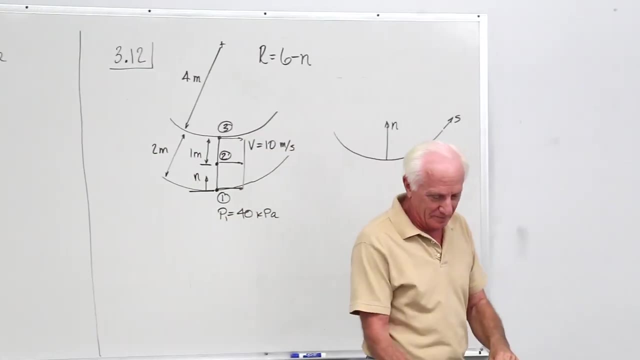 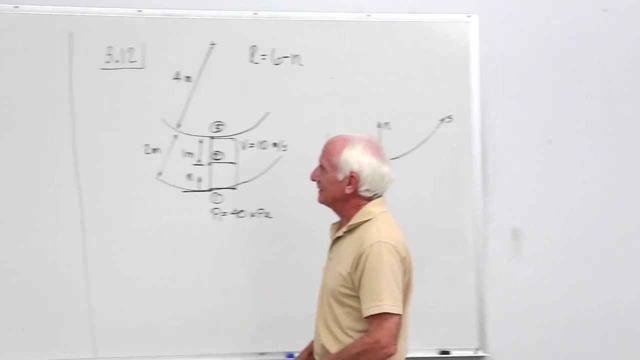 along a streamline with this equation- And this one is a problem- normal to a streamline, which is this expression right here. Okay, Now anything else on that. before you go on, Let's see, I need space, I need, let me erase this guy. I. 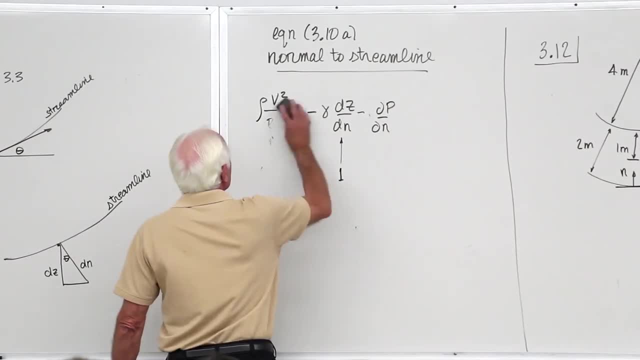 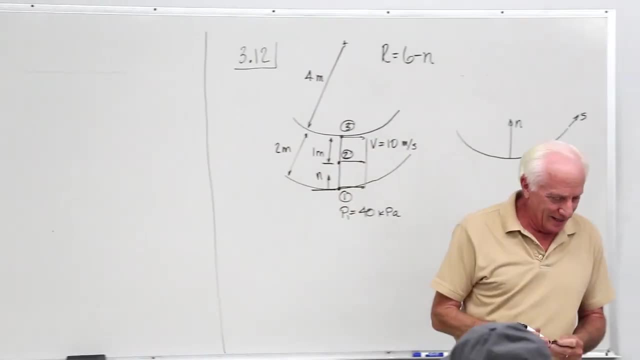 don't need him right now. Okay, All right, Nothing. Why don't you erase it, sir? Okay, I just want to go back and look at 3-48.. I didn't have any questions on it, But I want to go back and look at it. Somebody mentioned a couple of things. 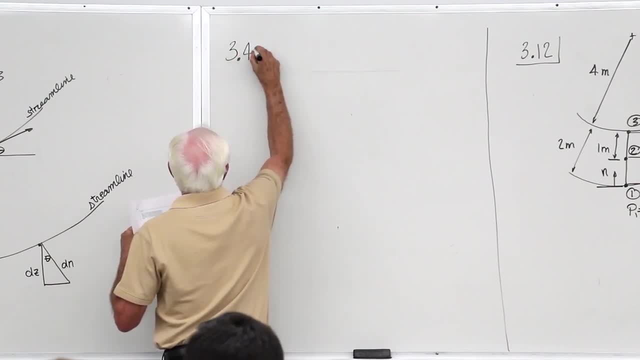 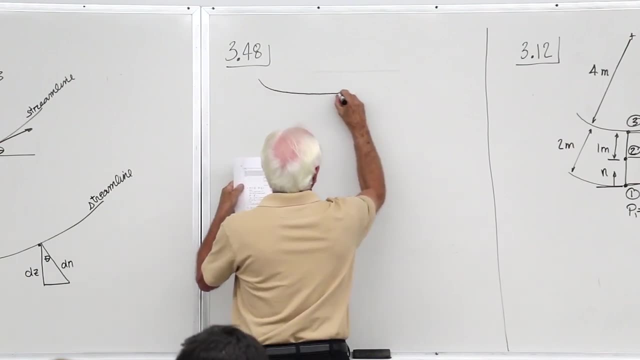 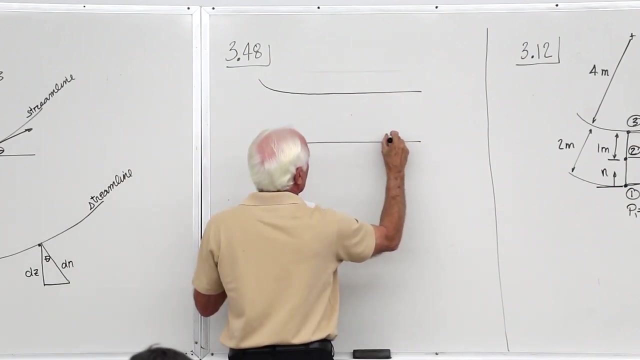 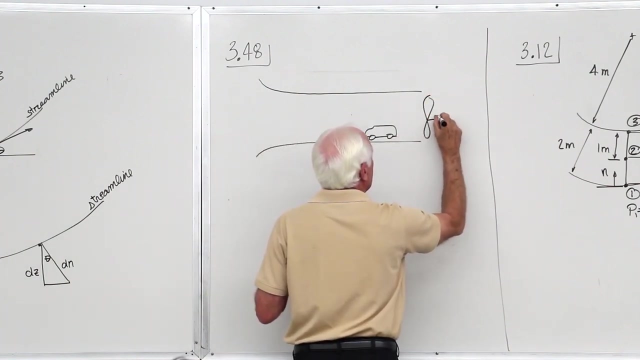 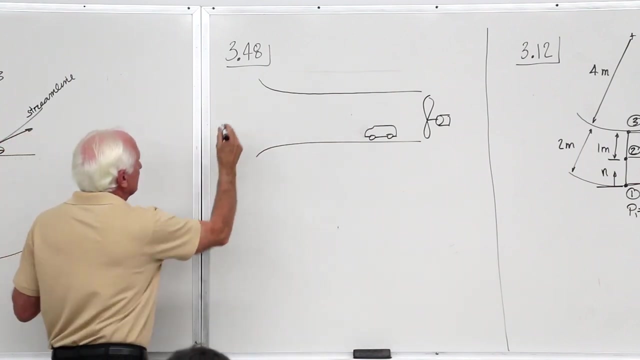 3-48.. This is a wind tunnel And in the wind tunnel we have air. We get bowl for it. Okay, an automobile. so we've got this little car and there's a fan here which pulls the air through the wind tunnel. the fan pulls the air through the window, so we 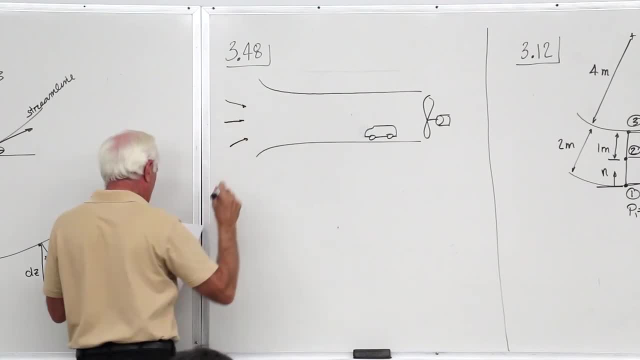 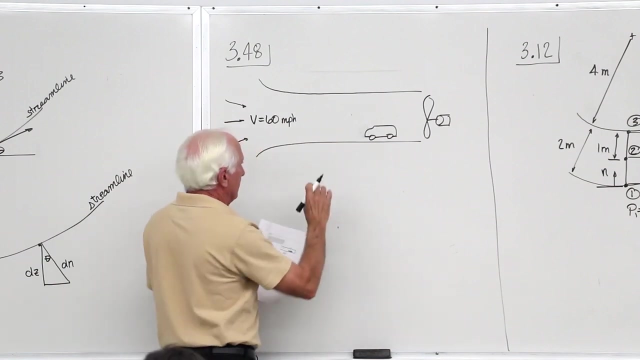 have the air coming in the wind tunnel like this. it's used for testing automobiles. okay, the speed is 60 miles an hour. okay, there is a YouTube manometer here and as he comes down, goes over and goes up, it's open to the atmosphere on the. 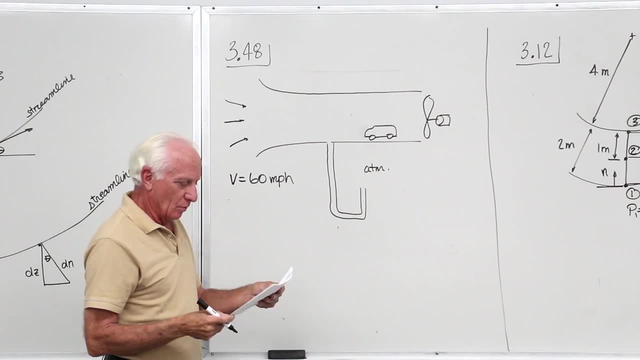 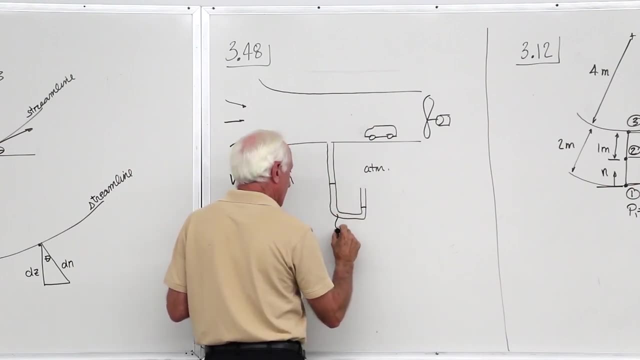 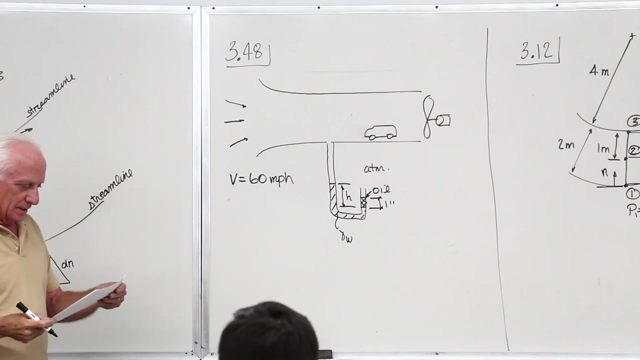 other end of YouTube. there's water in the YouTube. the water height in the water is H, the differential height H. and then he tells us that there's a one inch column of oil on top of the water in the manometer. so we have oil here. okay, that's oil. okay, let's see here part A: 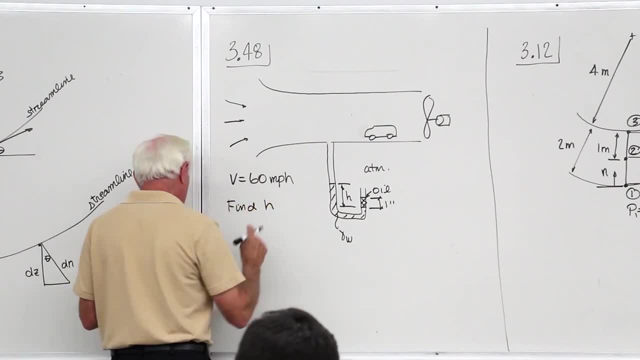 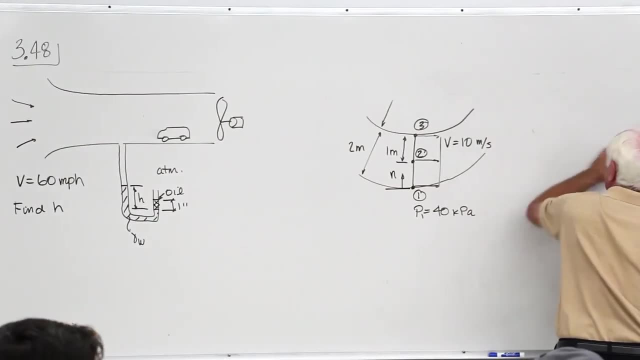 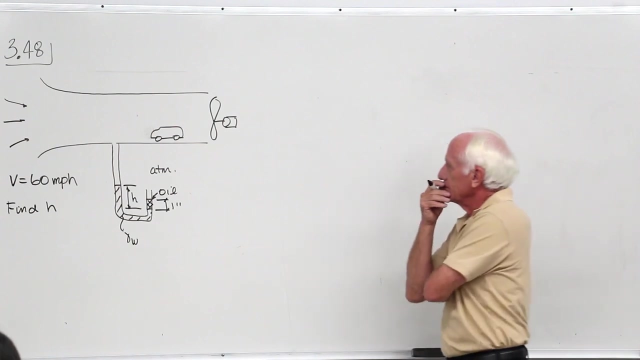 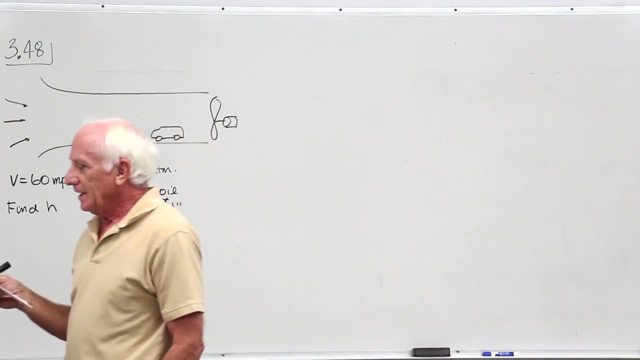 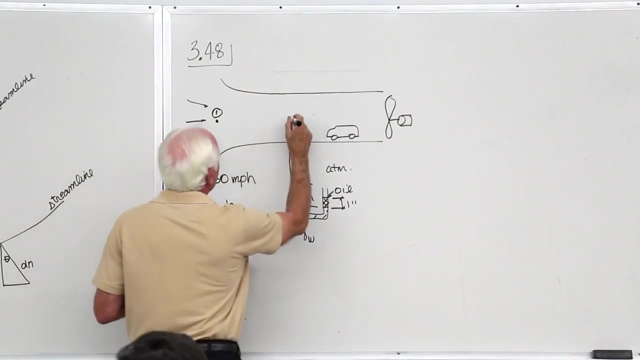 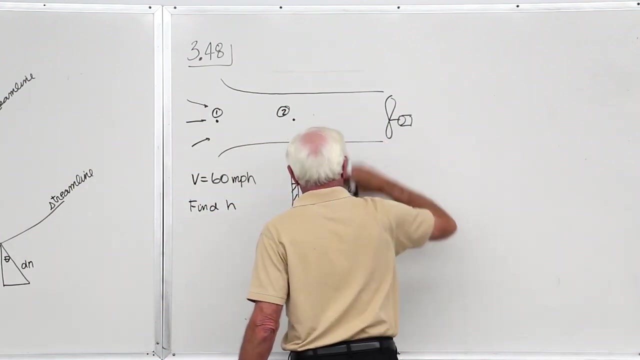 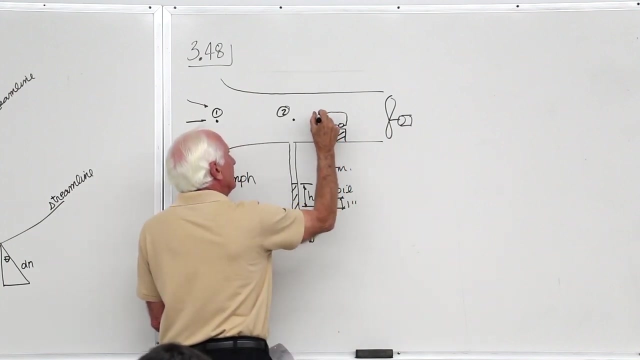 fine H. all right, he. he's nice to you. nobody's this nice on exams, but he's nice to you. he puts a point one out here, he puts a point two right here, you, and he puts the point three right there. rise up, whether grill on the man. 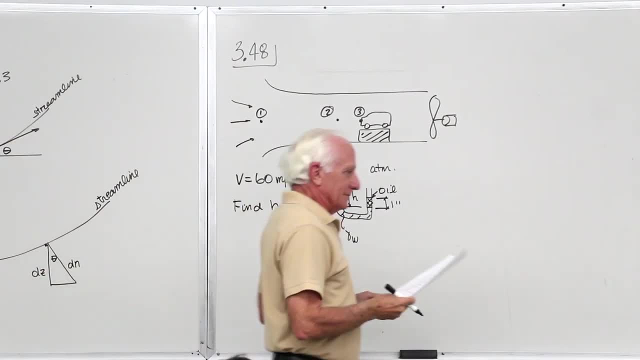 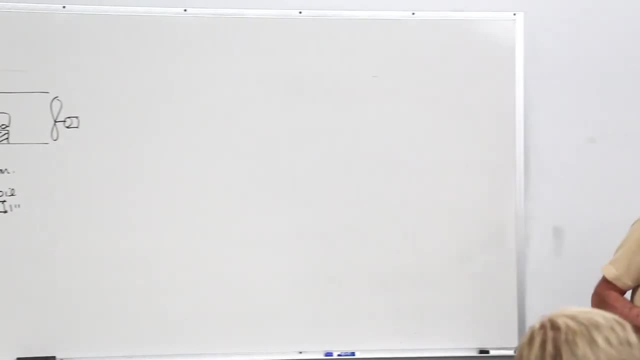 find H. okay, now this is in check for three, chapter three. it's use little logic. its using logic is probably gonna mean you're gonna use Bernoulli's gonna need to master conWorld a little logic work. I want to make sure you actually have an. 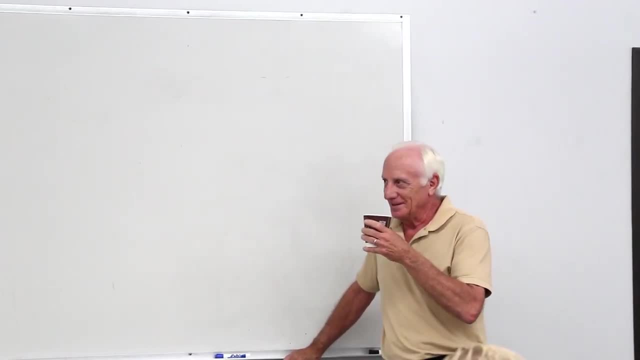 idea of how those logic work. but I just want to give you a part of a shout out. We're not going to use the equation, the streamline we had before normal, to streamline. No, this is the Bernoulli problem. So, with the Bernoulli problem, 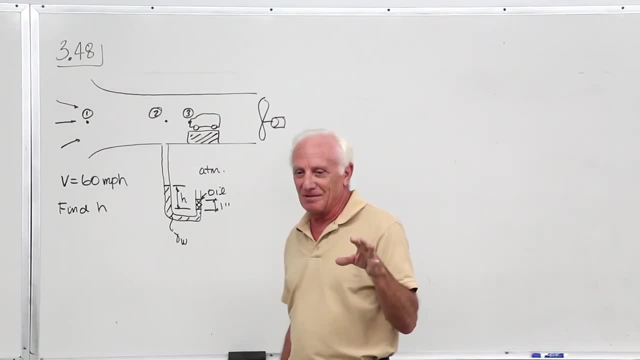 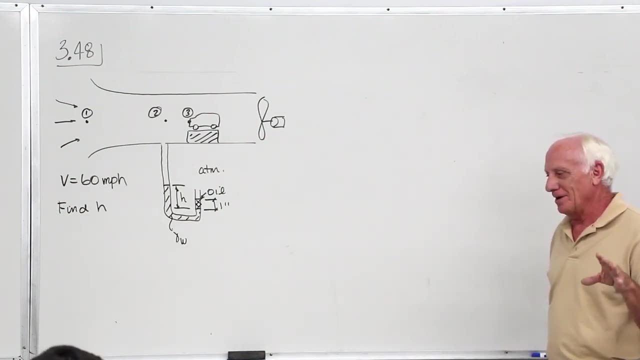 one of your first goals, of course, draw the picture. You cannot solve a problem without drawing the picture. okay, You've got the picture drawn. Now you've got to pick the points that you think you want to write: Bernoullis from where to where? 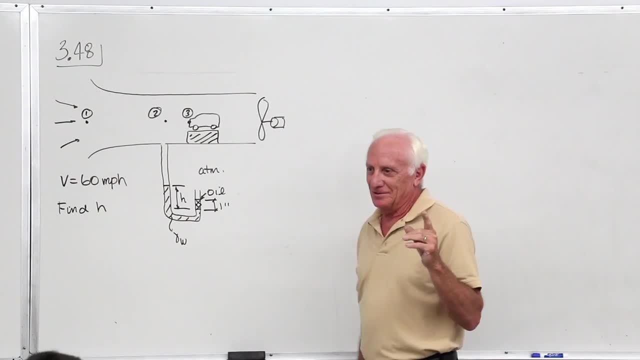 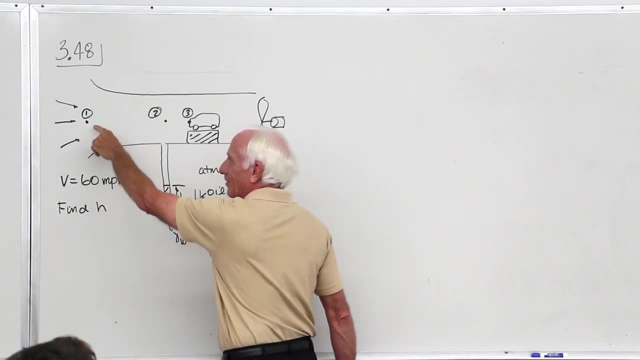 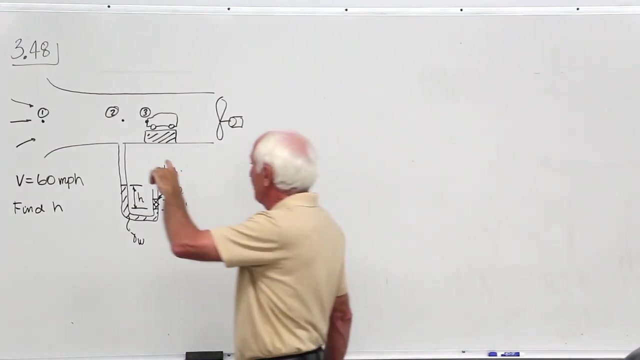 Okay, and I told you what you do. Number one: you look at where you know something. okay, I know the velocity at 1.. It's 60,- good, I'll call that point 1, near the entrance. I know the pressure at 2, sort of because there's a hole in the. 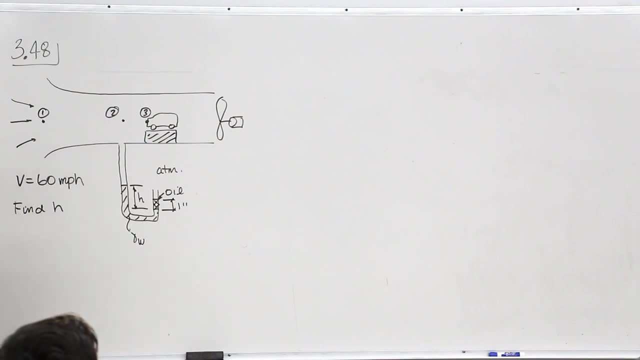 duct right there, the wind tunnel, And there's a manometer attached to it. What's the purpose of the manometer? To allow you to calculate the pressure pressure. We did that in Chapter 2.. Okay, so I do that too. Now I also know that. 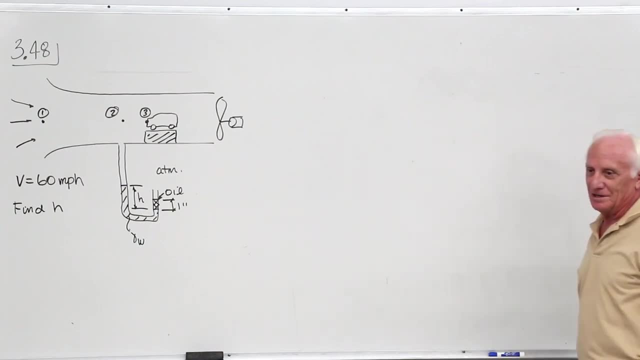 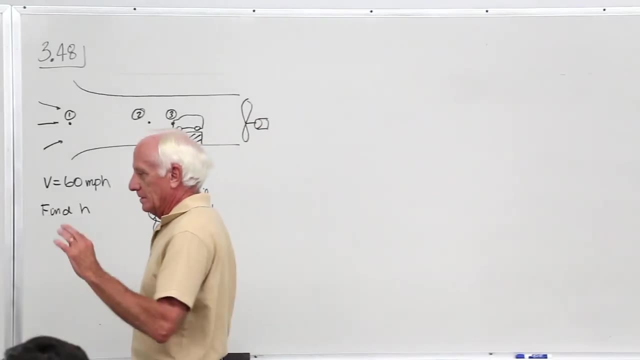 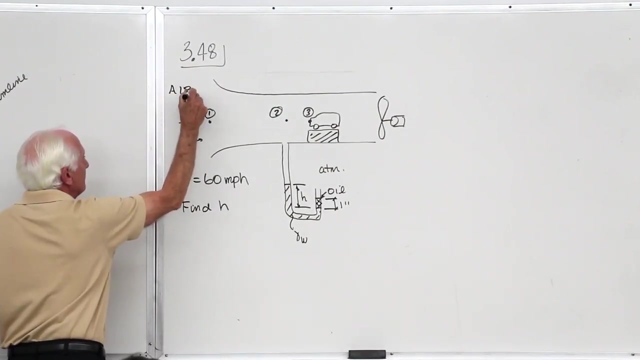 the front of that van is called a stagnation point. We talked about stagnation point. Stagnation point is where the velocity is brought to rest, or zero, The front of the van. the velocity of the air there is zero, By the way. it's here, So 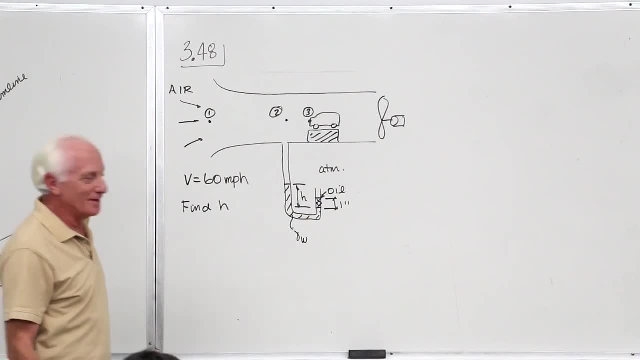 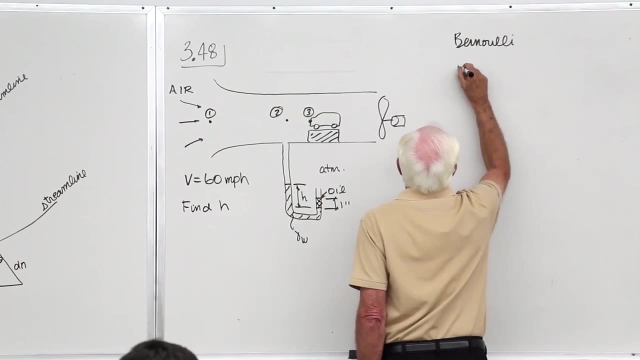 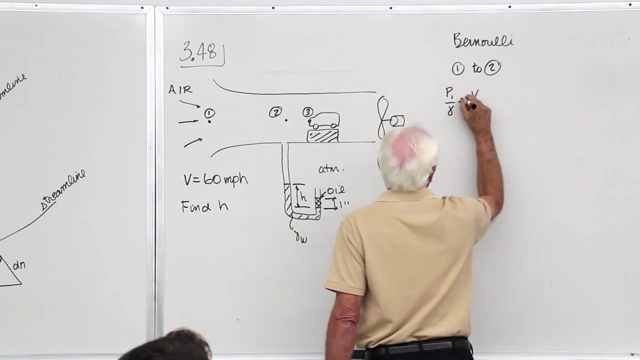 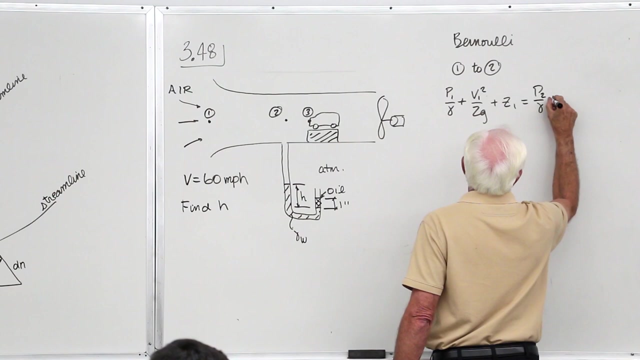 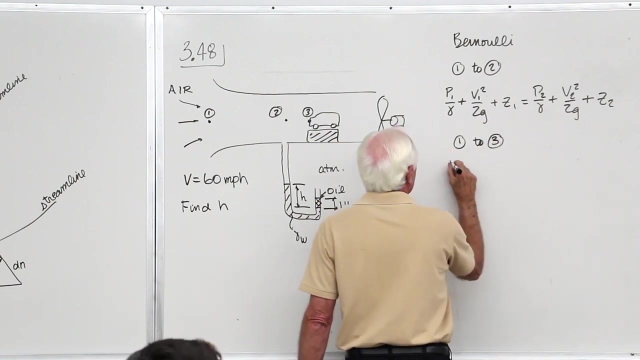 there are three possible points to write Bernoulli's: from where to where. So, Bernoulli, let's go one to two: P1 over gamma plus V1, squared 2G V1.. Oh, let's try another one: Bernoulli's 1, 2, 3.. Right, Maybe Bernoulli's 2 to 3.. 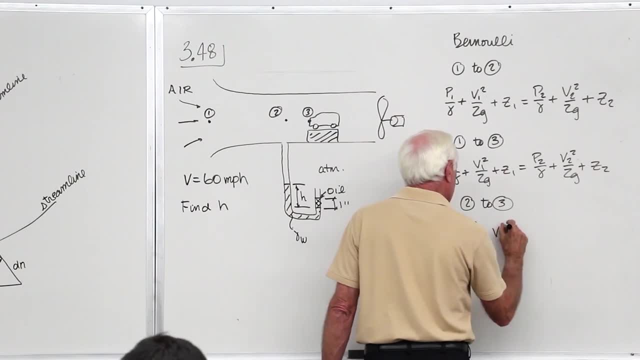 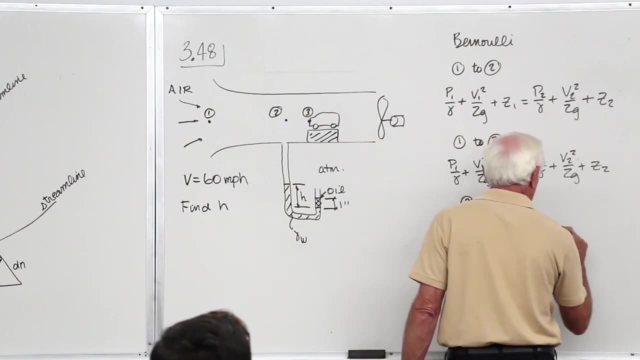 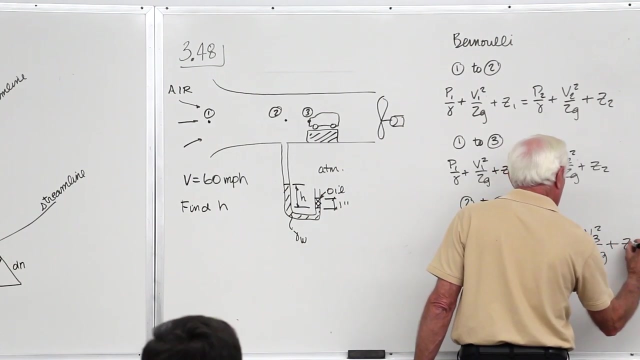 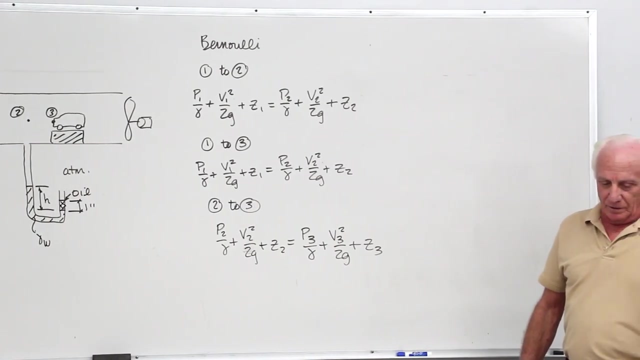 Now I told you before too: when you write Bernoulli's, the lower number- 0.1, should always be where the flow is coming from. 0.2 is where the flow is coming from. 0.2 is where the flow is coming from. 0.2 is where the flow is. 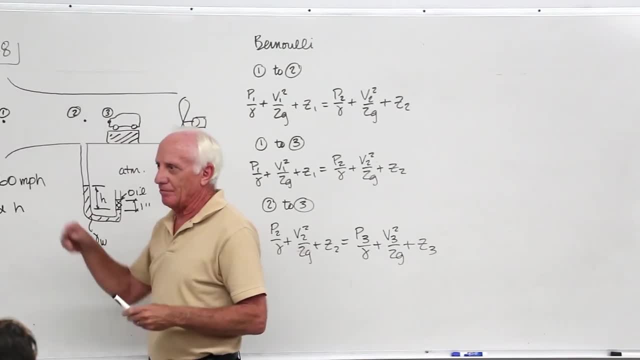 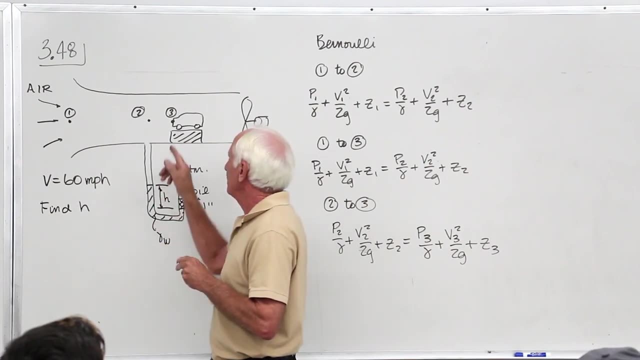 ending up. So don't write Bernoulli's 2 to 1 backwards- No, that's bad. Don't write Bernoulli's 3 to 2 backwards, That's bad. No, don't write Bernoulli's 3 to. 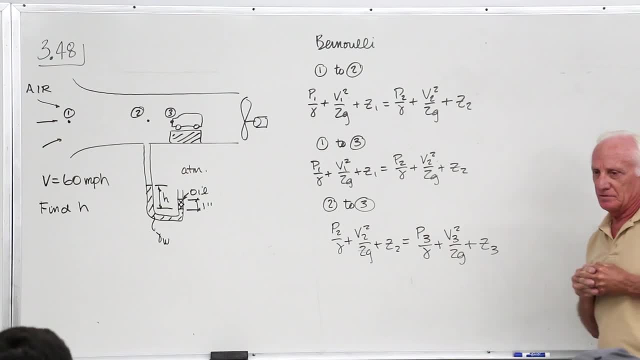 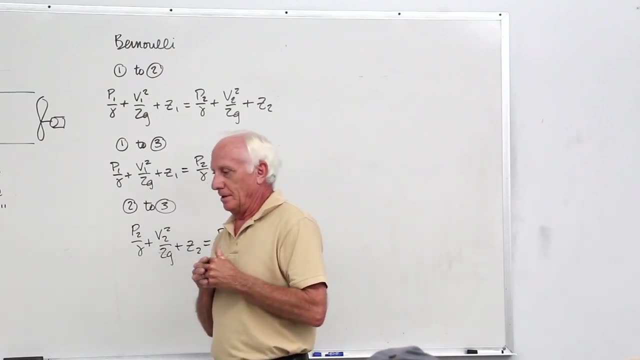 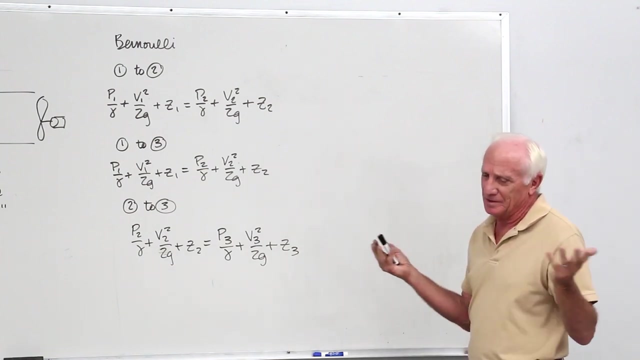 1 backwards. That's bad. Bernoulli's- from where the flow starts to where the flow ends up. Write it in that direction. We'll just review: Is Bernoulli's applicable? Okay, let's go through it. Is it a steady state? Yes, it's a steady state. 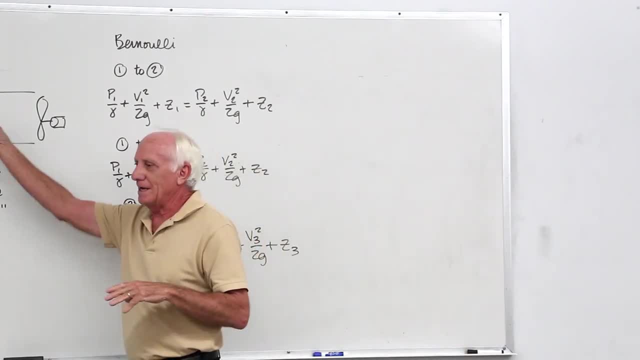 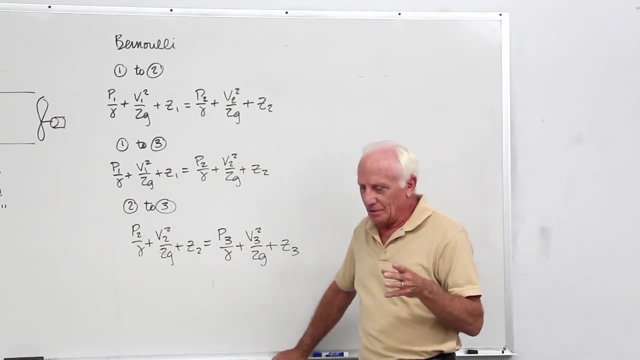 Incompressible. Yes, low velocity of air. Low velocity of air can be assumed to be incompressible. You probably know what the Mach number is for jet aircraft or commercial aircraft. Speed of sound: Mach 1, speed of sound. Normally, if the Mach 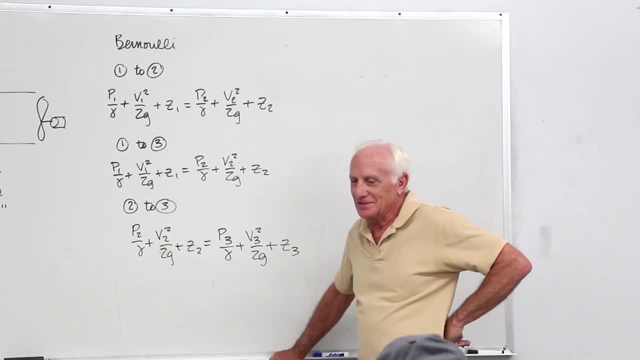 number of air is less than 0.3, air is treated as incompressible. This is low velocity air. I don't think this van is going Mach you know 0.3.. I don't think this van is going Mach, you know 0.3.. This is low velocity air, I don't think. this van is going Mach, you know 0.3.. I don't think this van is going Mach, you know 0.3.. I didn't know that was 0.5.. No, So it's low velocity, So we know it's. 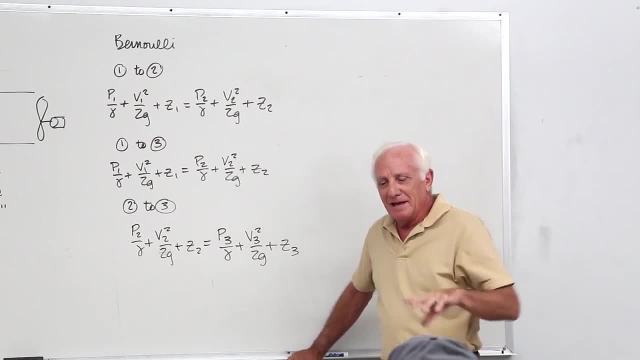 60 miles an hour, It's not anywhere near Mach 1.. If the Mach number of the gas is less than 0.3, then you can assume it behaves as an incompressible fluid. Okay, it's incompressible, So steady, incompressible. We're neglecting. 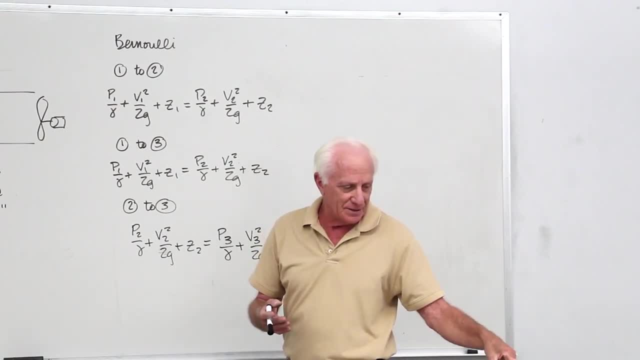 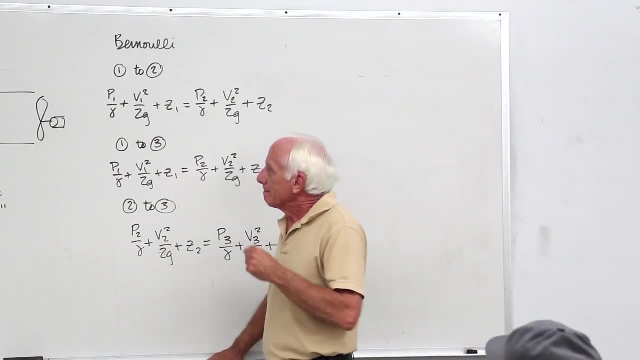 viscosity. Yeah, the problem said: unless I say otherwise, neglect viscosity. If the problem says you know, include viscous effects, then okay, but this one like viscosity. Oh, and along the streamline. Yeah, it's along the streamline. The. 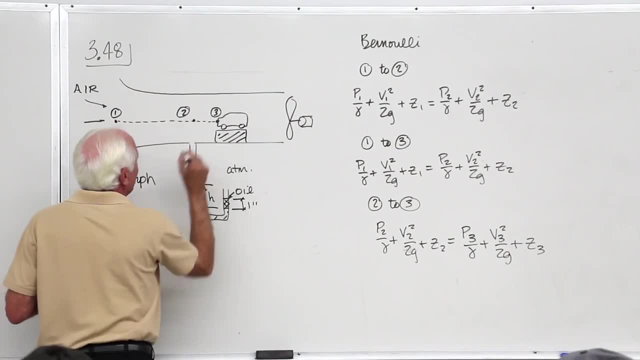 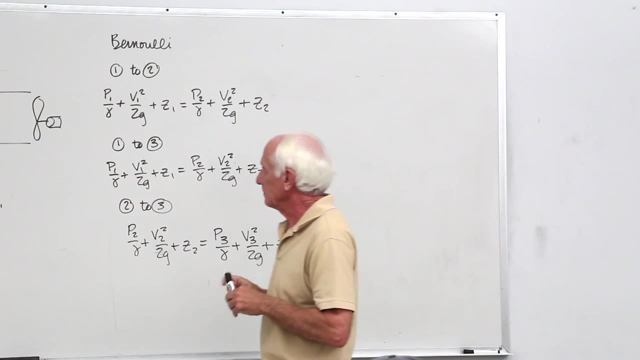 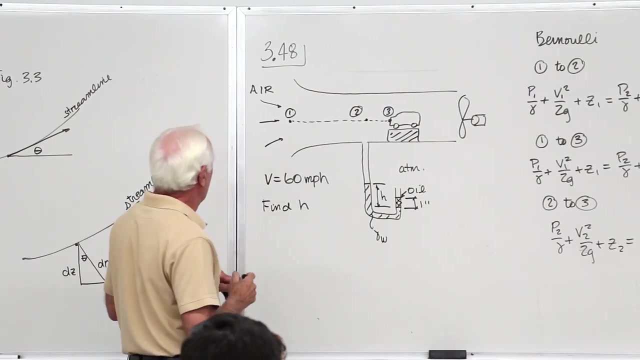 streamline goes from here to 2 to 3.. That's the streamline. You could follow a molecule of air as it did that. Now let's try and simplify each of the three renewables if we can. if we can Do I know. V1? Yeah, 60 miles an hour, Got it. 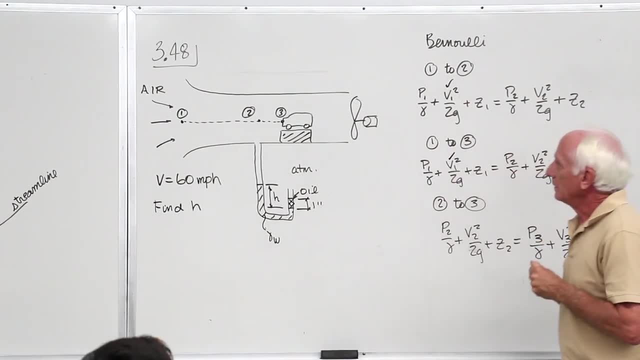 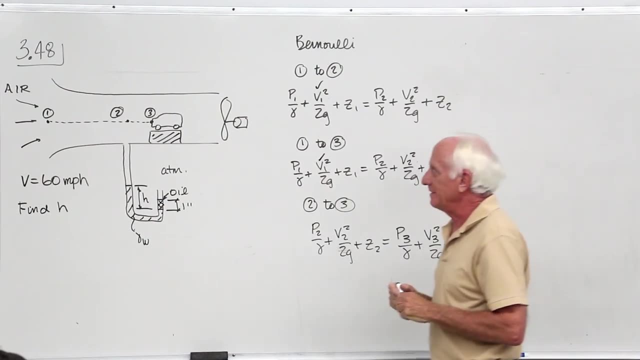 Got it Okay. Do I know Z1, Z2, and Z3?? No, but they're all the same: Z1, Z2, cancel, cancel, Z1, Z2, cancel, cancel. I got Z2 up there. Oh, where did I go? 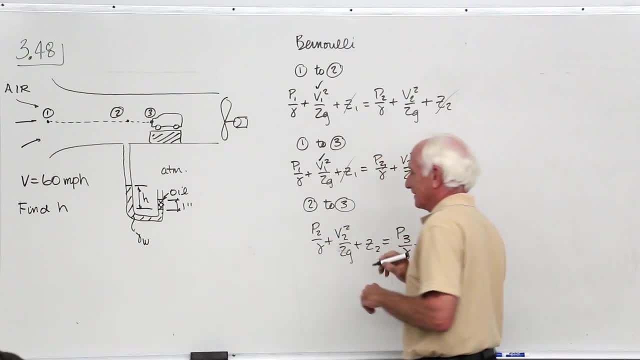 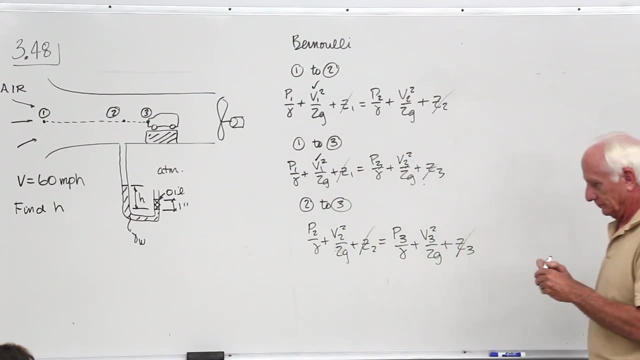 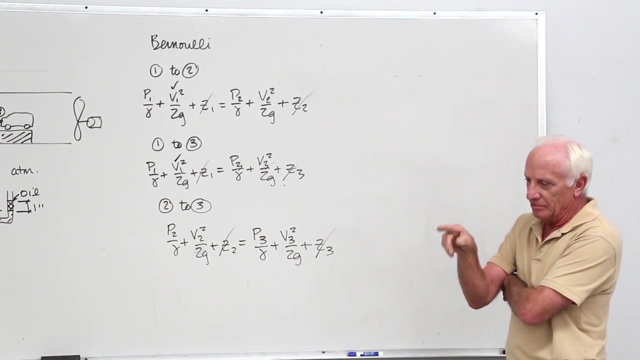 One of the three. thank you. Three, three, three. cancel. Thanks. Z2, Z3, cancel, cancel. Okay, See, one by one, you go through these guys. Sometimes you don't know which equation you want to use If you don't write them. 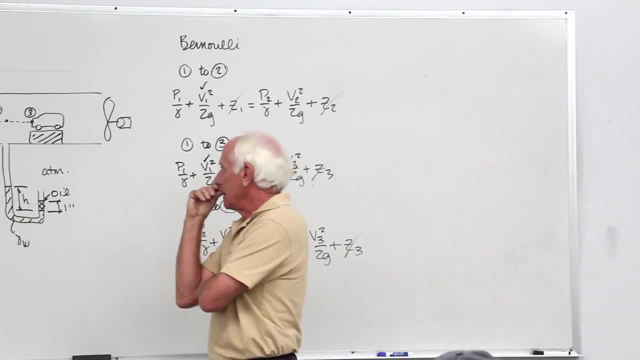 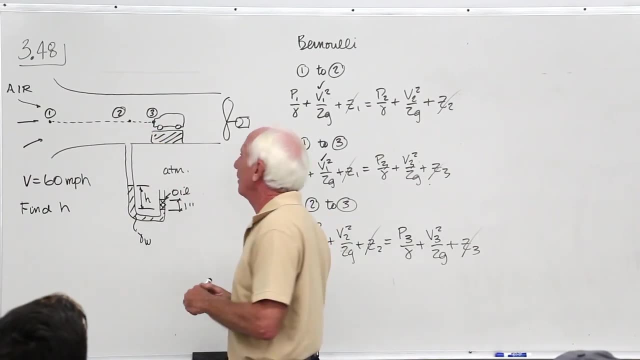 all down and think about them a lot. Okay, Now we'll get to the harder stuff. Oh, you know what stagnation point is? It's the point in the flow where the velocity is zero. Okay, V3 is zero Gone. V3 is zero Gone. 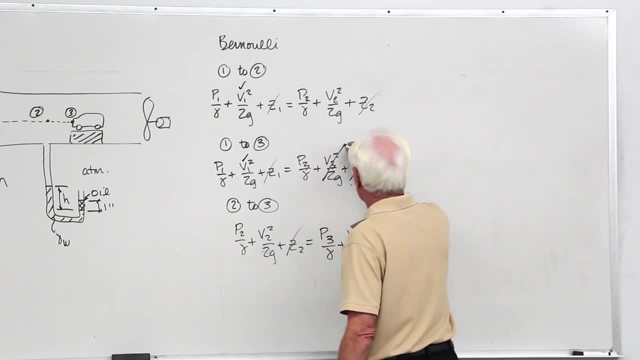 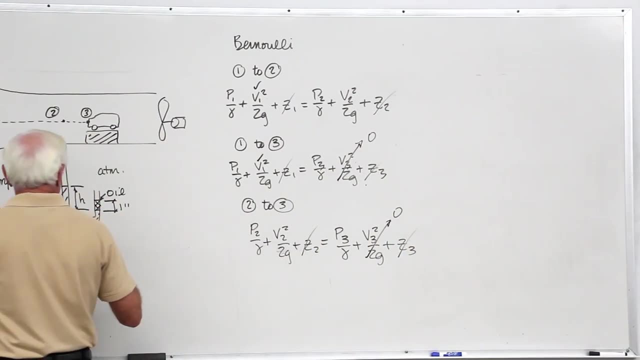 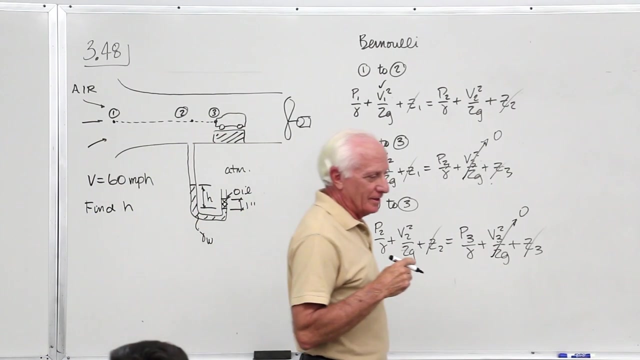 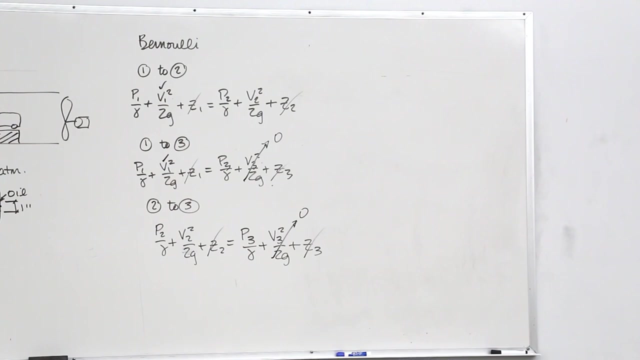 Okay, Oh, that monomer is there for a reason. I told you the reason. This is going to give us pressure. at point two, Let's review pressures. Is it going to give me the dynamic pressure, the static pressure, the total pressure? I told you, if you drill a hole, you're going. 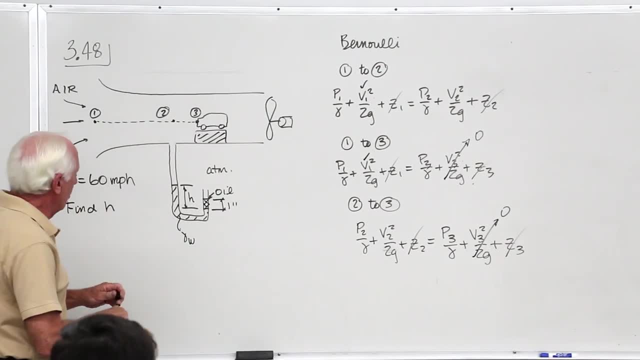 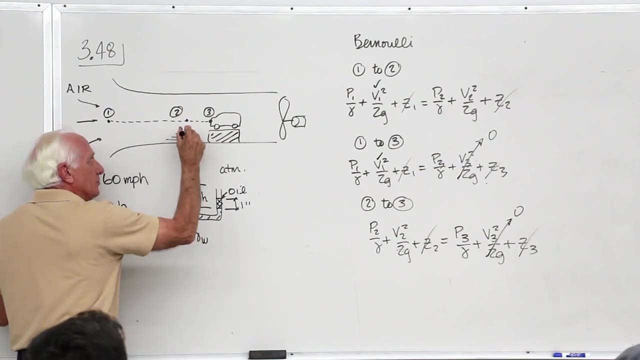 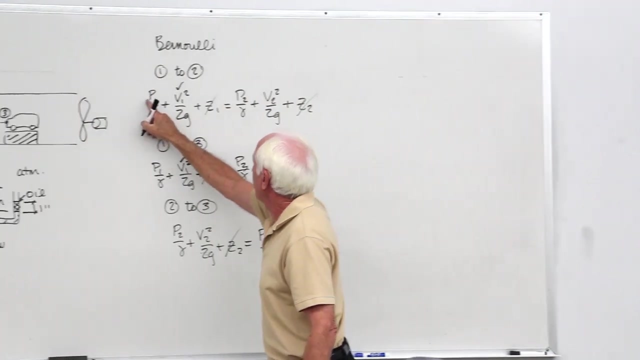 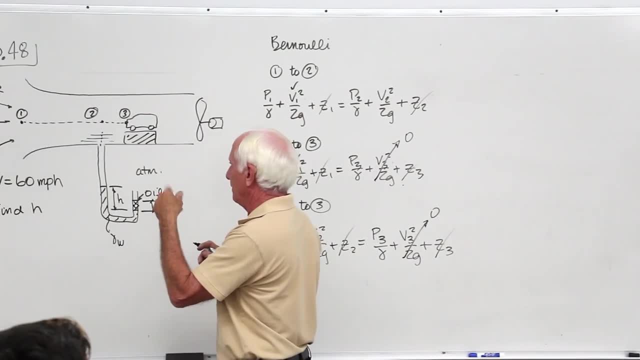 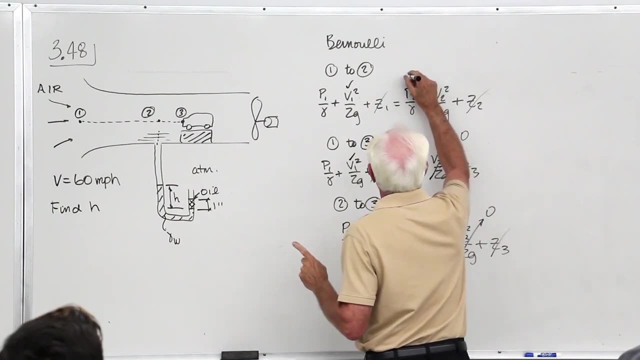 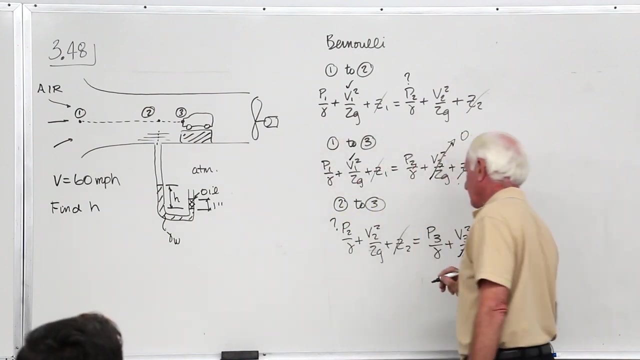 Okay, So can I find? I can't find P2, but it has H in it. okay, It has H in it. So what I really want to do is I want to find that P2 so I can get that H. Okay, Now look. 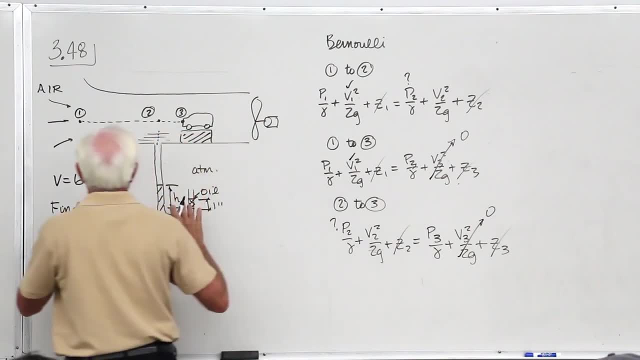 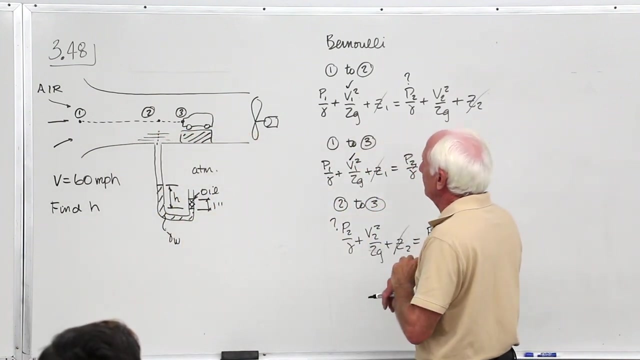 at the picture. My picture is out of kilter. a moment here. The velocity here is 60, okay, 60, zero. 60, 60, zero, Okay, All right, Good, Okay, okay. v1, v2. same thing. v1, v2, v1, v2, v3, v1, v2. I know it. 60, okay, we're supposed to. 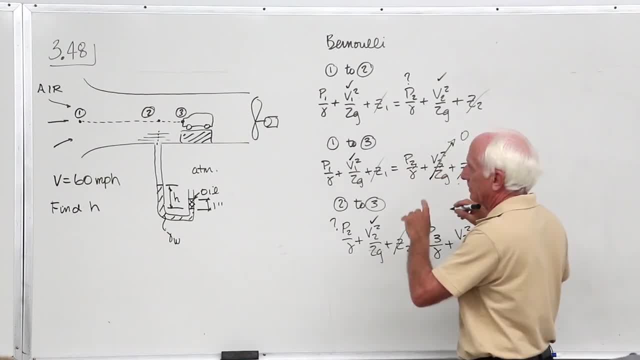 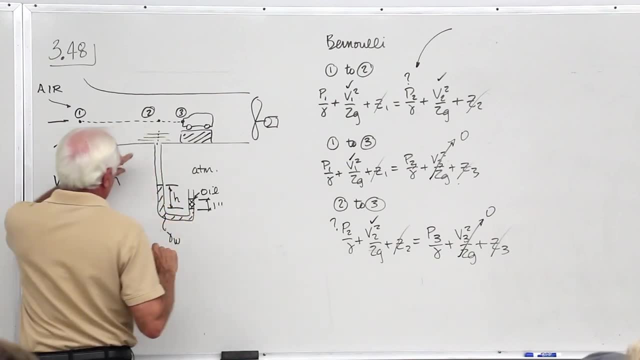 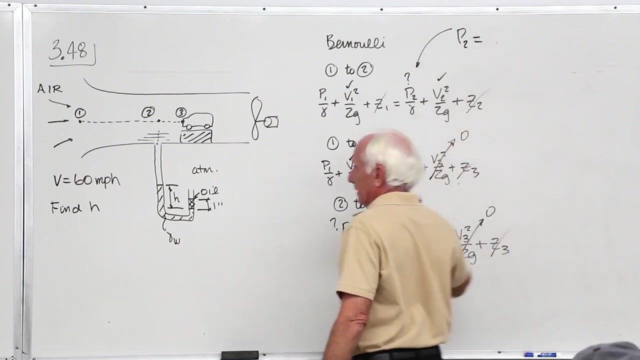 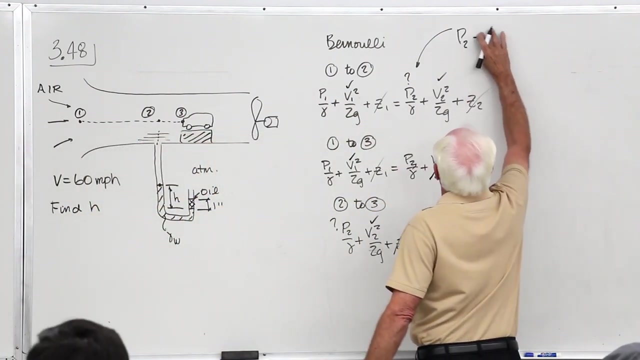 solve for H. okay, start here p2. okay, pressure down there, p2, the same. don't forget we neglect the density of air. okay, pressure here, same as the pressure here. pressure here, women, to compare the water is negligible. okay, now we go down in water. go down plus sign how far down. 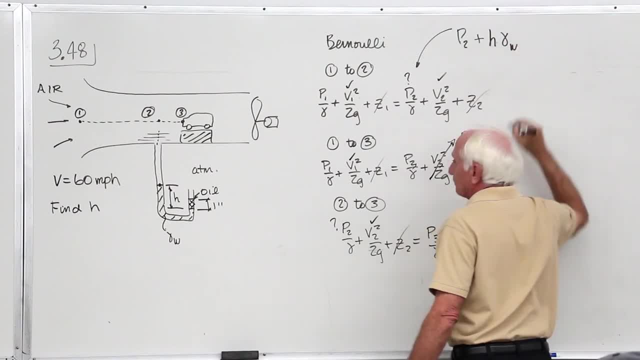 H. what fluid gamma water? stop right there now go across horizontally. look right there, same fluid continuous line, take my finger. continuous lines saying fluid. conclusion: the pressure here and the pressure here is the same. okay, now I go up. minus. in what fluid oil? how far? 112, and what's the? 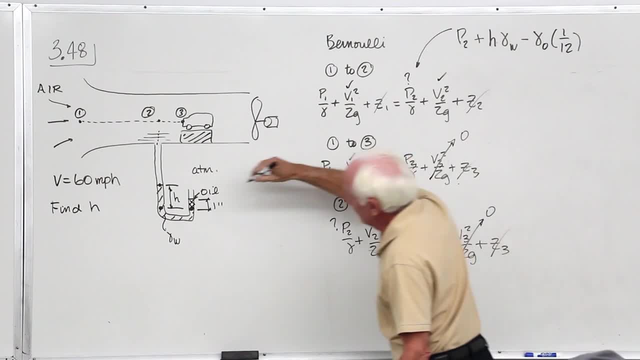 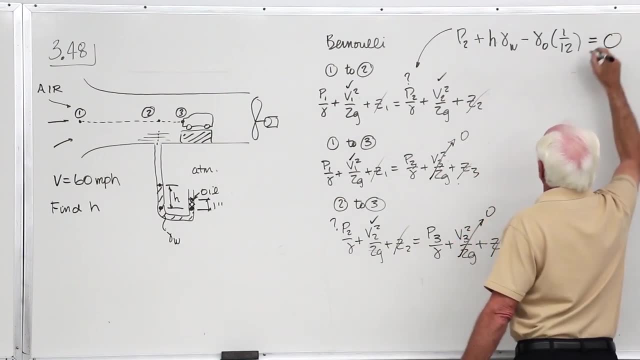 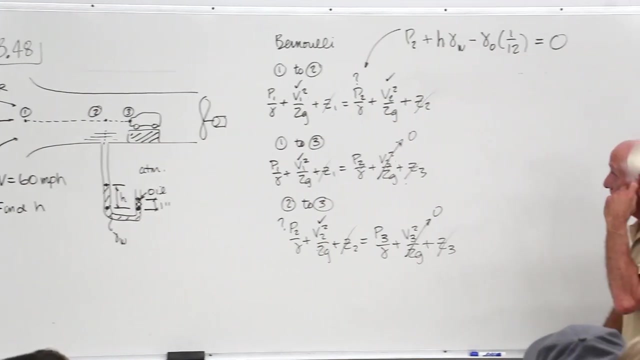 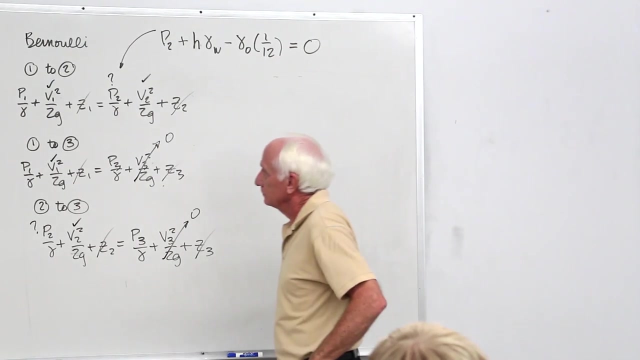 dotted line double, still 12, 3. What's the pressure at the dot right there? Well, I put up there for you atmospheric zero. Put that P2 in that equation right there. okay, Where did the air come from The room? 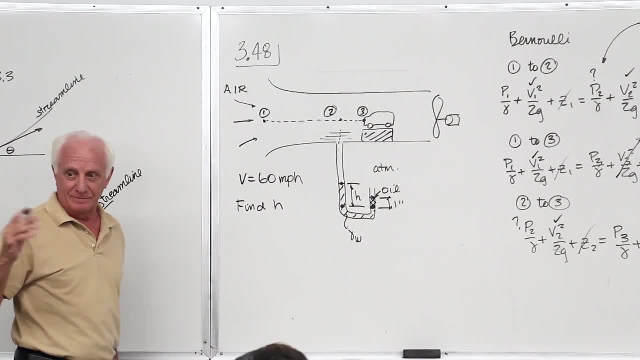 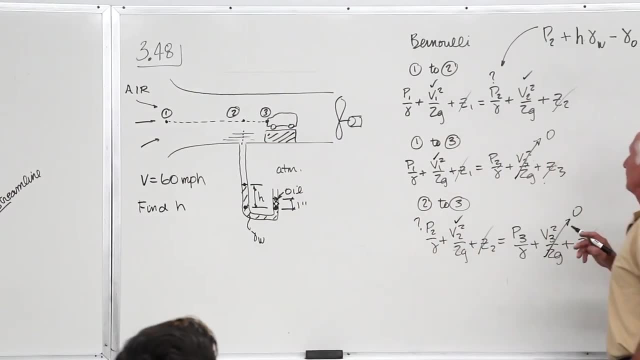 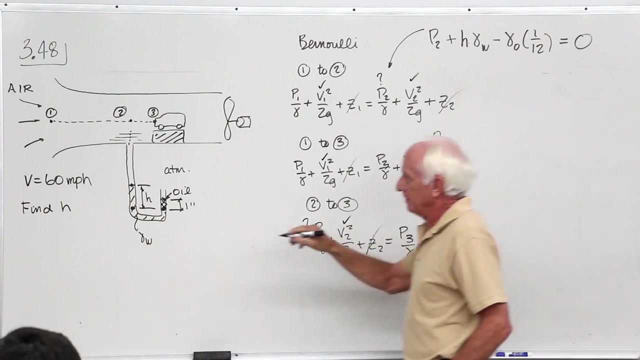 What's the pressure in the room? Zero PSI gauge. What's P1? Zero, Okay, Go ahead and solve that guy. That's part A. Part L, Part A: Fine stagnation, pressure. Fine P stagnation, Okay. 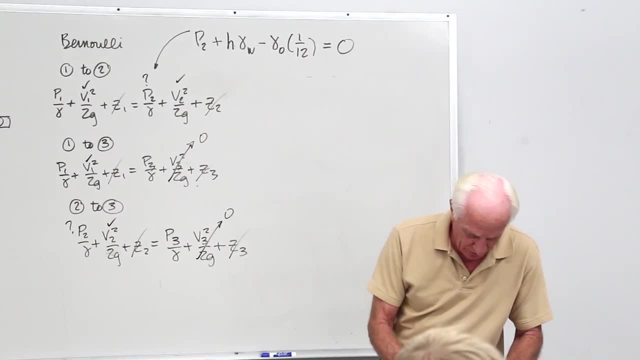 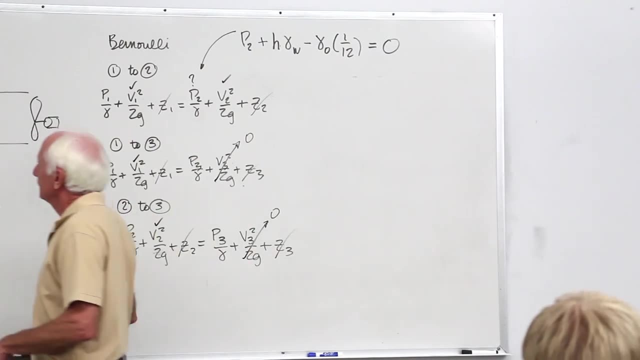 And again, you've already worked this for homework, so I'm just going over it just to explain a few things about this. Oh, I'm sorry, Let me just put this higher further. Yeah, I'm holding the hook close enough. 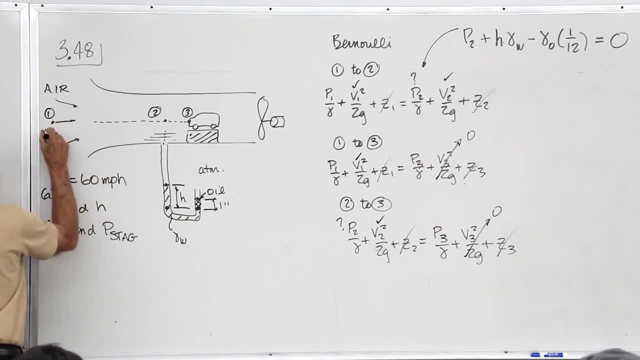 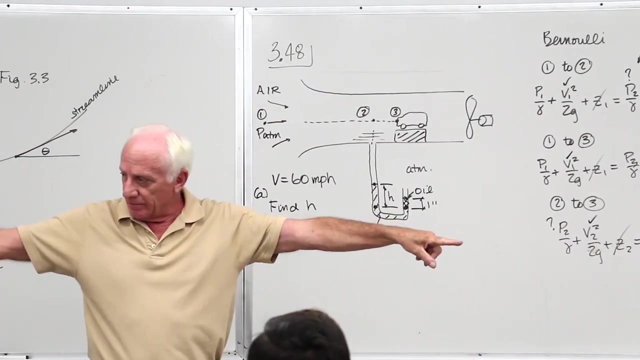 There's .1 right there. P atmosphere, P atmosphere. If you put the wind tunnel in this room, where does the air come from? that's going that way. air is coming out of there. Okay, The fan is over there sucking the air through. the air goes through here, hits the body of the van. 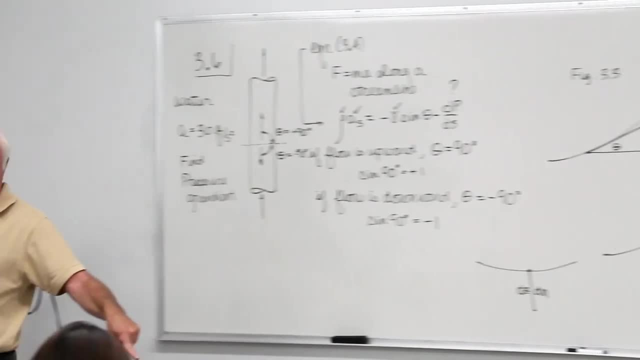 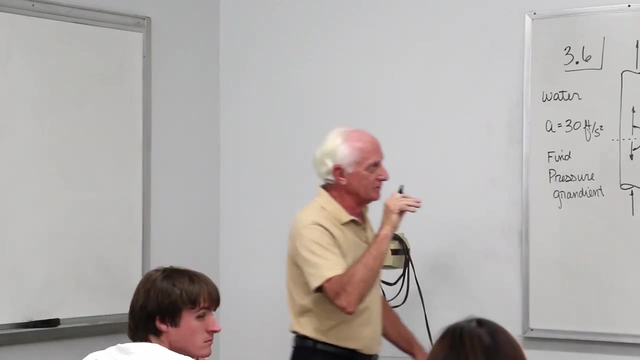 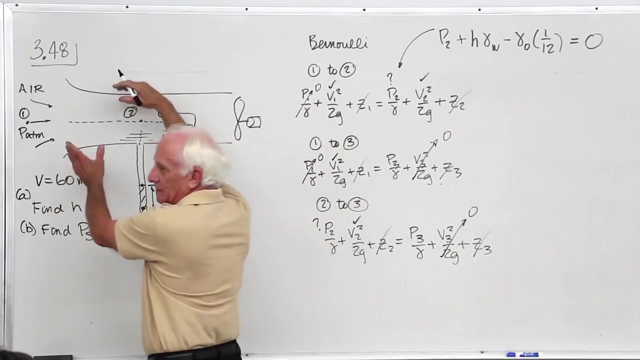 If I'm standing out here and the wind tunnel is right there, the pressure of the air is what The atmospheric pressure? zero. so P1 is zero. That's not a continuous duct. It stops here. It's a bell shape. 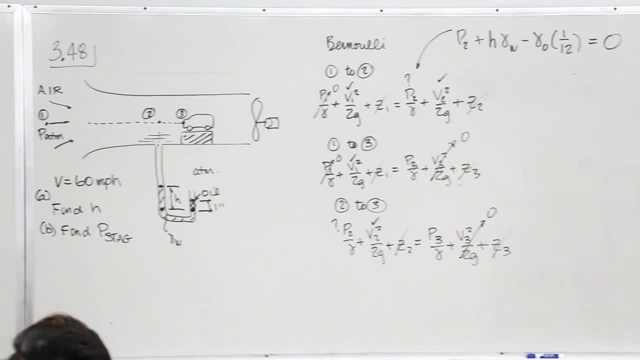 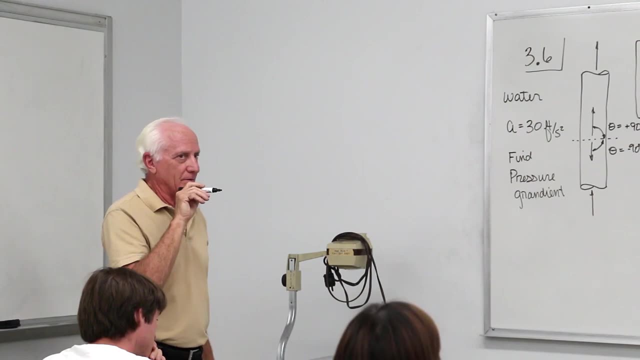 It's an entrance, It's a drawing area. If I'm standing over here, the pressure here is P atmosphere. If the wind tunnel is over there, what's the velocity here? Ah, zero, I'm so kidding. I need to put the air up here. 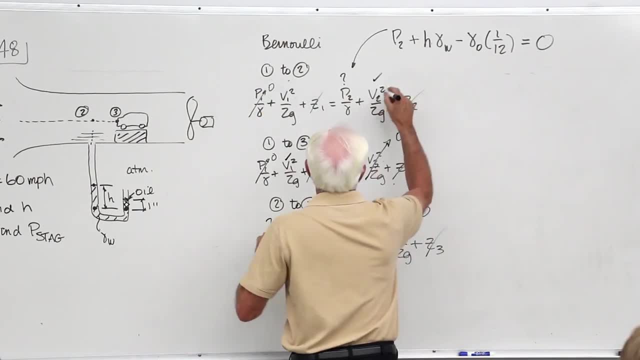 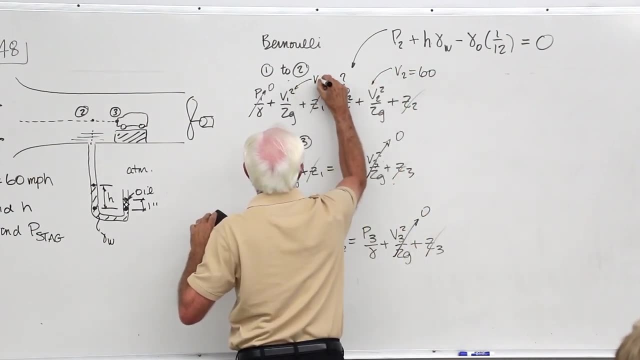 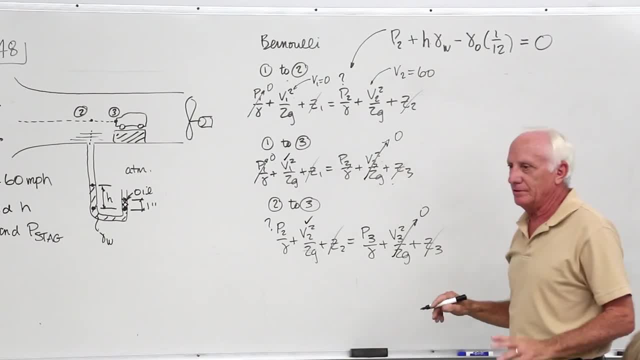 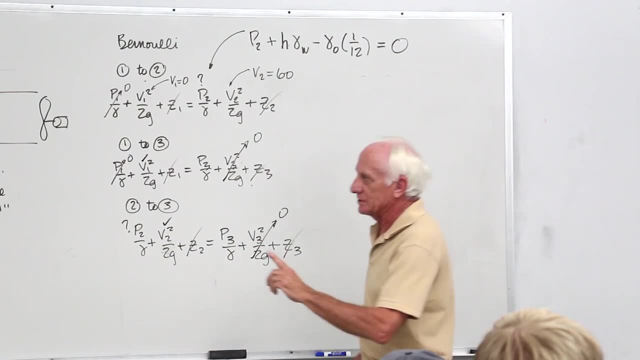 Plug, Plug, Plug, Plug, Plug, plug. put a P2 in here and solve for H. Okay, you can do that, I'm not going to do too much math. Find P: stagnation. Okay, where's the stagnation point Three, P3. 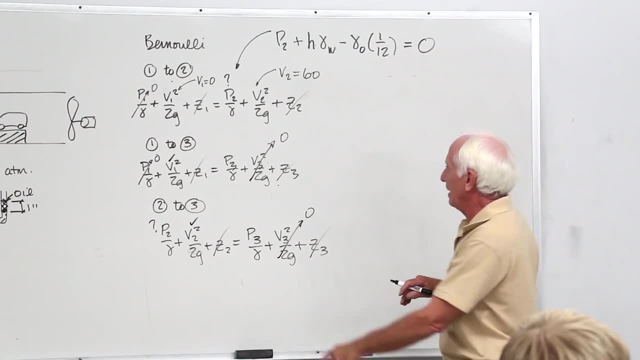 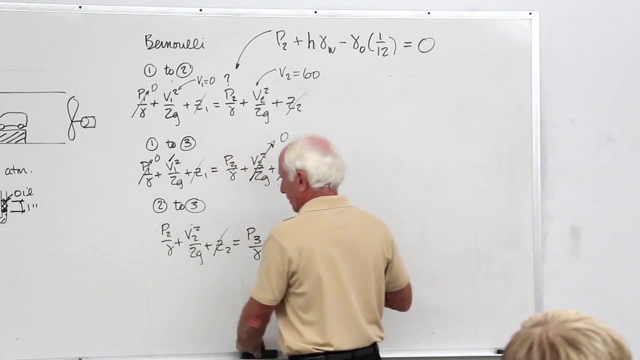 is not static, it's stagnation. Okay, where is a P3?? Here or here? Take your guess, Do you know? do you know P2?? Yeah, it's right here, you can solve for it. Yeah, you know P2.. Do you know V2?? Yeah, 60 miles an hour. Yeah, you know P2.. Can? 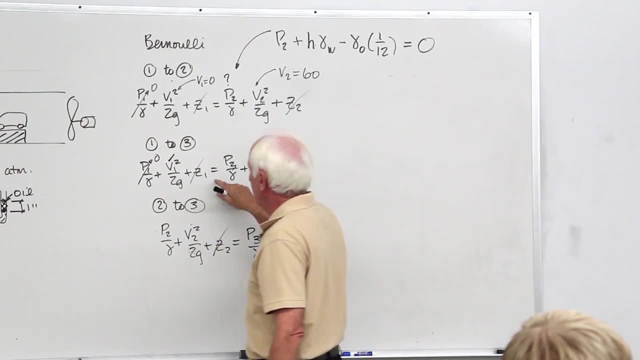 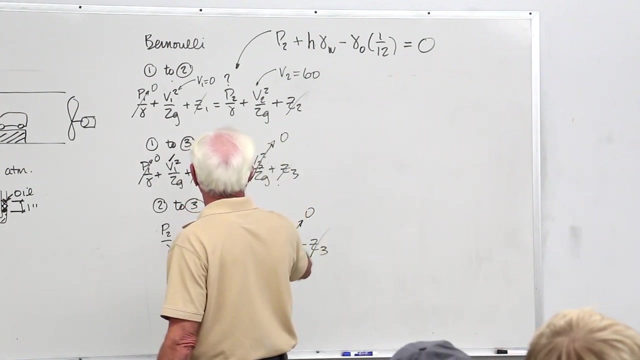 you solve for P3?? Of course you can Do you know. V1? Yeah, zero, P1, atmosphere zero, P3, zero. Our stagnation point three, Right here, that's a stagnation pressure three, 60 miles an hour, that's zero, Zero, zero, three, zero. Oh yeah, P yeah. 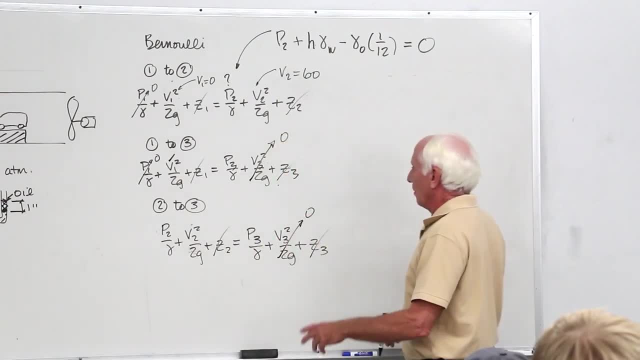 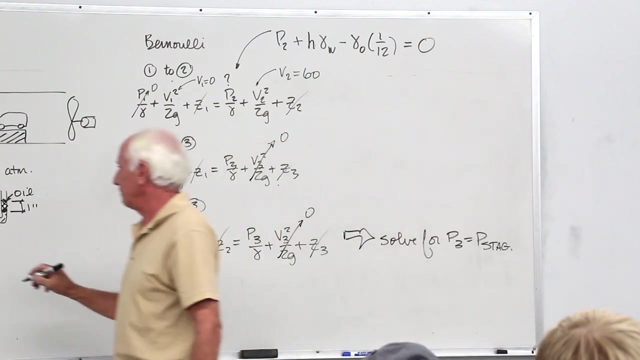 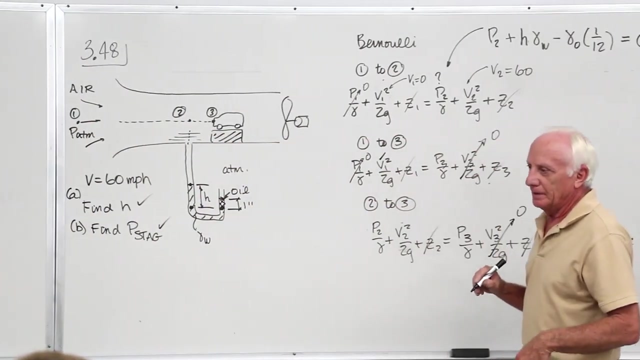 our P3 is a stagnation point, Okay. So from here I don't think we can use this guy. From here we want to solve for P3.. P3, which is equal to P stagnation, P stagnation, P stagnation. Oh, okay, why they put oil in there. You know, if 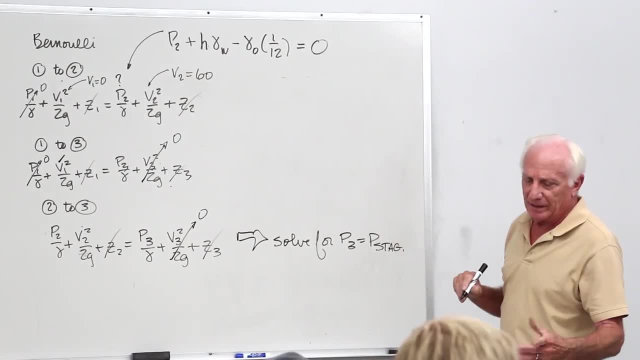 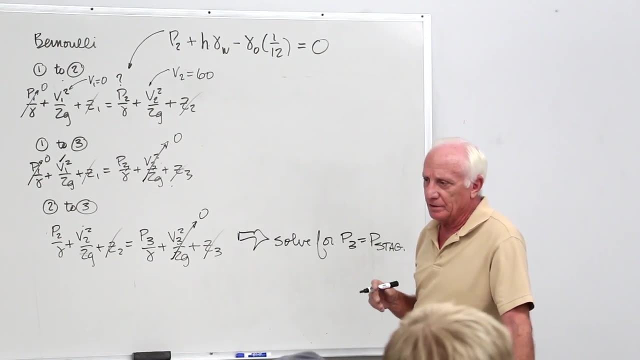 water is exposed to air, algae can build up. it gets greenish in color after time. it looks kind of crummy. So to keep the water clear, they put a layer of something on top of it, and oil won't degrade like water will with time. So they put a little. 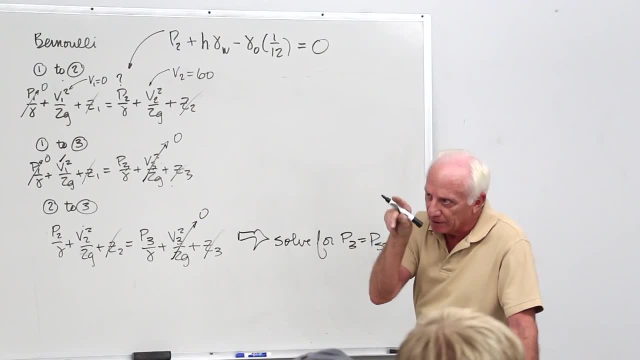 bit of oil on there to keep the water nicely clear. So you look at the manometer, you can see the delta H in the manometer. So that's what they do in that part. Okay, anyway, just a bunch of little things on there. The conclusion is: 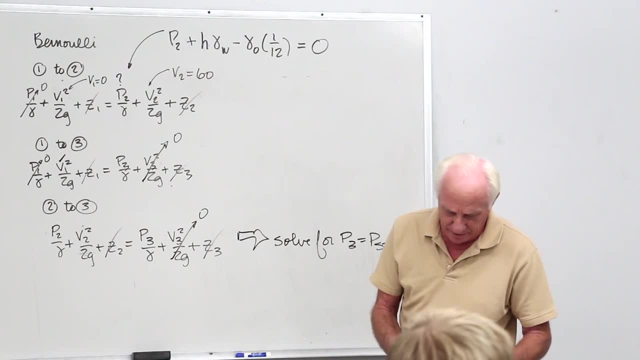 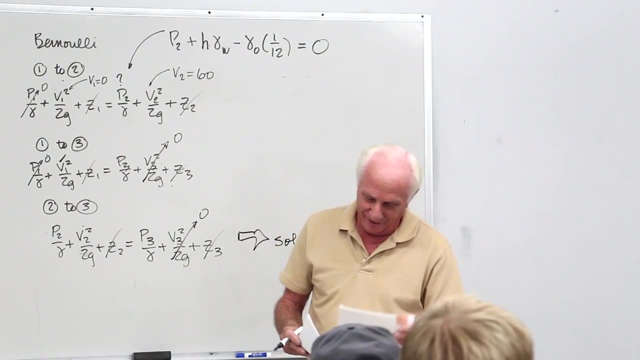 that sometimes there's many different Bernoulli's, so it's not just one Bernoulli, There can be many different Bernoulli equations, And the point there being, if you get stuck on an exam, write down whatever you think Bernoulli's. 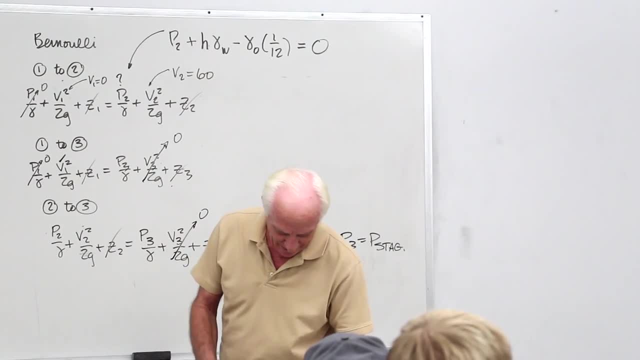 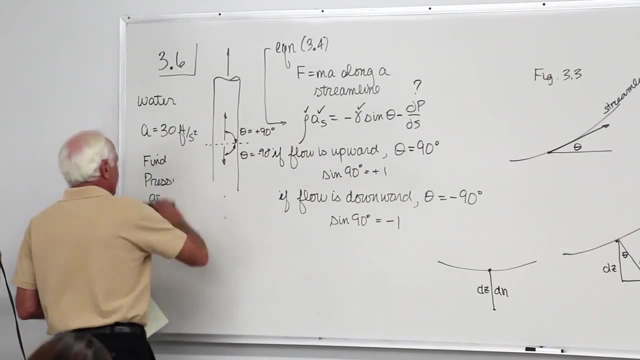 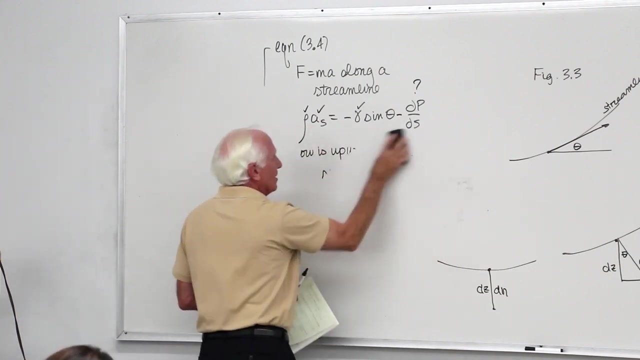 Bernoulli's you could use and then look at them, identify what you know and you don't know, and then go to the one in which you know the most stuff, or as easy as for you. okay, anyway, that's a homework. that was some. I had questions. 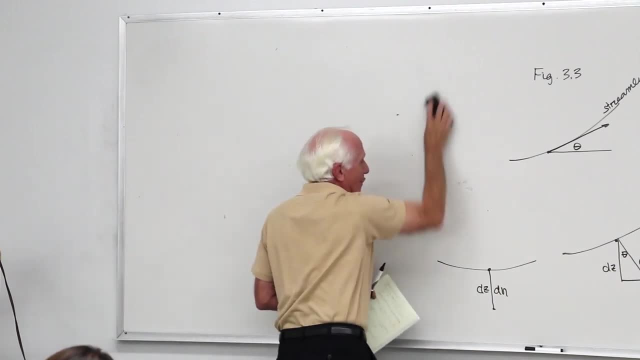 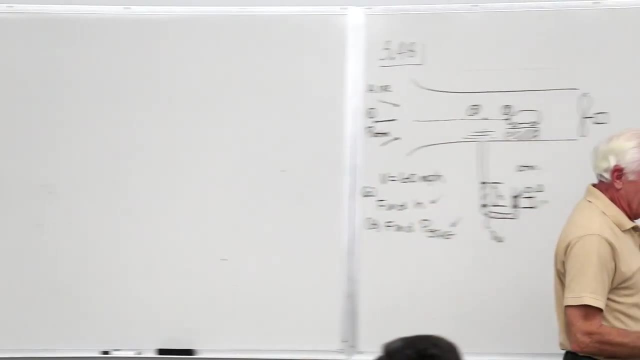 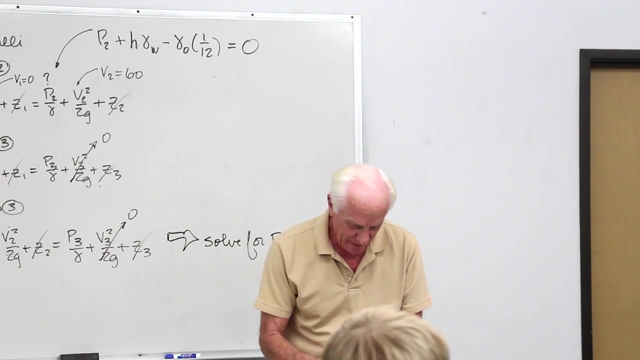 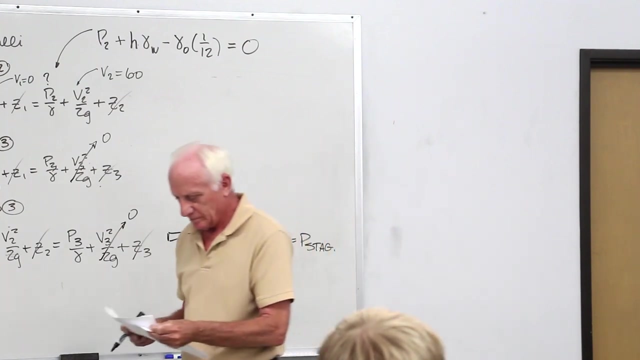 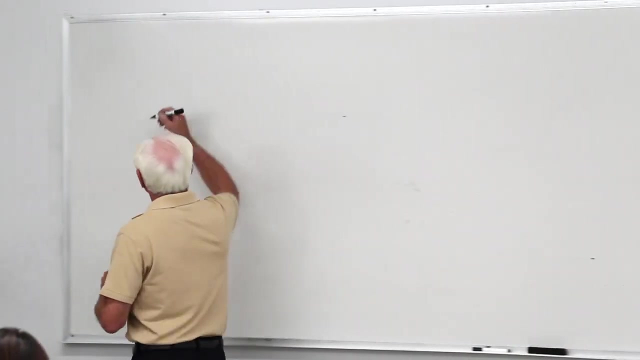 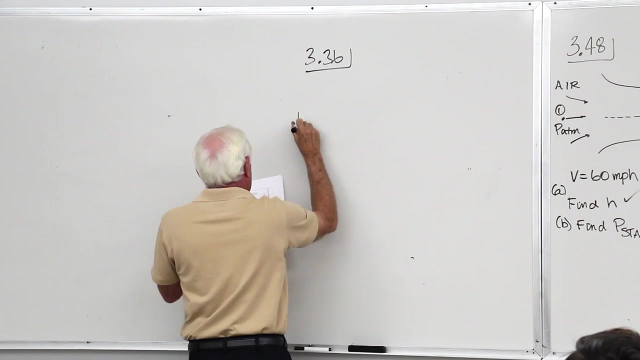 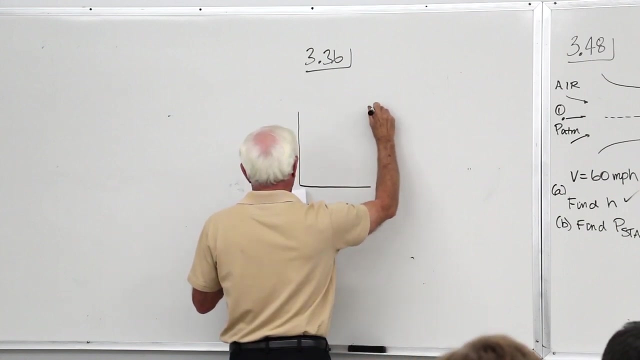 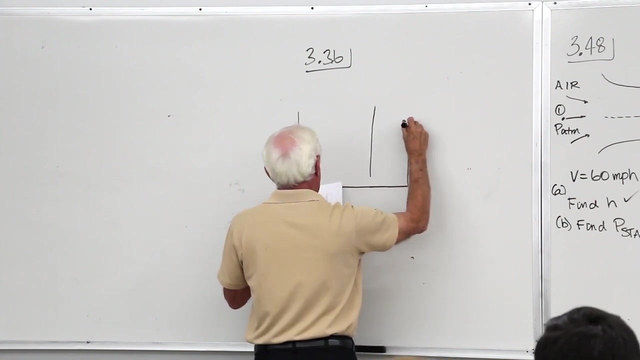 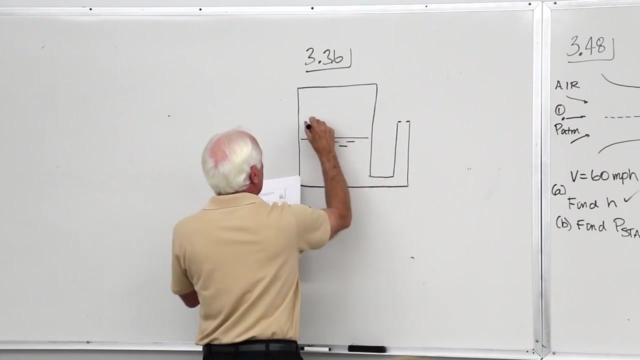 on. somebody had a question on that one too. there's problem 336. okay, there is a pressurized tank, there is a nozzle. it comes out of a two-inch diameter, comes out here pressurized water. it shows the water level down here. air here, pressure gauge up here, water down here. 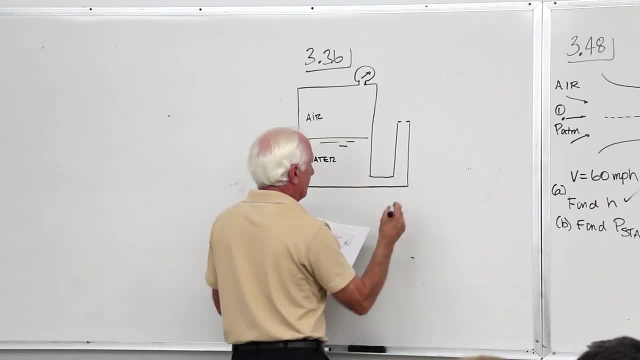 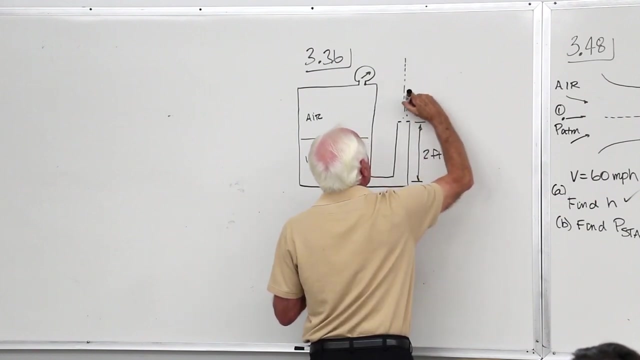 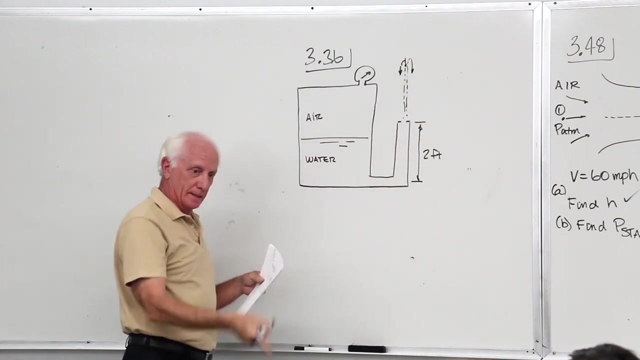 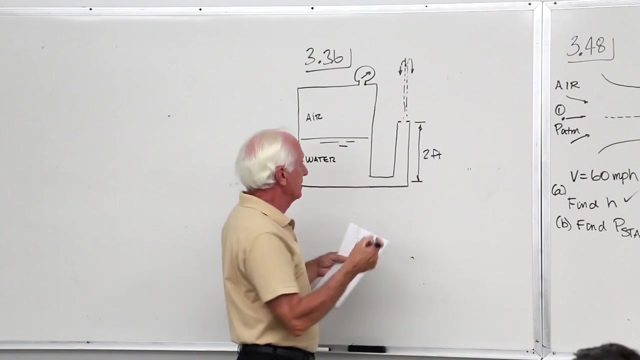 distances two feet. and here water comes out into the atmosphere and goes up to point to where it stops and comes back down again- a fountain effect. the height of that water just to the top is 20 feet. my drawings greatly out of scale, but that's okay. 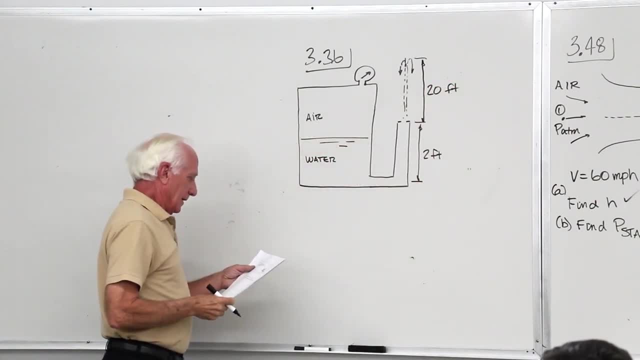 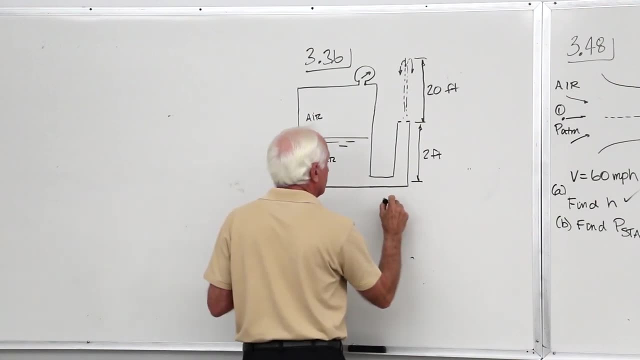 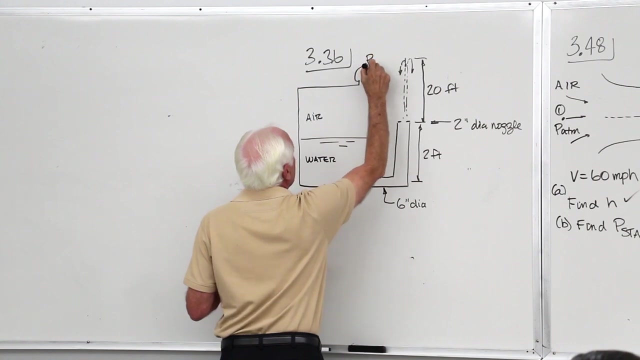 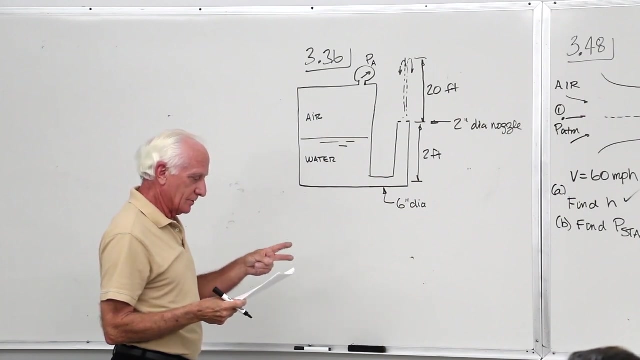 let's say two inch diameter nozzle and the pipe is six inches, okay, determine the pressure in the tank here, the pressure of the air in the tank if the flow is steady, frictionless and compressible. sounds like Bernoulli's. yes, it is steady, frictionless and 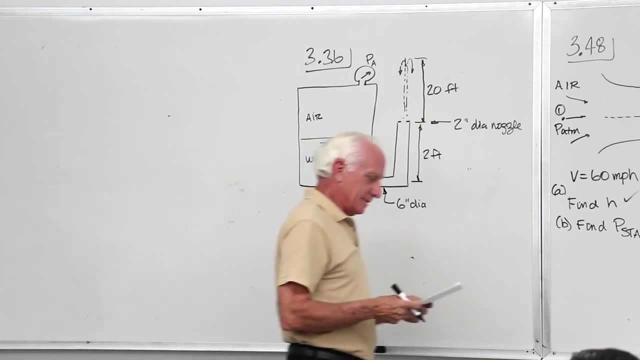 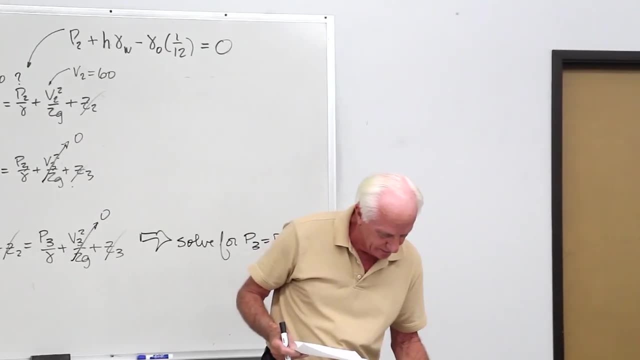 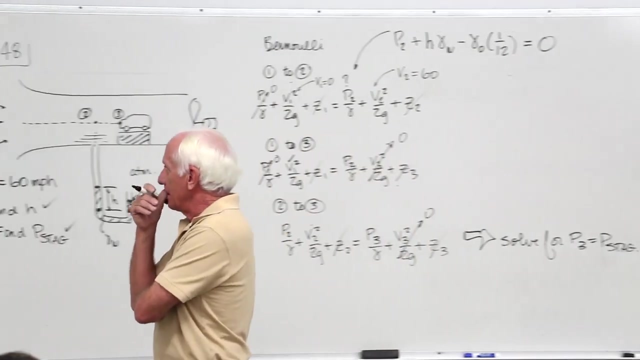 compressible. again. I think we see check 336. let me check for that. let me check for that. ok, ok, Okay, yeah, that's what it looks like. Not knowing any better, you might say: well, I'm going to write Bernoulli. 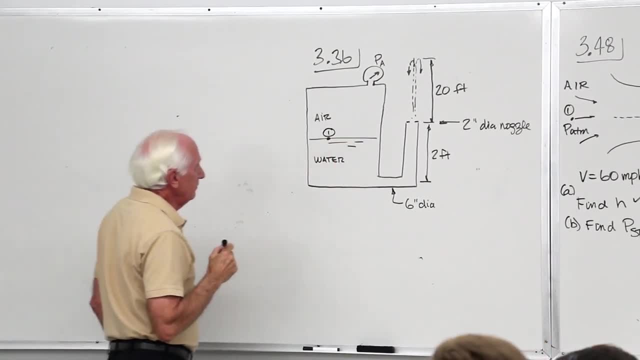 I'm going to call that one. Do I know the pressure there? Uh-huh, it's PA. I don't know it. I'm going to find it. It's PA, The velocity Zero. Okay, It leaves here. 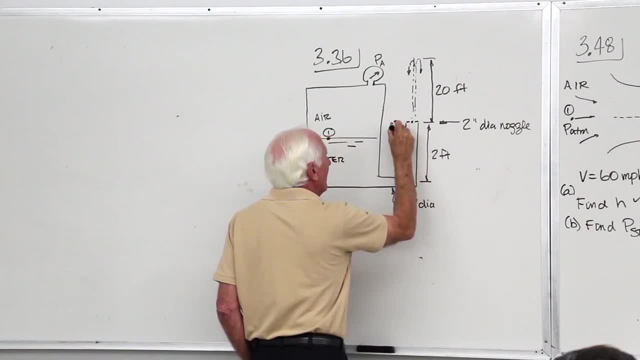 I don't know, Maybe I'll call that two, Why not? It leaves a pipe there. You know what? Here's the word: stop it going up. I'm going to label that 0.3. Why? Oh, I know one very good thing there. 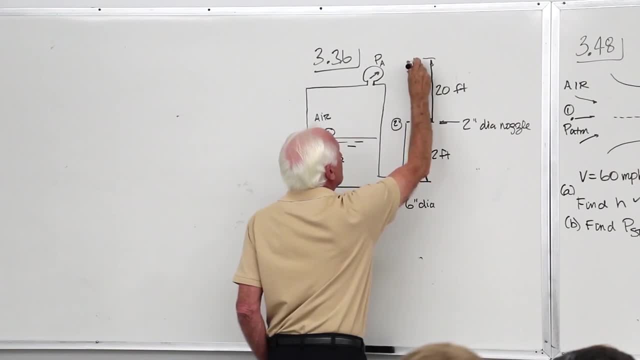 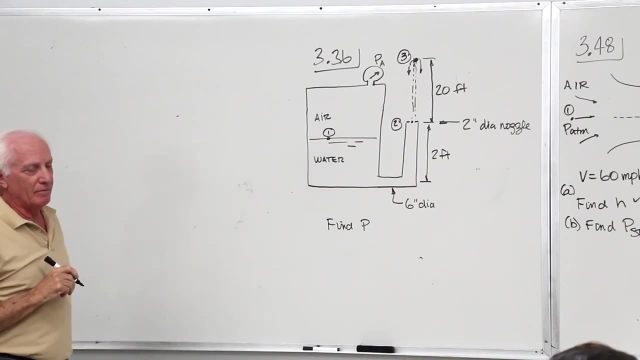 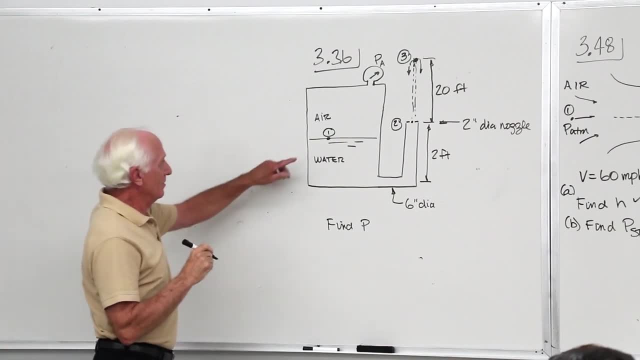 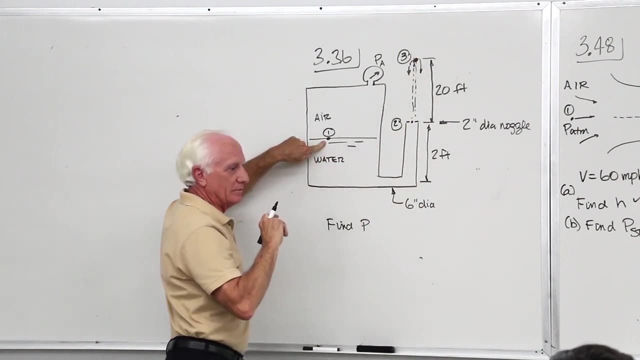 It's going to fall, It's going to fall down. So I know I don't know this pressure, I'm going to solve for it. I know the velocity here is zero. I know the velocity here is zero in the y direction. 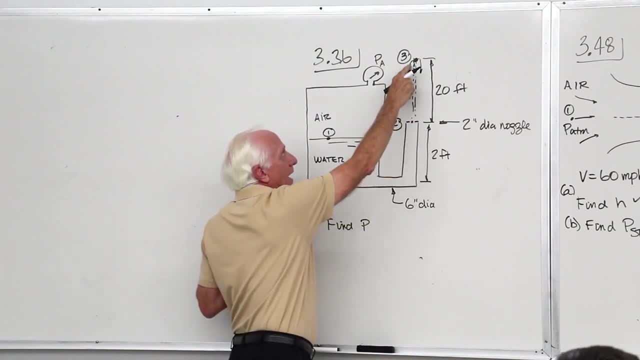 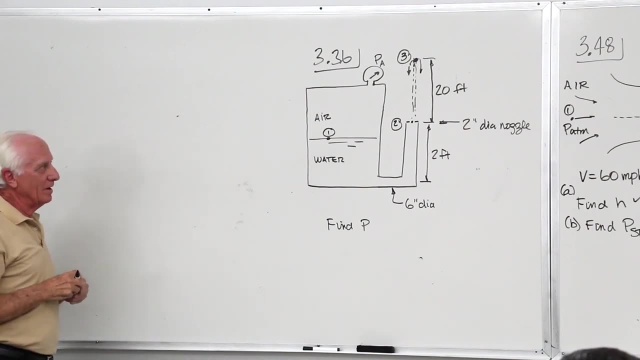 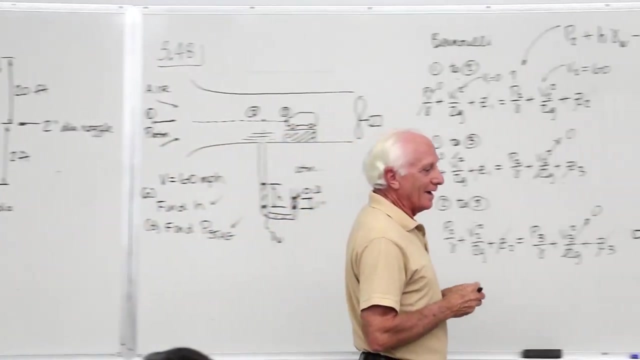 Here the velocity is not zero. I know the pressure at three It's atmospheric. You know what I think? I'll write for illusion: one to three, from one to three. Okay, You can do it that way. He well get z3.. 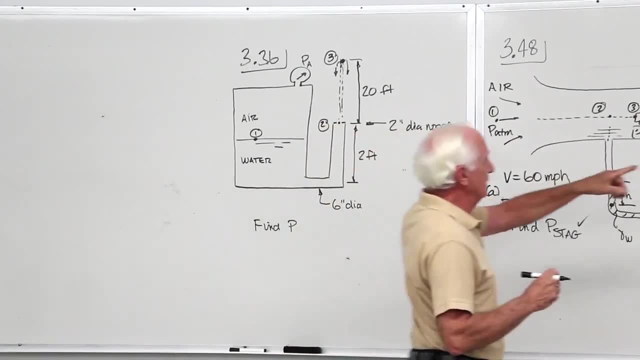 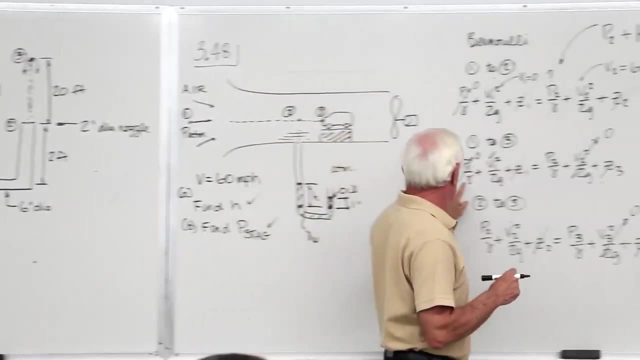 What's z3?? Okay, Because we need z3.. Like this, We need z3.. From one to three, We need z3.. We know We're summing for p1.. We know v1 is zero. We know p3 is atmospheric. 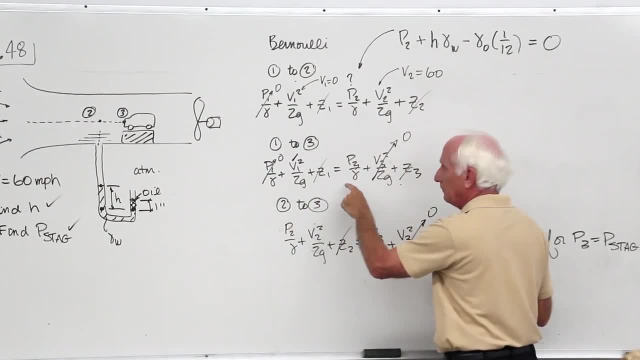 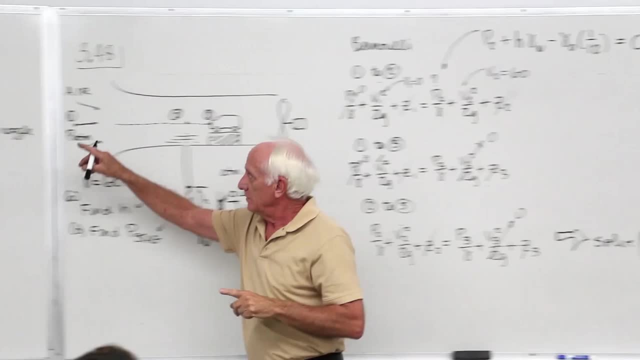 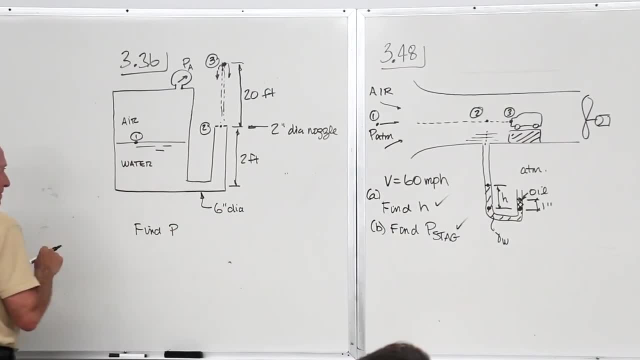 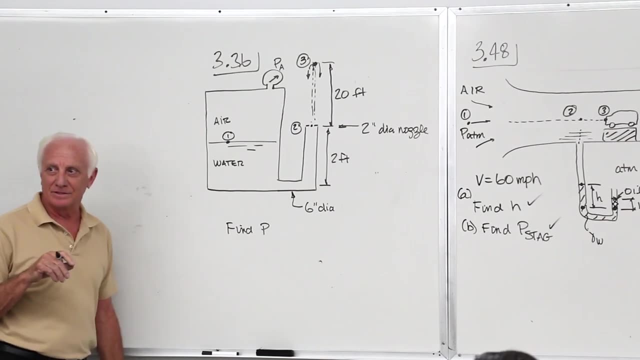 Above the data: Okay, Z1.. Put z1 in. I put z–I put z1 in. I don't know. You want to guess. I have no idea what z1 is. Don't dare say two, Don't dare say 22.. 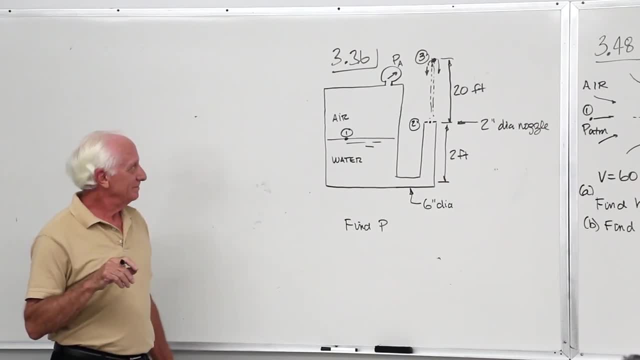 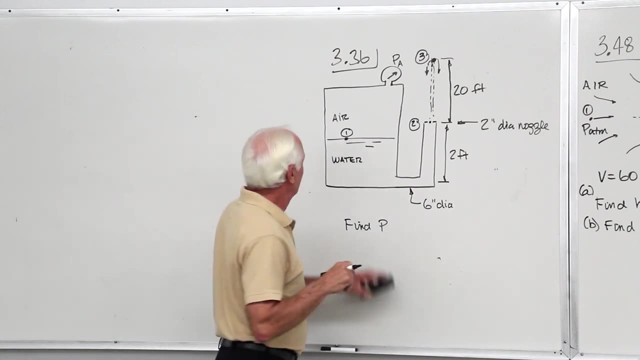 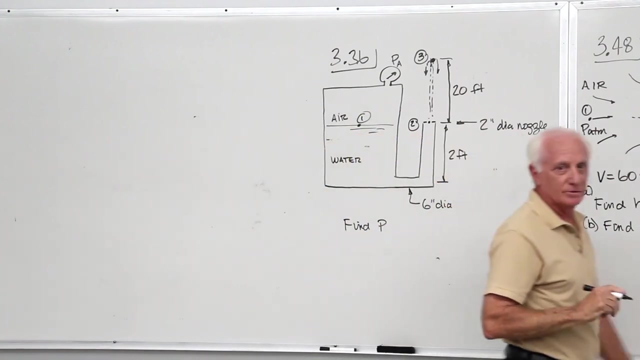 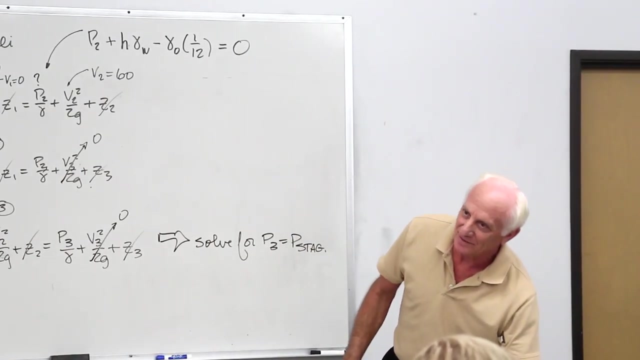 Don't dare say 20.. Why z1? z2? one? Oh, he made a mistake in the picture. okay, That's what a water level is. You wouldn't know that, unless I told you that, of course, Or you guessed it. Anyway, he mistook the. 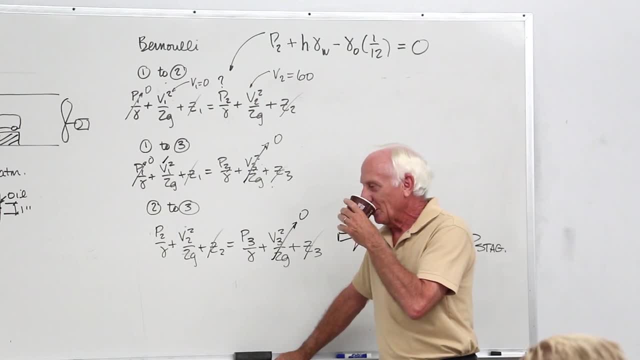 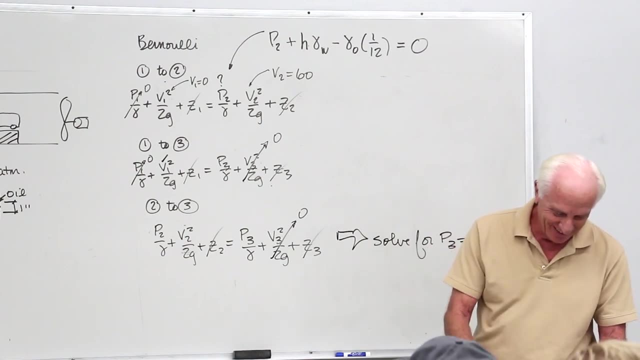 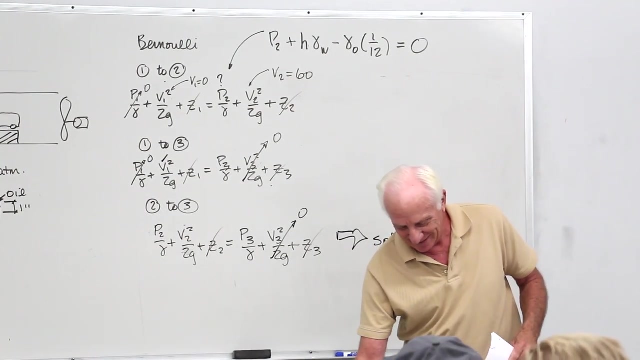 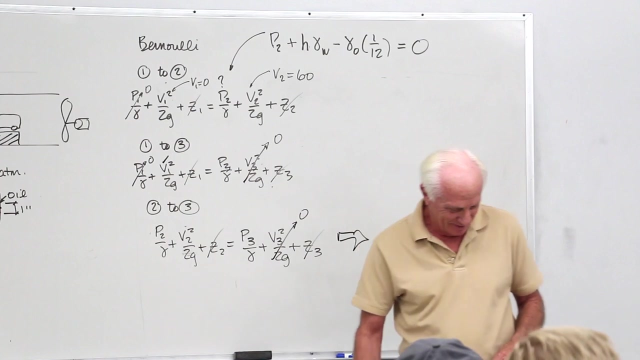 picture, just so you know for a moment. Okay, Now that takes care of all that homework. It's a long thing to go through, but I'm going to go through those, because chapter three is not easy. I understand that. Chapter four: well, we're in five now. Chapter 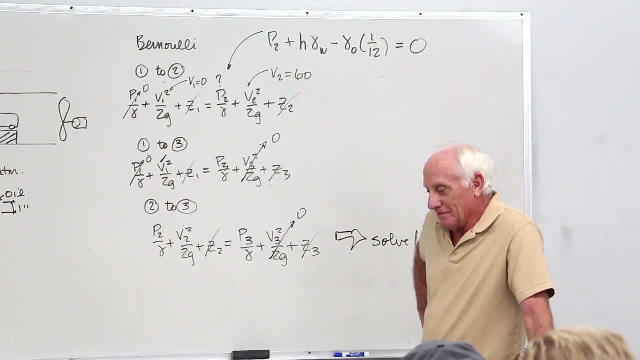 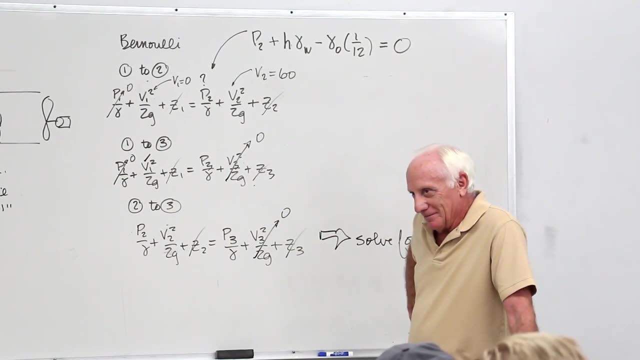 four. Chapter four is probably, in my mind, the hardest of the first four chapters. That was going through Reynolds, Transport Theorem and fluid acceleration normal to a stream line, a long stream line. Okay, So now we get into five, which is the application part. 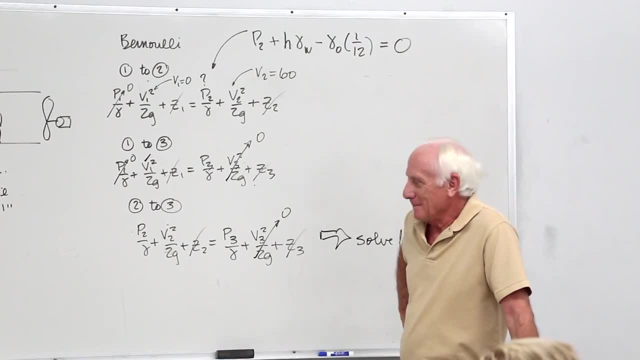 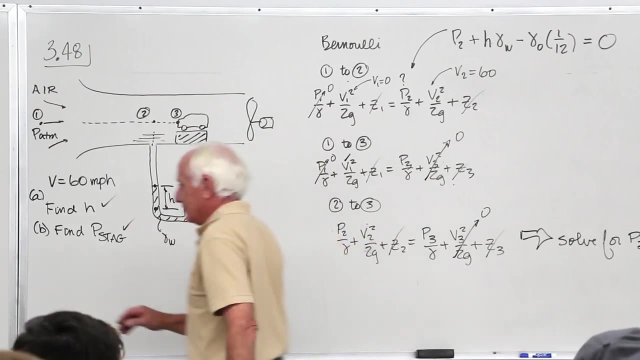 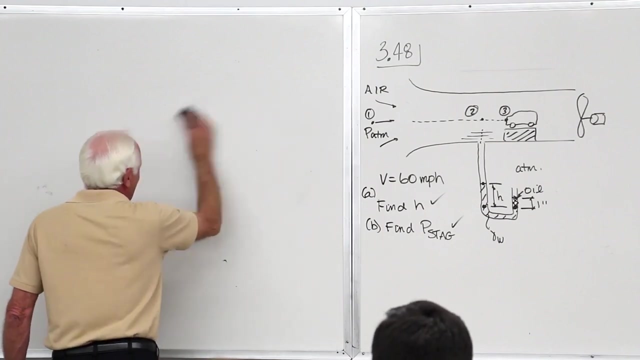 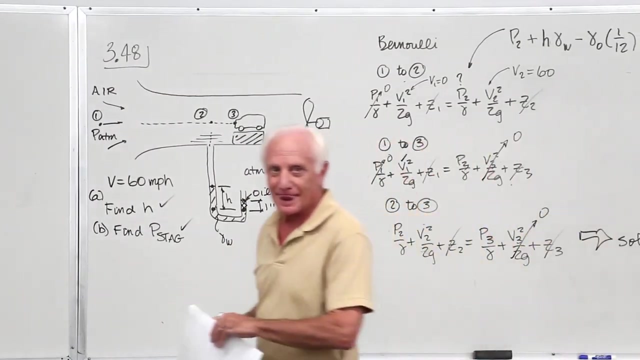 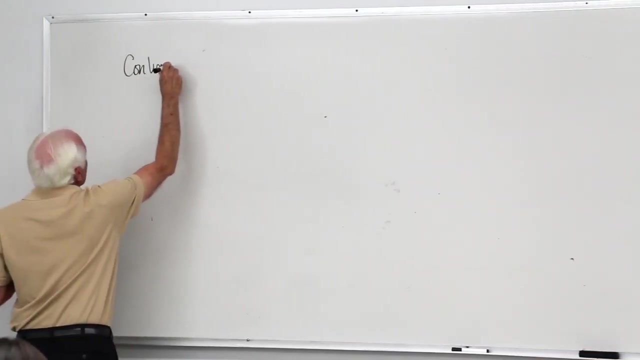 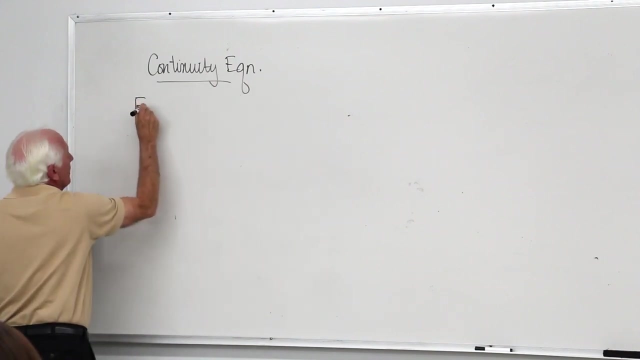 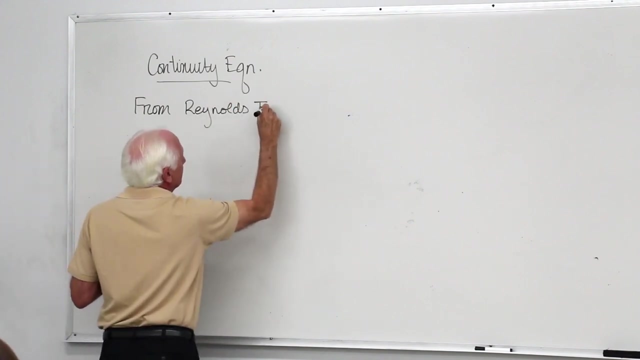 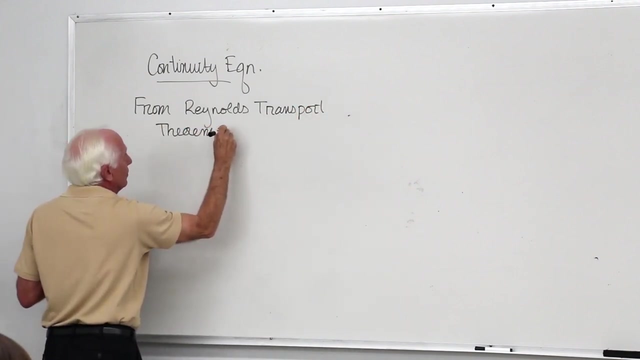 It's maybe what you might think of as the fun part. All right Continuity, All right Continuity played. It comes from Reynolds transport theorem with a value of B equal to the mass, So little b is then equal to big B over the mass, which is the mass over the mass which. 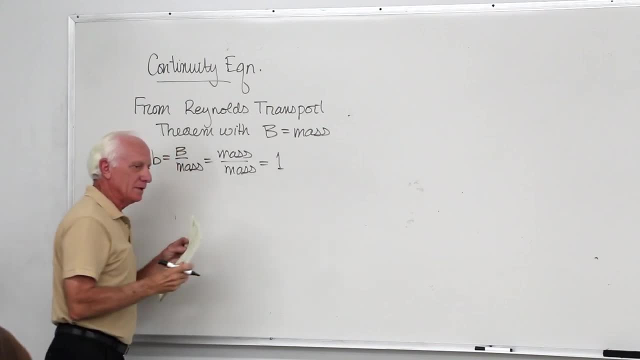 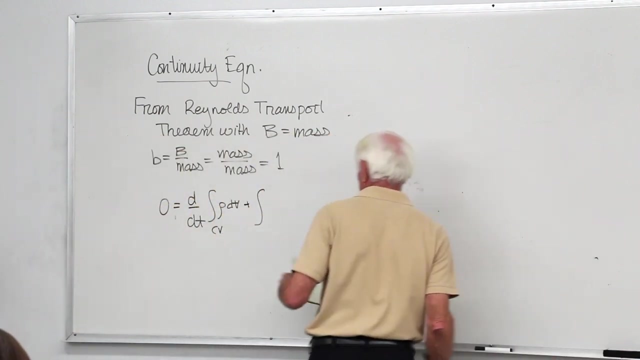 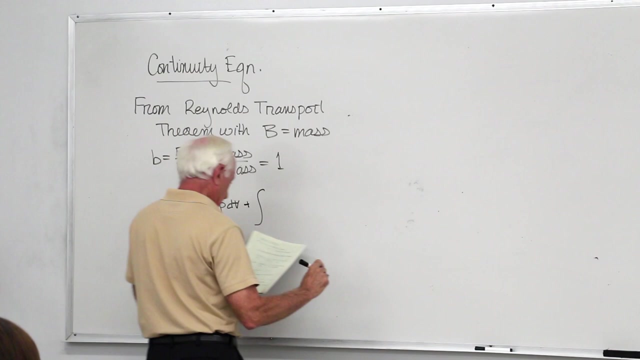 of course, is uniform. So everywhere in the Reynolds transport theorem, where we see a little b, we put a 1, and we end up with this equation. Okay, Let's well like. this is what I'm going to put it in terms of you know, for a flow. 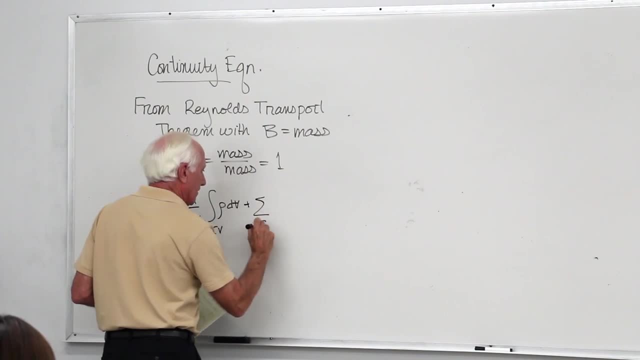 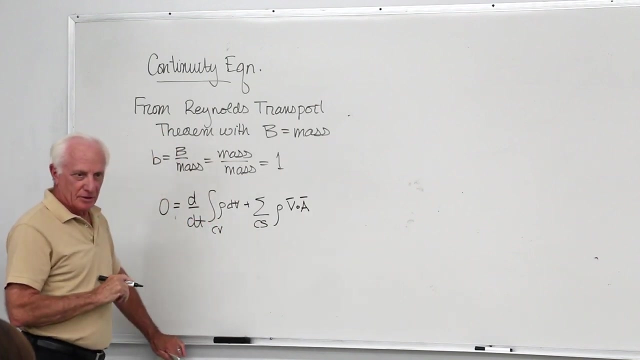 I guess simplifying for us a little bit, sorry. Remember, uniform flow is where the flow remains the same value across the cross-sectional area: uniform flow. So if you want to then put the terms around, that's essentially. that's essentially we. 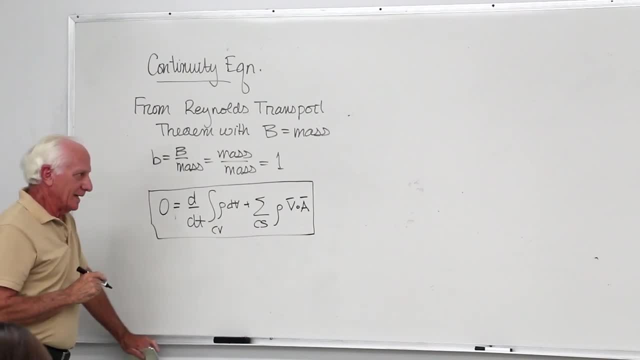 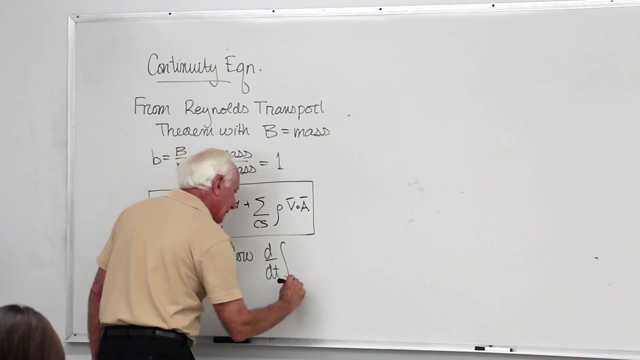 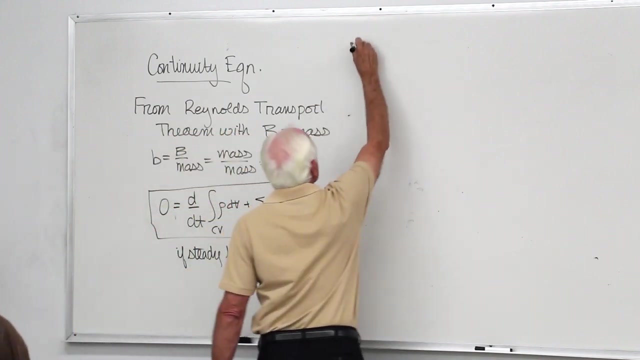 did this last time. Okay, We said: if steady, Okay, Okay. Okay, If steady flow d d t of anything, anything, including this thing, is zero, Okay, That term goes up. So if it's steady flow, then we have just this term left. 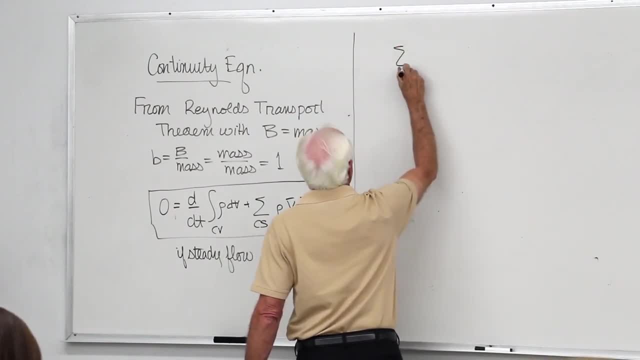 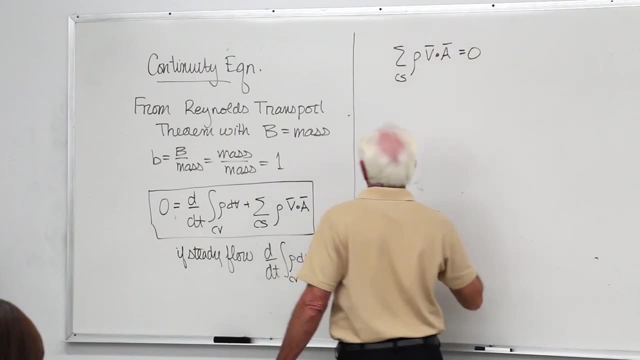 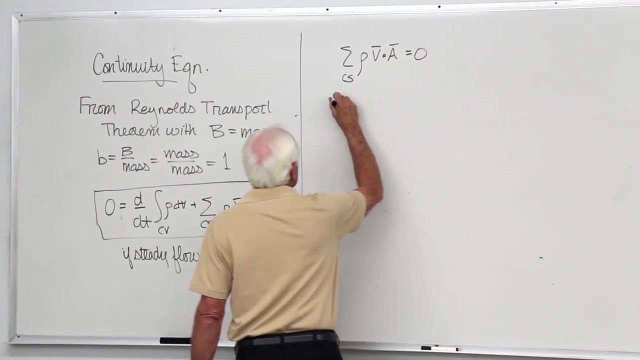 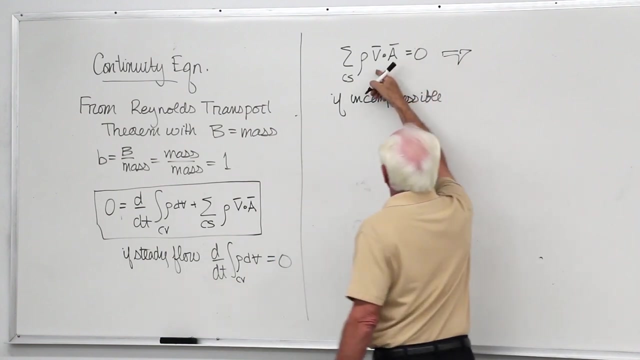 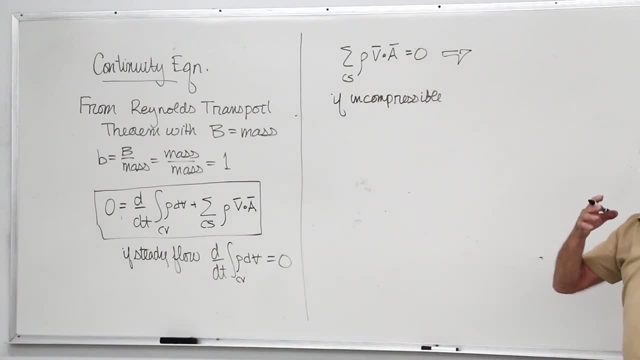 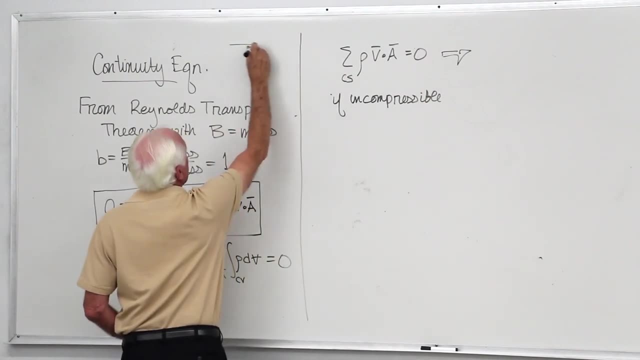 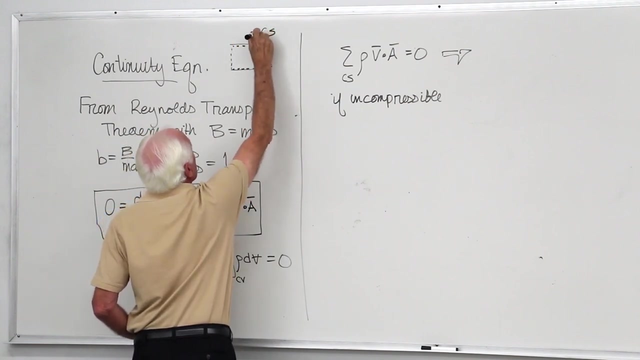 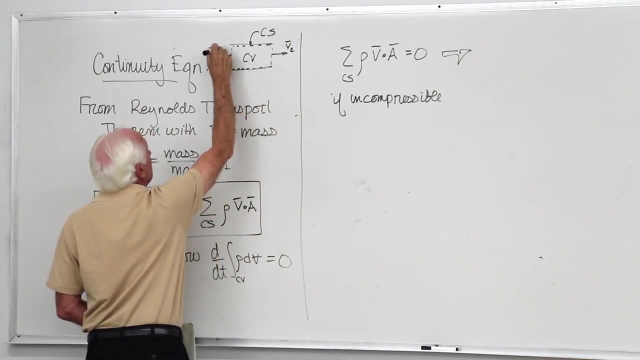 Velocity times area is Q, capital Q, the volumetric flow rate. So you remember the rule. The rule is- I'll do a very brief one here. Here's the control surface, Here's the control volume. If the velocity vector is going this way, V2,, this is V1.. 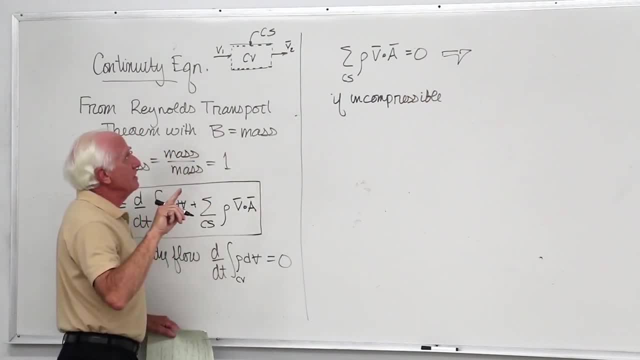 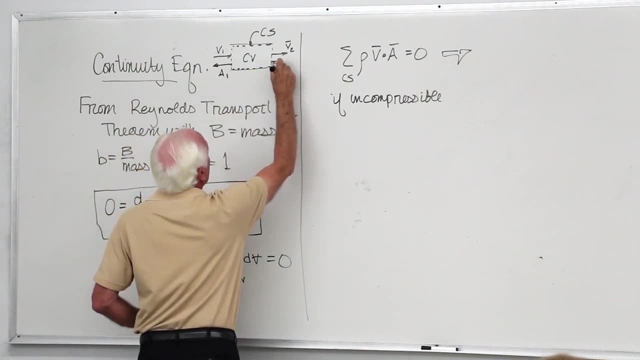 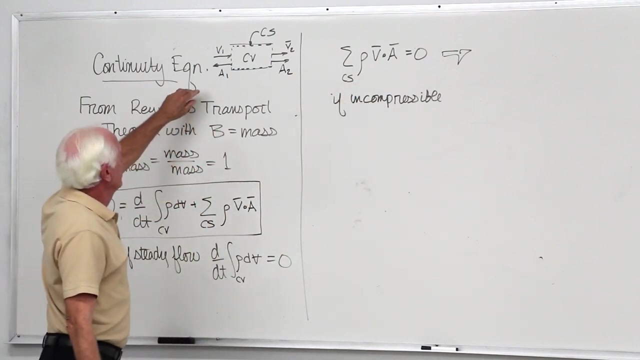 Now I draw the area vector. Don't forget the rule: The area vector always points outward from the control volume A1, A2.. You know the dot product, okay? So in this case let's take the easy case first. 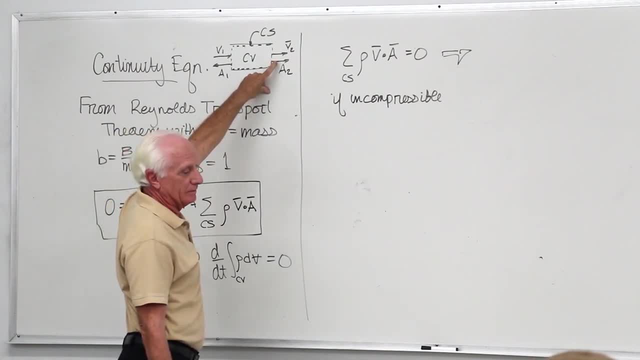 These two guys are in the same direction. in the same direction, okay. What's the angle between them? Zero, They're in the same direction. They're coincident, They're collinear Zero. What's the cosine of zero? 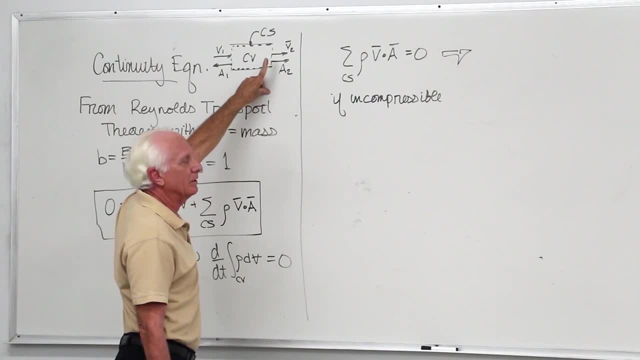 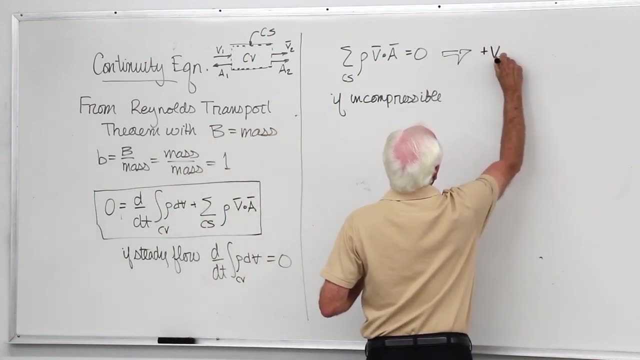 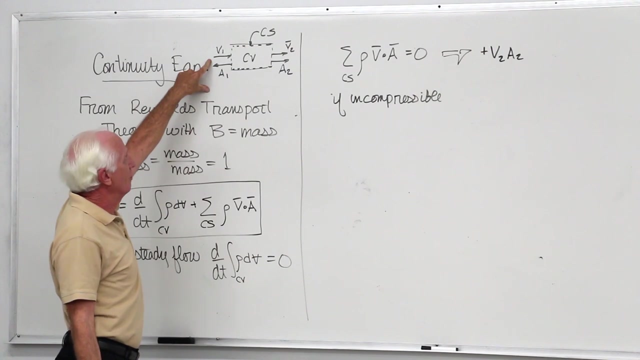 One Plus or minus Plus one. Okay, That's going out V2, A2, plus Coming in. V1 is going in the control volume, The angle between them. Well, here's the picture: V1, A1.. 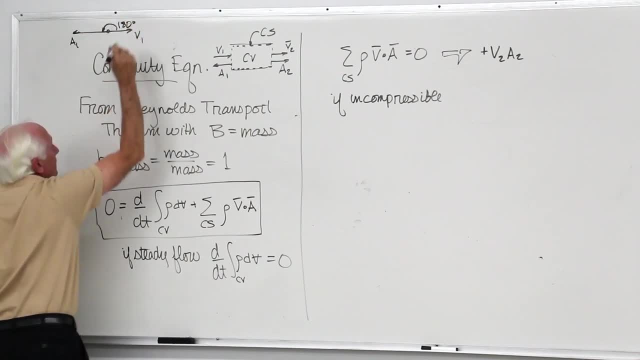 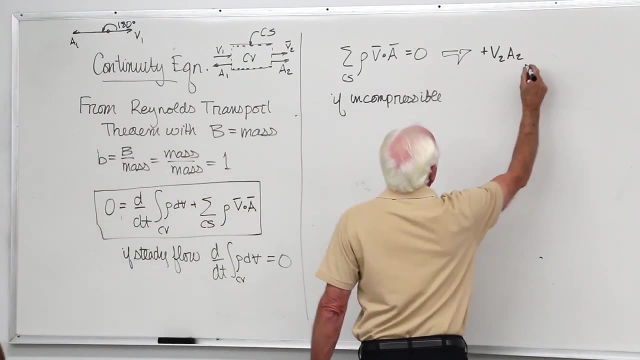 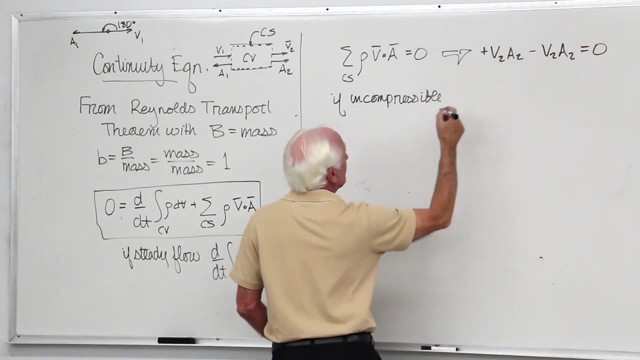 The angle between them: 180 degrees, Cosine, Cosine, 180.. Here it comes. Minus one, Minus one, Okay. minus V2, A2 equals zero. Now, if you want to leave row in there, okay. 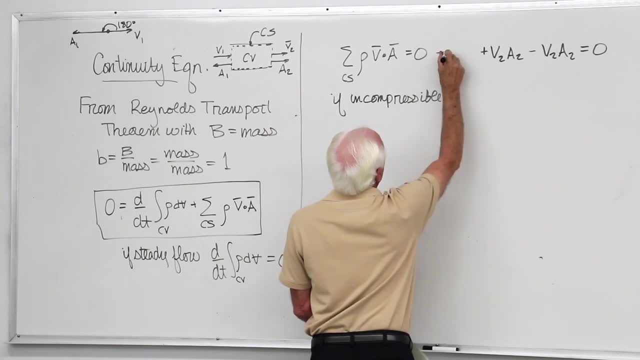 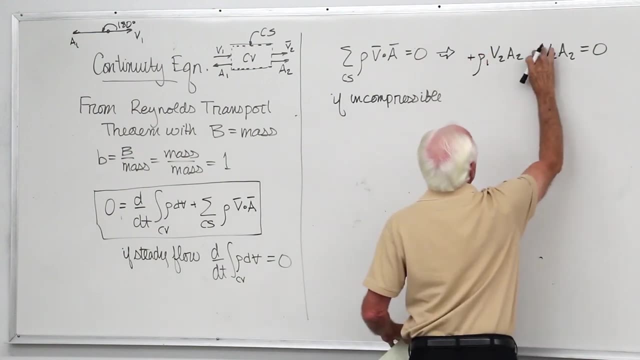 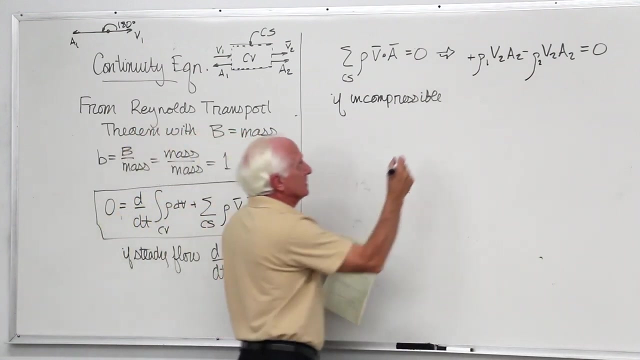 Leave row in there, just to be general. Leave row in here. Okay, Now you say if incompressible, incompressible means row one equals row two. So then we have V2, A2 equals V1, A1, which means Q2 equals Q1.. 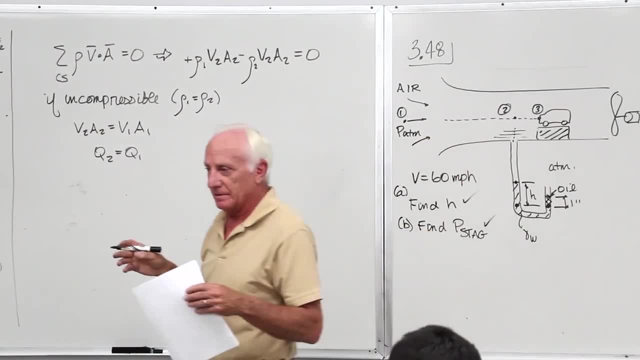 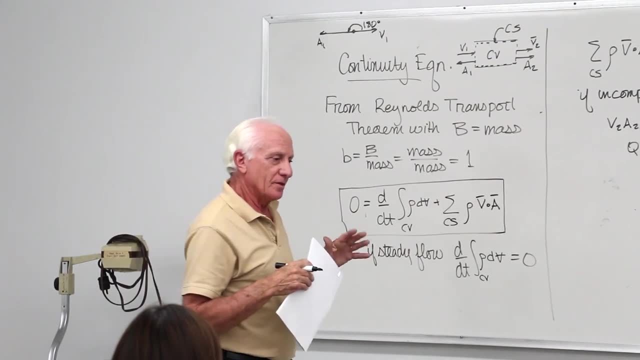 For instance, if we have 50 gallons per minute coming in, we have 50 gallons per minute leaving. If we have 1,000 liters per second coming in, there's 1,000 liters per second going out. Volumetric flow rate. 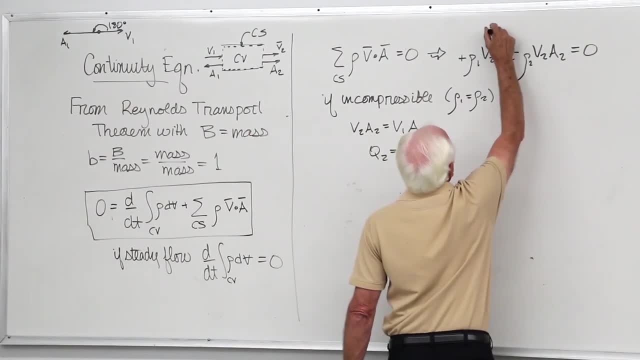 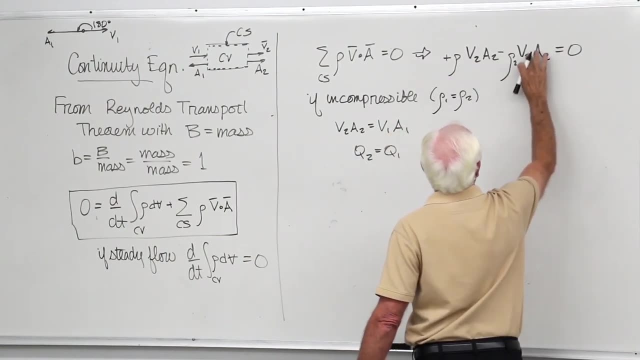 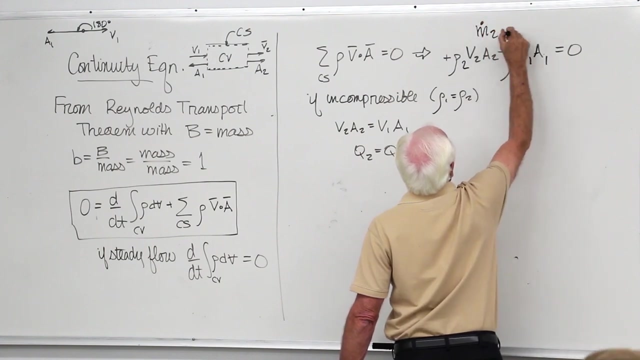 This one up here, of course, is m dot. This should be. oh, this is, how do I get that? Okay, This was my outflow, my inflow, excuse me. M dot 2 equals m dot 1.. 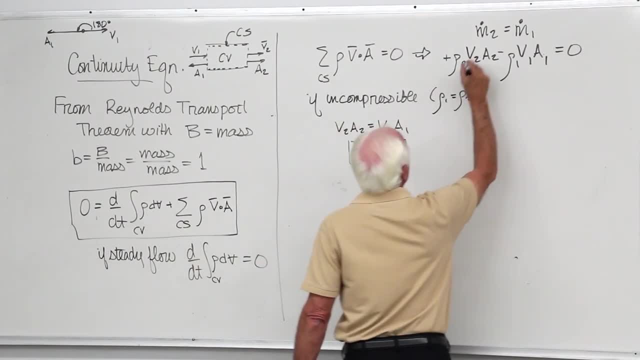 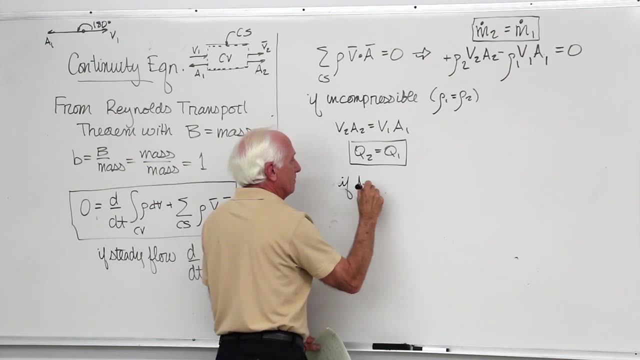 And last time we talked we bought all these guys in. We bought all these guys in, And then we talked about this And then we said if the areas are the same, A1 equals A2, then V1 equals V2.. 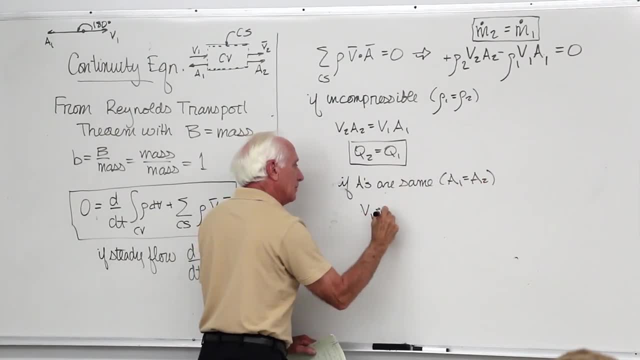 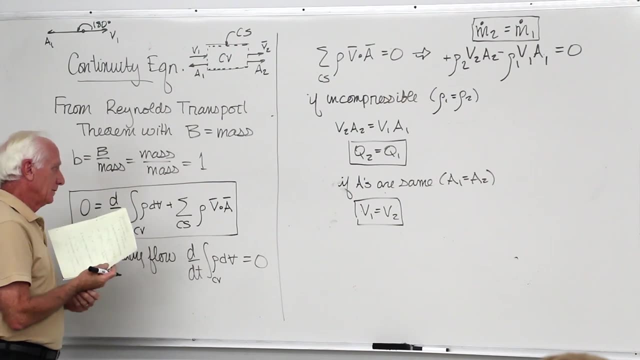 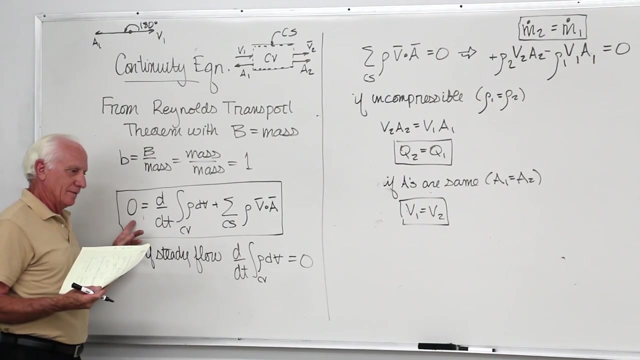 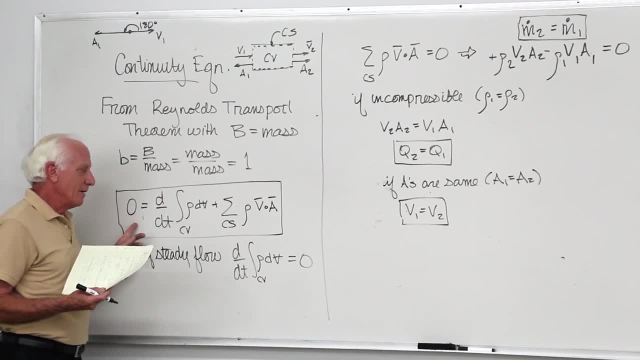 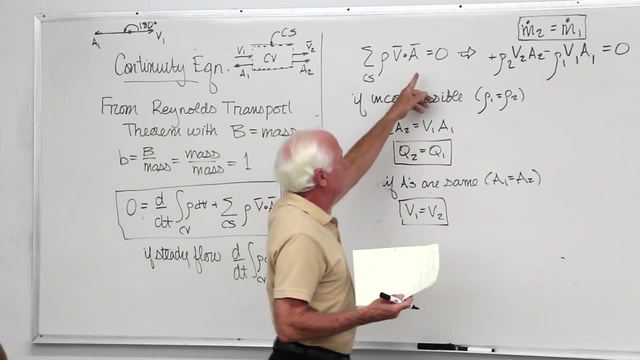 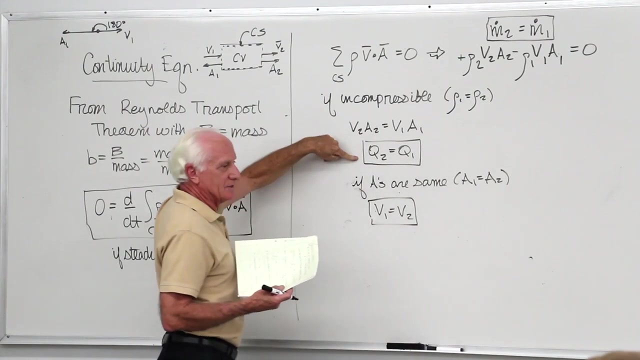 Okay, Mass could be accumulated in a storage container, But if it is steady-state, if it's steady-state or steady-flow, then that term goes to zero. Okay, I got this guy. This guy applies when steady-flow. Okay, This guy applies when steady-flow and incompressible. 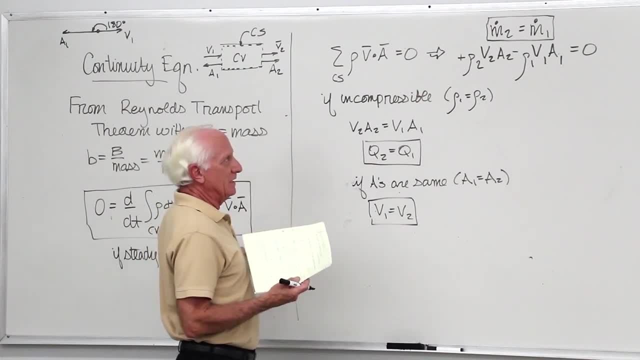 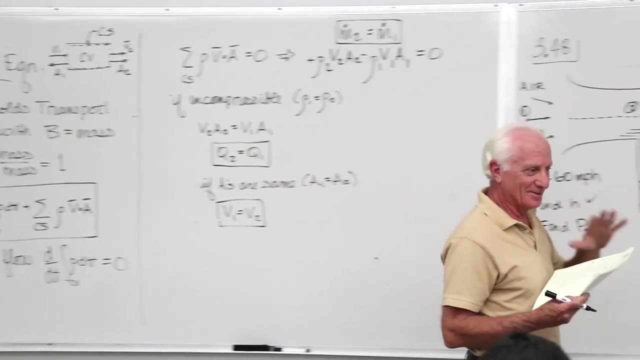 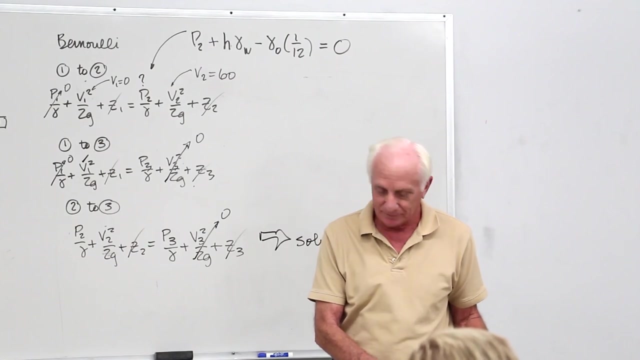 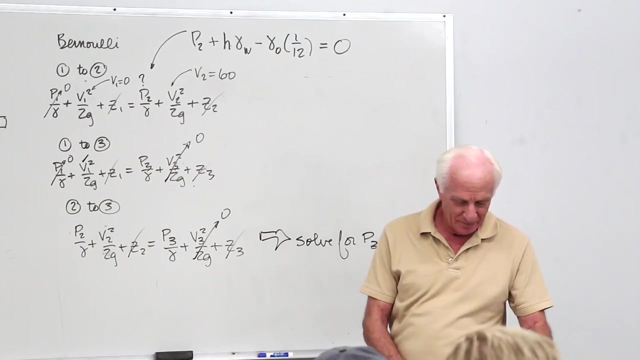 This guy applies when steady-flow, incompressible and area's the same. So each one has a certain limitation built into it. Okay, so we're going to use those in examples. Let's see which one we'll take first. Let's do this one first, Okay. 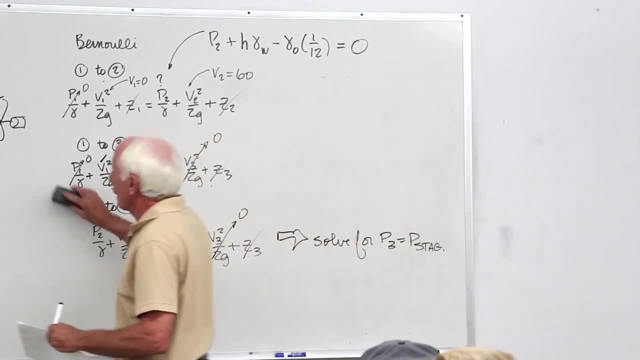 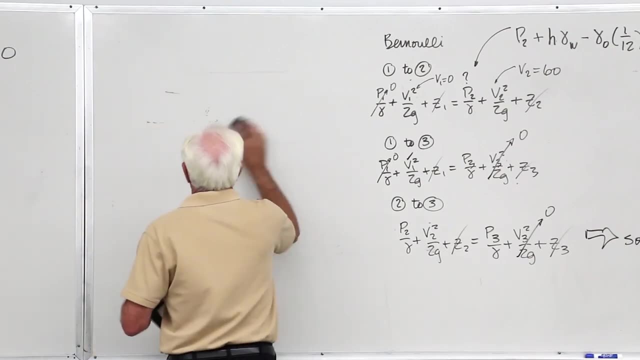 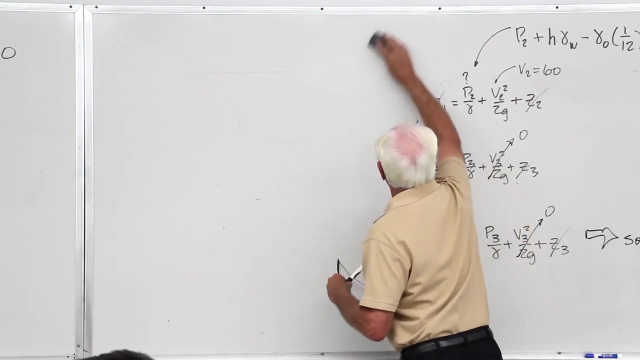 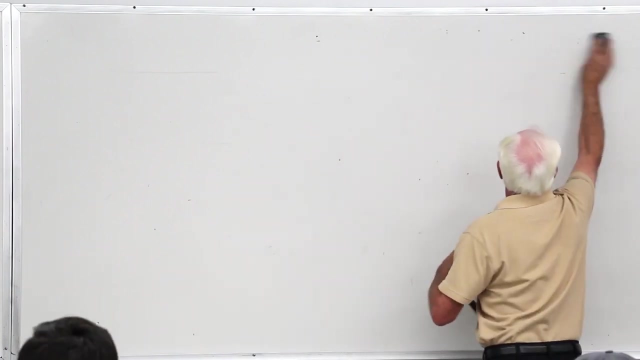 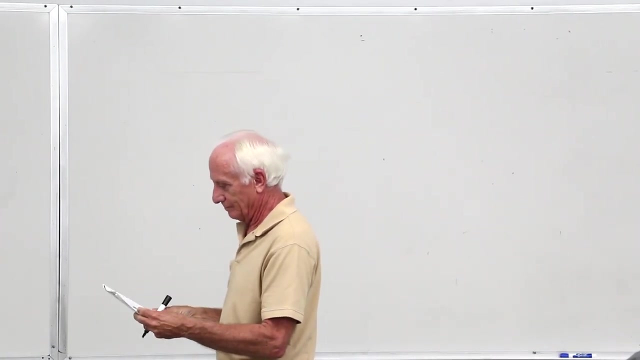 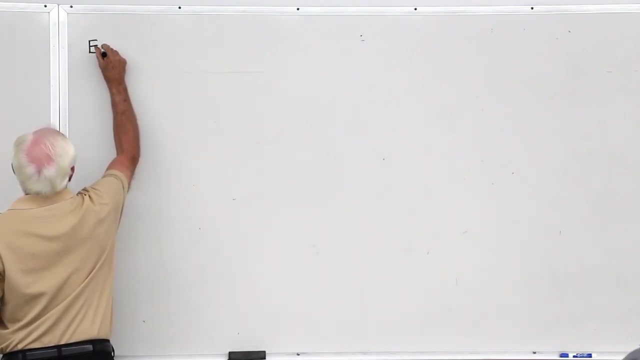 let's make some room over here. We're going to work a problem that we'll start simple and get to more complex. We'll end up with a non-steady flow problem. We'll start simple. Okay, Let's see, This is not in your textbook, It's an example. We have some kind of 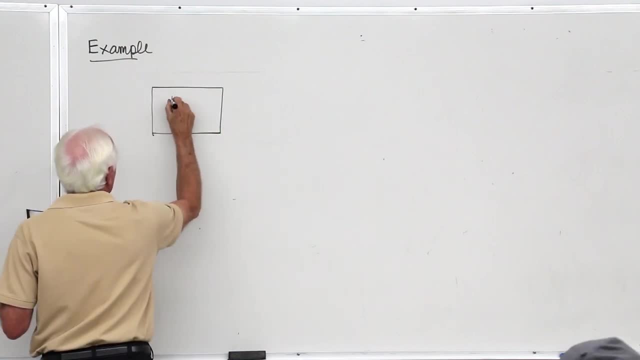 flow device. We don't know what it is. It might be a mixing chamber or something. We have flow coming in, We have flow going out the right side And we have flow going out the bottom. Okay, We're given it's water, We're given the pipe size is three inches. 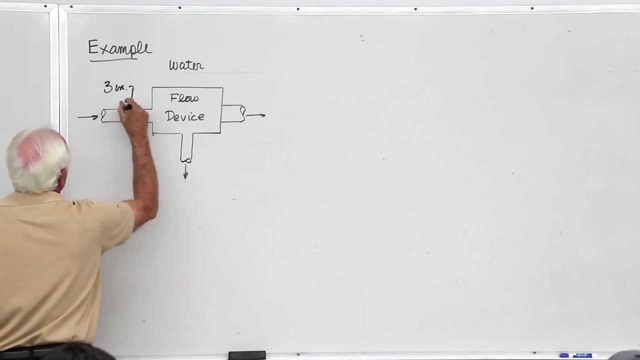 Okay, Okay, Four inch diameter. Four inch diameter, Two inch diameter. We're given the velocity coming in the left: 30 feet per second. We're given the flow rate going out the right: three-tenths cubic feet per second. Okay, 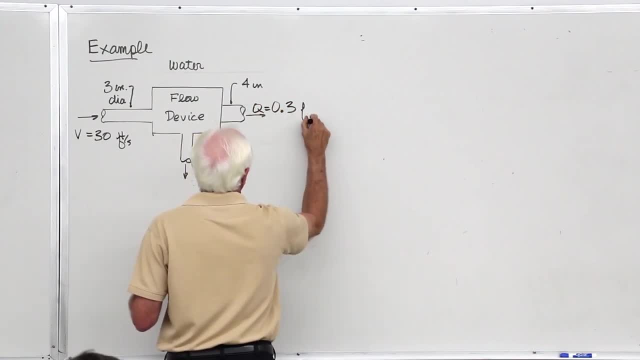 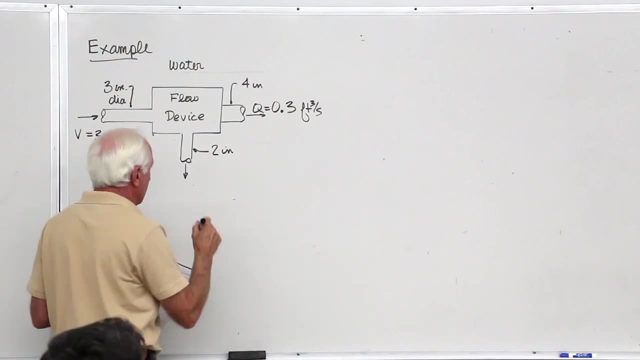 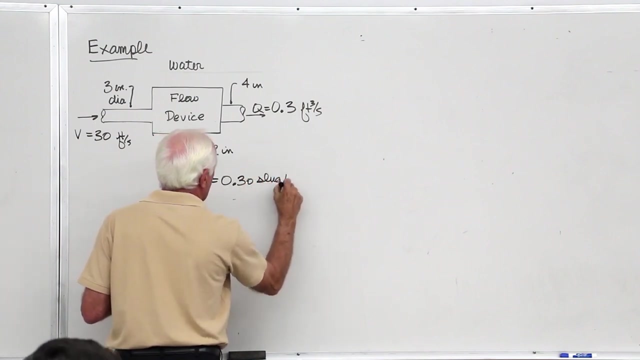 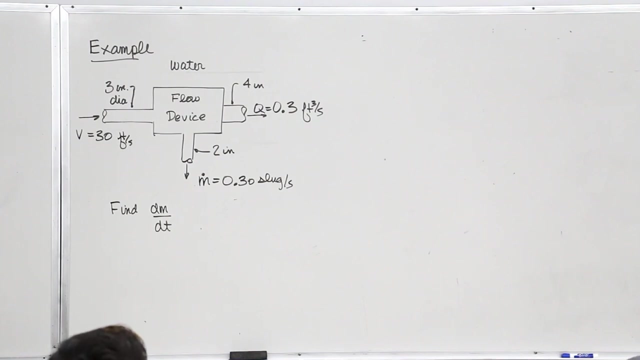 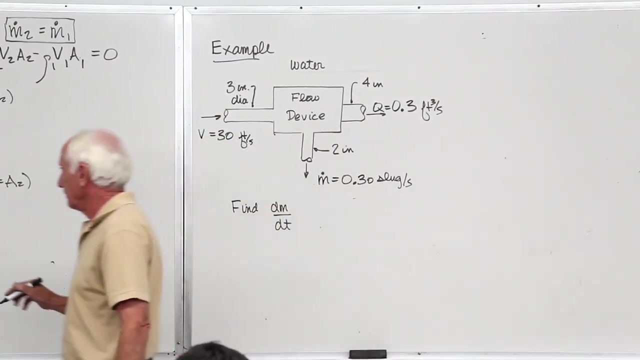 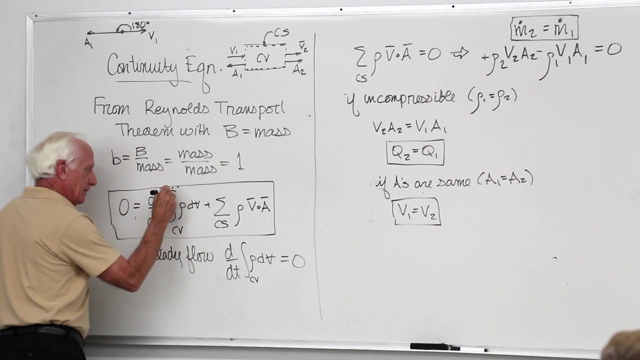 Slowly to the bottom. We're given three-tenths slug per second. We want to know the rate of change of the mass of water in the device. Okay, Okay, So this is a non-steady flow problem. Okay, so, here it is right here. There it is right there. That's M This thing, right. 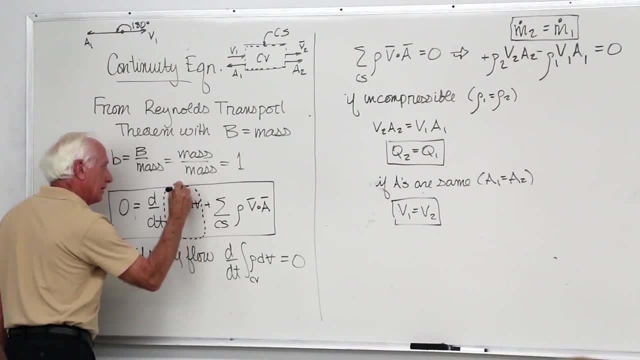 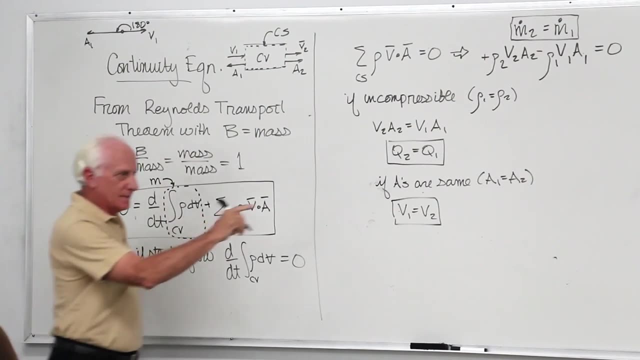 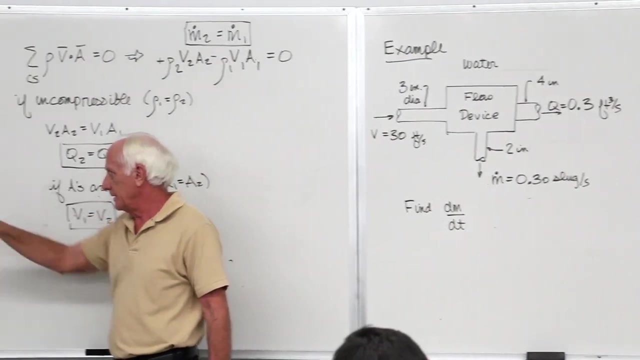 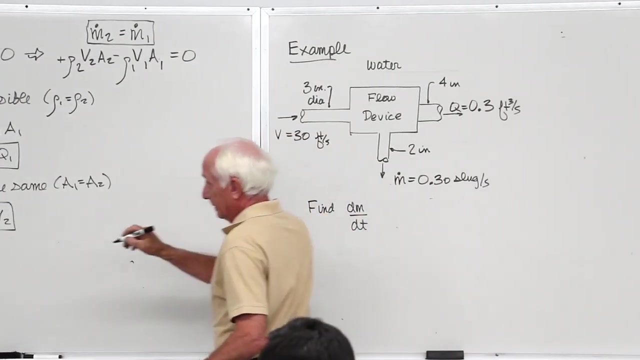 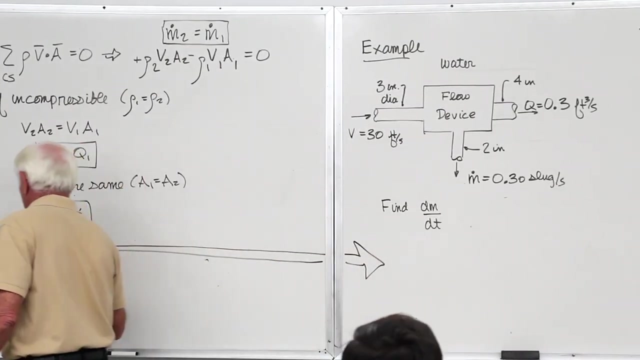 here in the dashed line is the mass of what's in the control volume. That's what he asked us to find. Find dM by dt, Find that guy. So there he is. Let's take this. I'll just put a big line here. I'm going to take that and I'm going to put that guy right there, Zero. 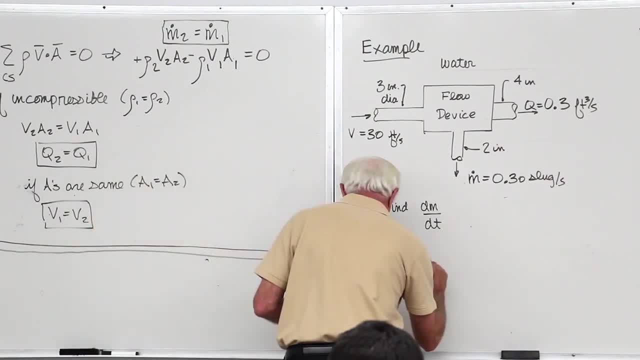 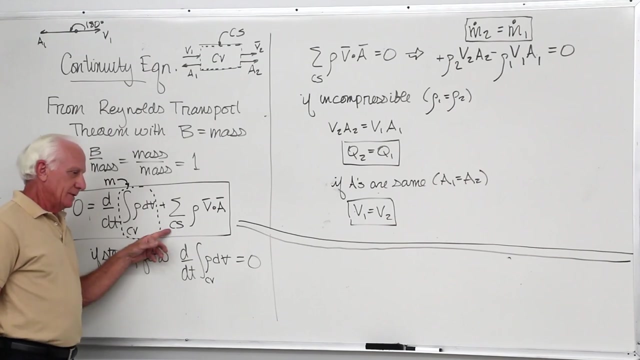 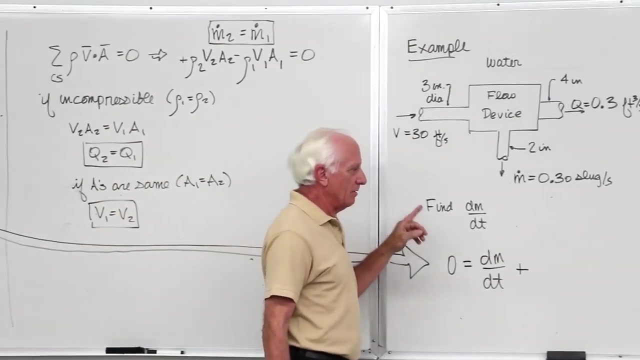 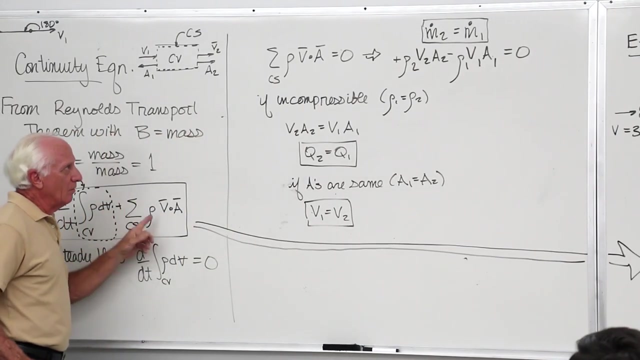 equal dM by dt. Okay, plus what's the summation mean? It means go around the control surface. This summation over the control surface means go around the control surface. Wherever you see fluid entering or leaving, stop and do what it says here. Now we know from here. 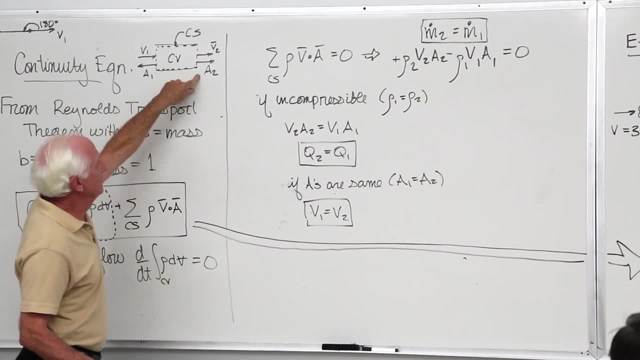 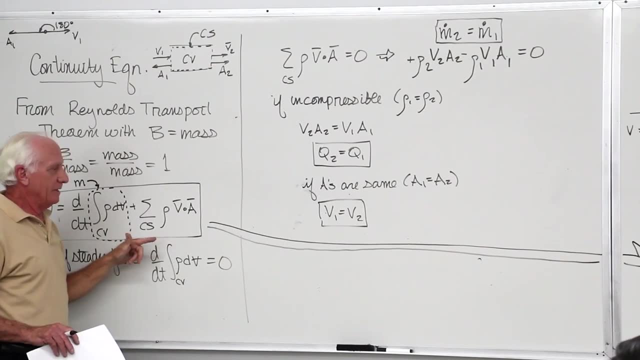 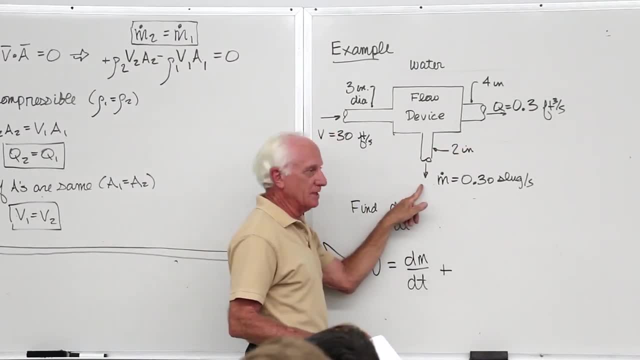 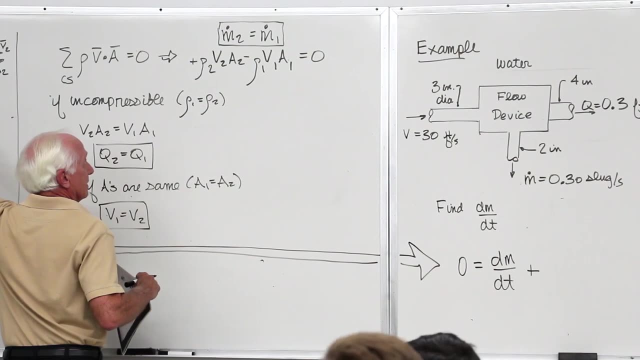 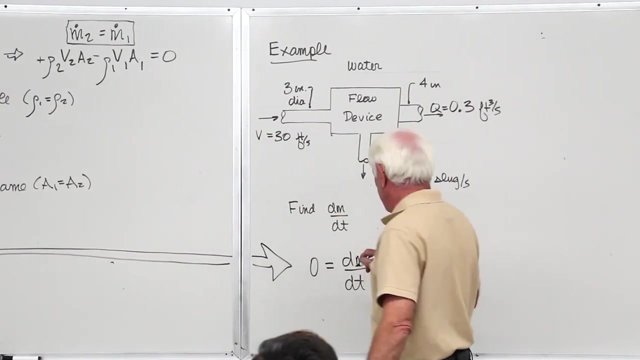 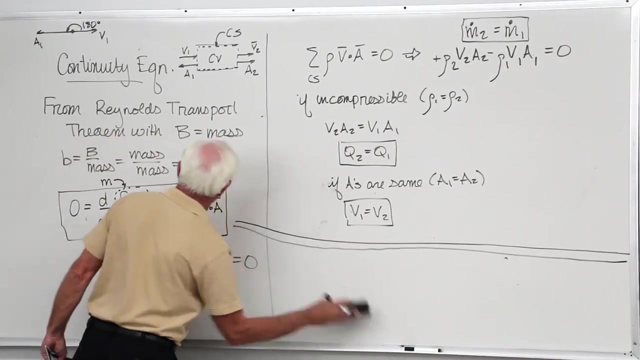 If it goes out, it's positive. If it goes out, it's positive. If it comes in, it's negative. because of that picture right there. B dot A is negative. Cosine of one, A minus one, Okay, going out. Every term in the equation has to have these dimensions Row: this is: 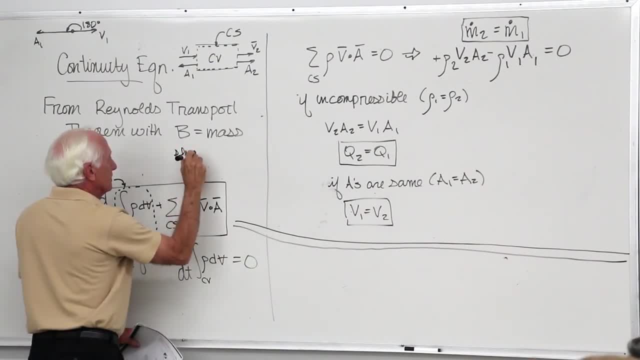 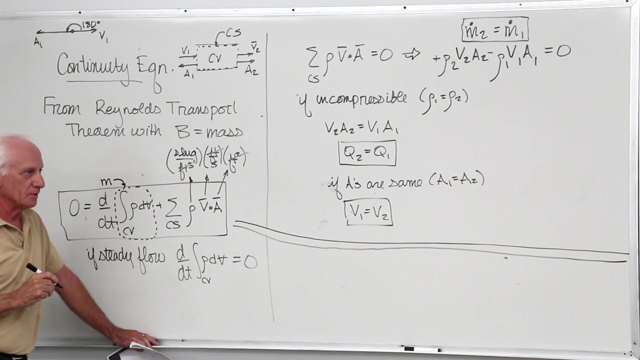 in English: Row slugs per cubic foot. Velocity feet per second Area. cubic square feet. Cancel, cancel, cancel, Yep, Every term in that equation is a mass flow rate term Slugs per second. Slugs per second. Ah, look at that. Thank you very much. 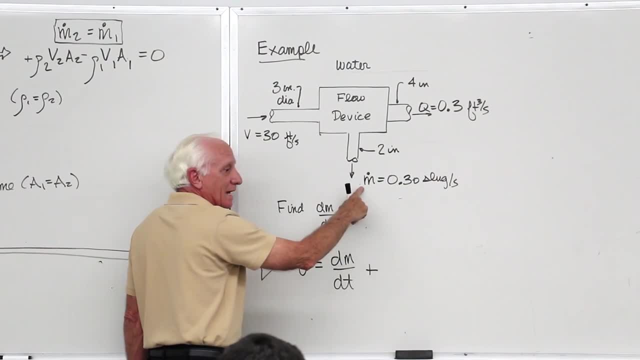 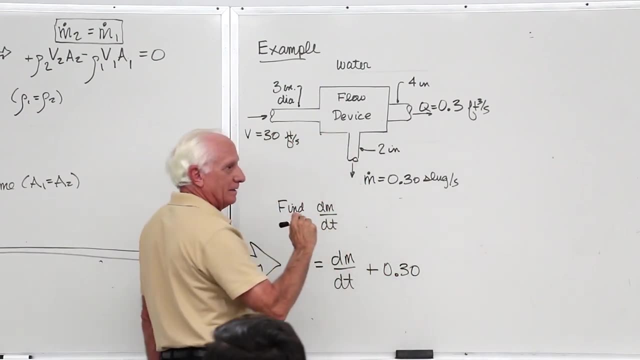 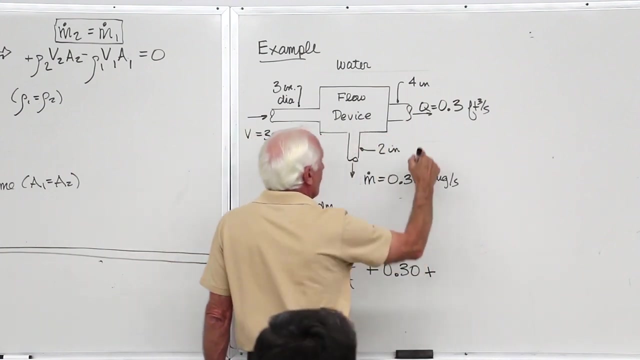 He gave me that one. It's going out. It's positive, Positive 0.30.. Keep going. The right hand side is going out Positive. What do you give me? Q? What do I want? M dot, How? 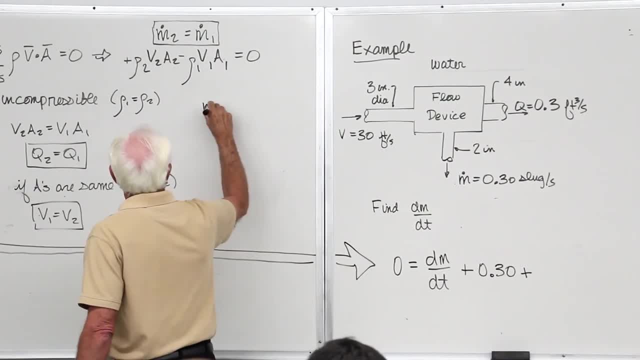 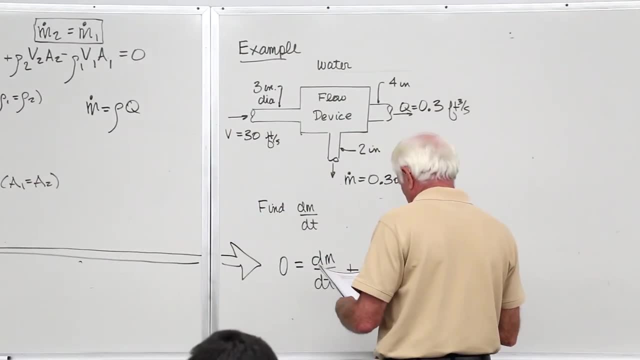 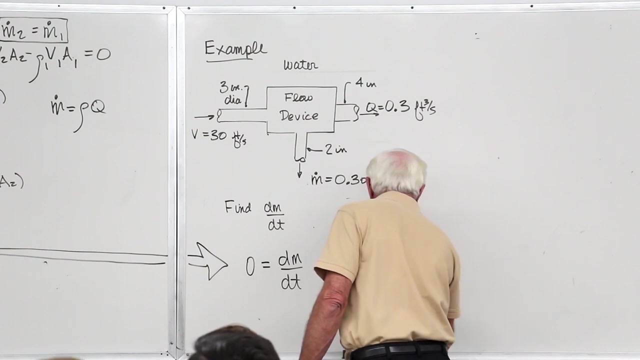 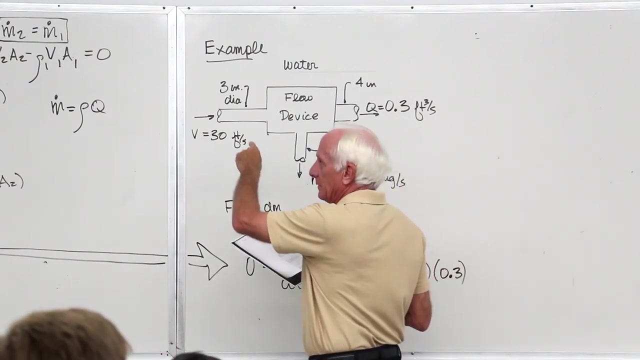 are they related? M dot equal row Q: Okay, Our row. let's see, There's our row. 1.94 slugs, 1.94 slugs per cubic foot Times: Q: 0.3.. Last one Flow comes in the left. He gave me velocity, Okay, So I'm going to. 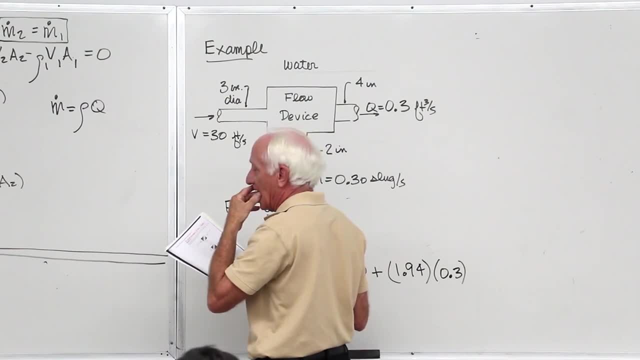 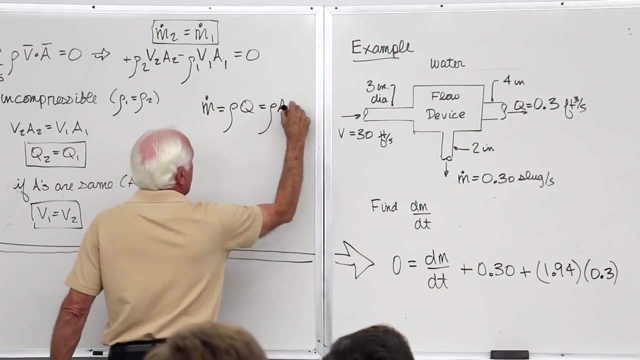 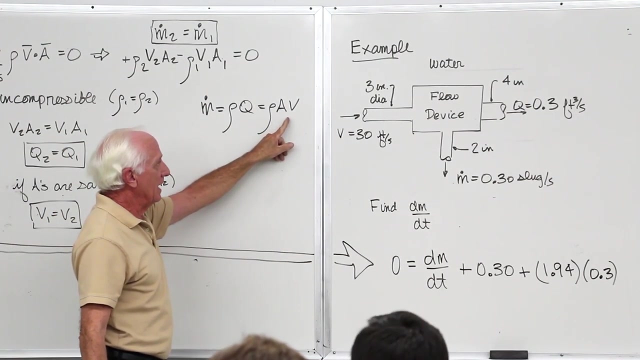 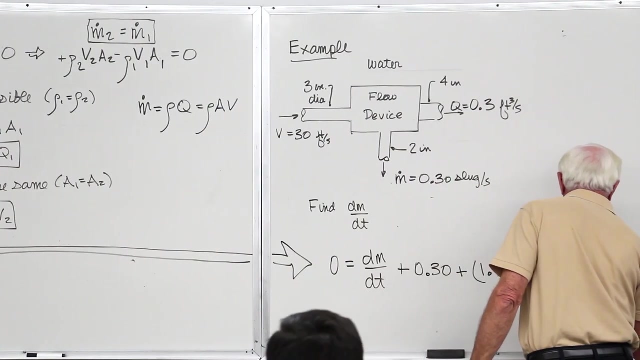 masse it up a little bit. I want a mass flowing There. it is M dot and row A V. I know row I can find A. He gave me V. okay, Row 1.94 slugs per cubic foot. 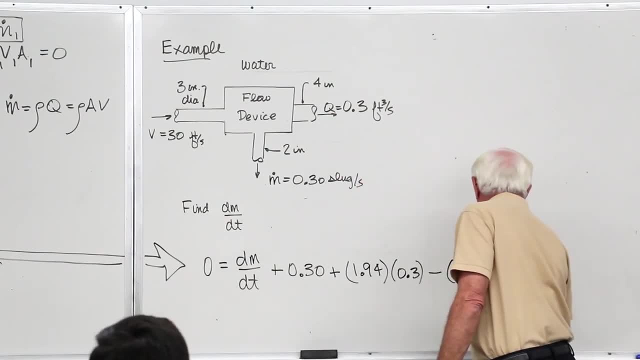 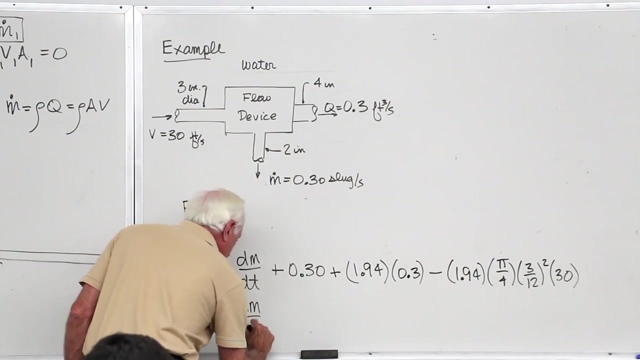 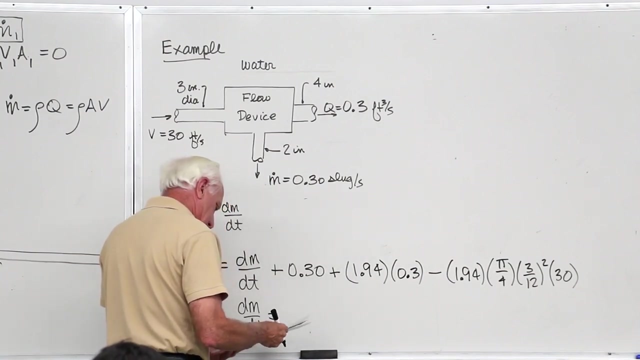 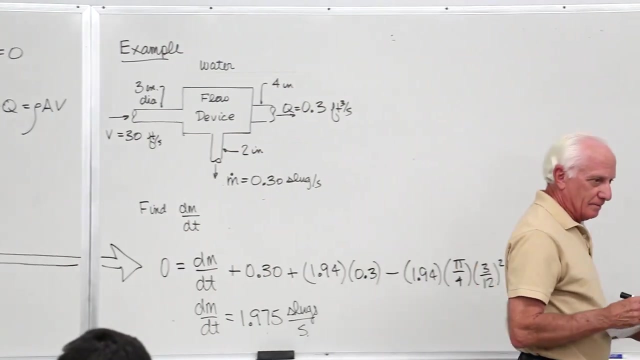 circular pipe 3 inch diameter. pi over 4, 3 twelfths squared, Times the velocity 30 feet per second, Solve for the MVT 1.975.. Yeah, 1.975 slugs per second. So deliberately. 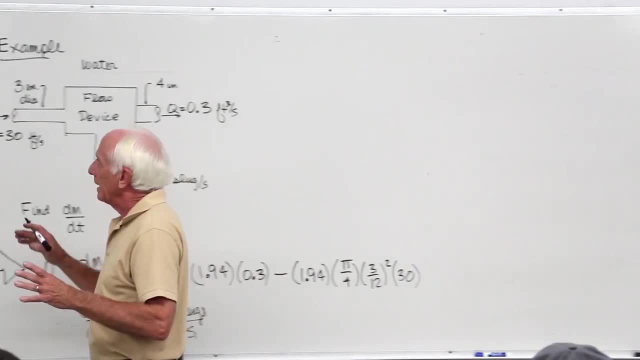 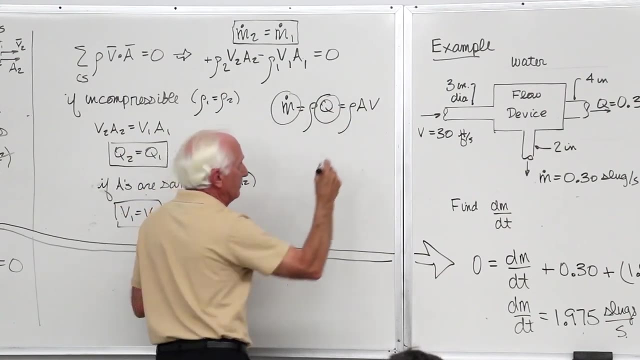 I gave you 3 pipes per second, 3 different quantities. I gave you a mass flow rate, I gave you a Q and I gave you a B to show you how to handle each one of those 3 quantities, Because you can expect. 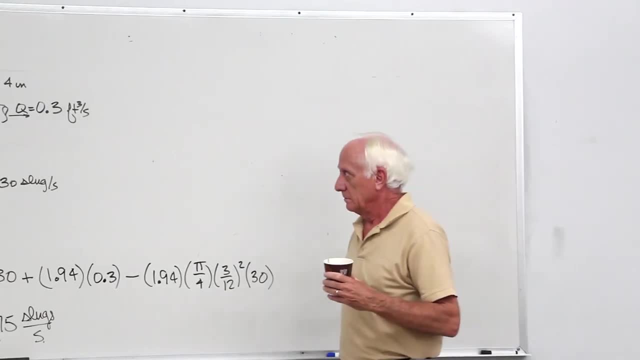 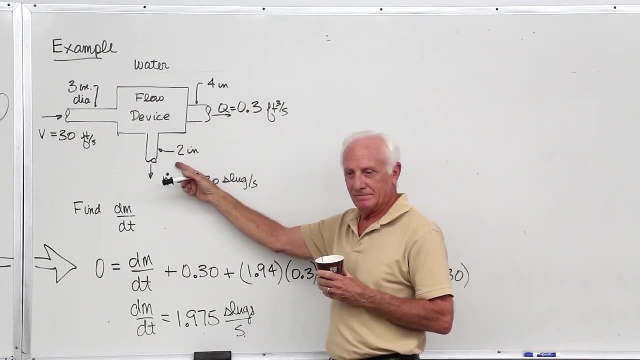 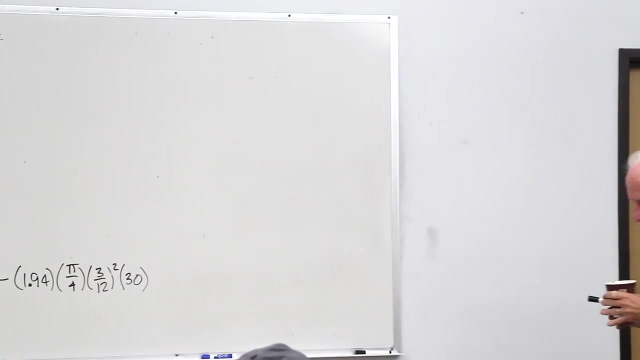 anyone of those 3, somebody to give you. Did I need the 4 inch pipe size? Nope. Did I need the 2 inch pipe size? Nope. Did I need the 3 inch pipe size? Yep. So you don't need the other part of that, it doesn't matter. 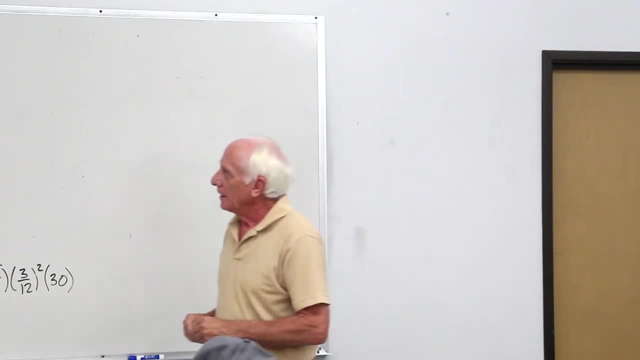 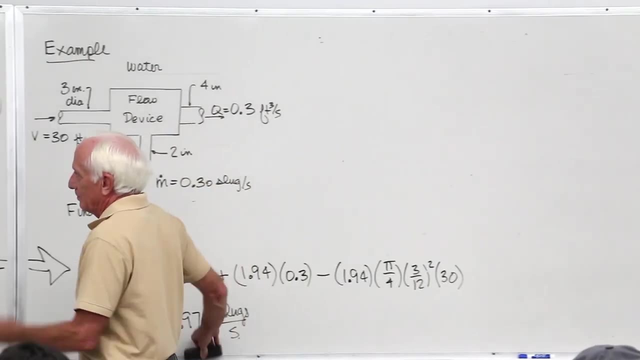 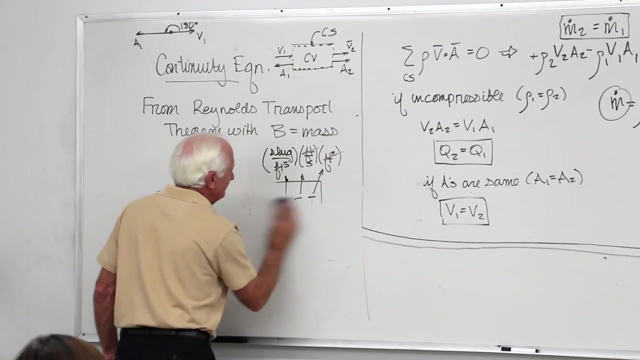 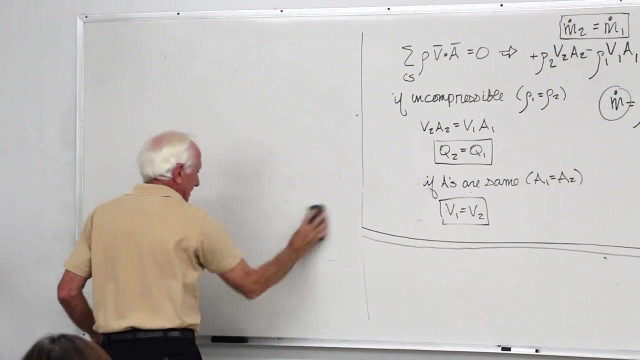 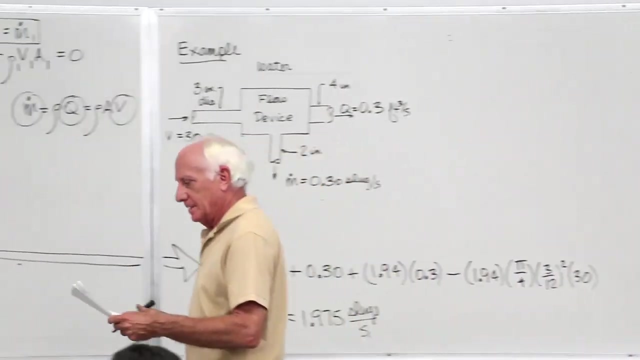 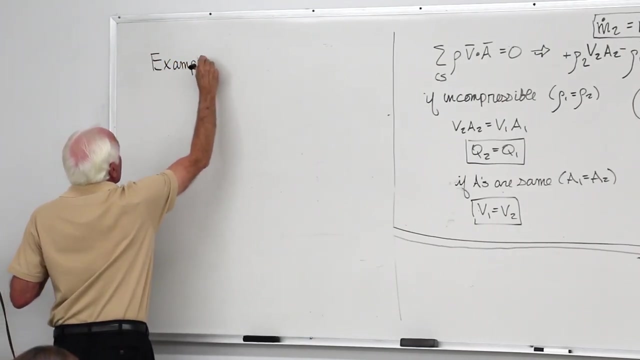 Okay, let's do another one. Let's see here. I'll put that in the middle panel now I'll put it over here. Okay, This particular one, I think this one, So it's not the book example- Okay, we have some kind of a storage device. 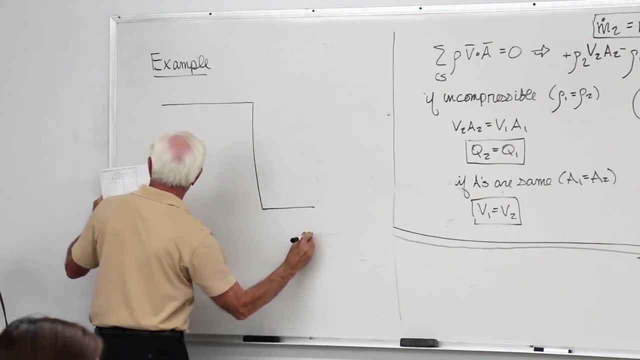 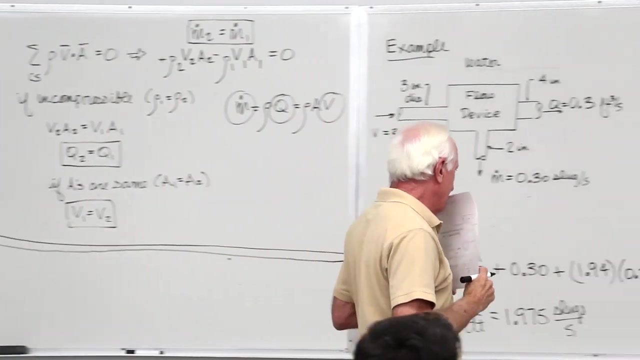 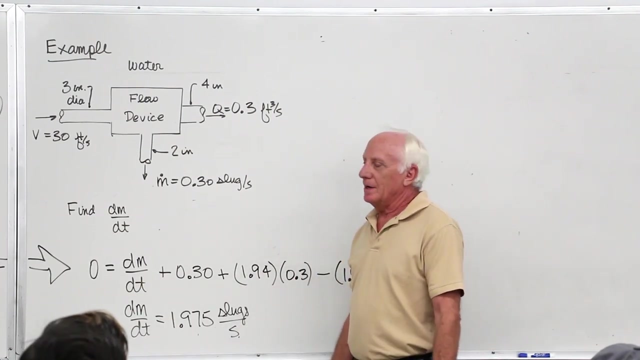 Where fluid comes in and goes up. yeah, What, conceptually, does the DMDT actually do to affect the problem? Because it looks like everything is accounted for. I don't see what it's doing, What this is. Yeah, Well, we'll come to an example later on. 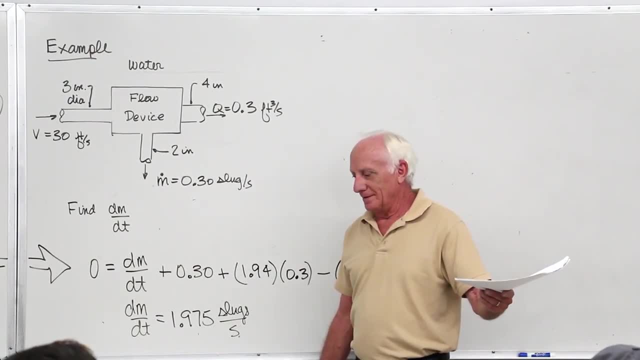 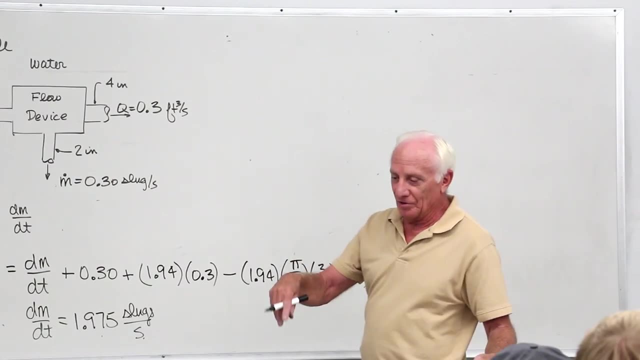 Okay, But let's say for right now, you put a piece of plywood over your tub in the bathroom And you drill a hole in it where the water comes in And you turn the bathtub water over And then there's a drain hole in the bottom. 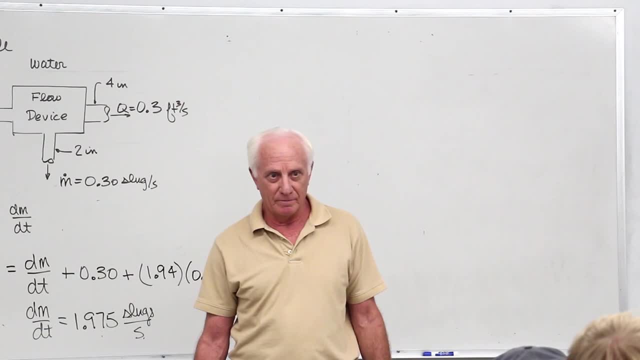 Is it going to fill? Is it going to drain Or stay the same? A hole in the bottom of the bathtub, Yeah. or the drain? Yeah, shower water goes out. I guess you'd have to figure that out. Guess what I just did. 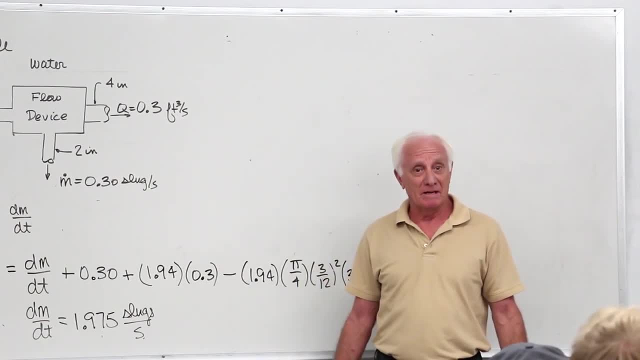 Okay, I figured it out, didn't I? And what'd I say? There's getting more and more mass in that bathtub. How much more mass? 1.7, 1.975 slugs per second, Yeah, Yeah. 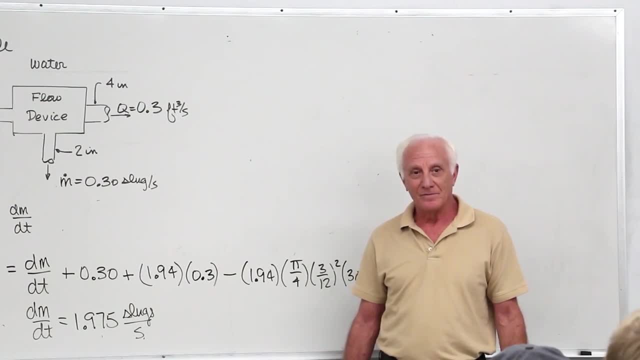 So basically, what's happening here is there's a certain volume flowing in and then there are two volumes flowing out. That's right, And you need to figure out whether- Yeah, We don't know the water level in here. We don't know the water level. 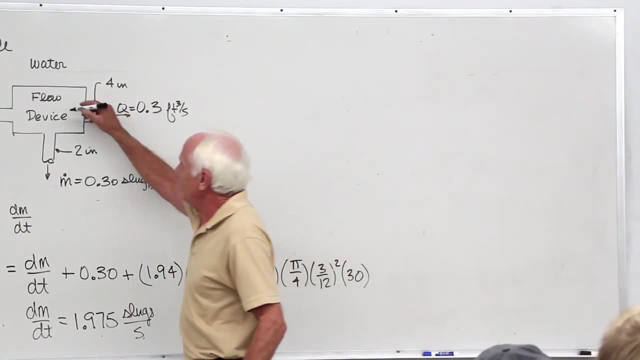 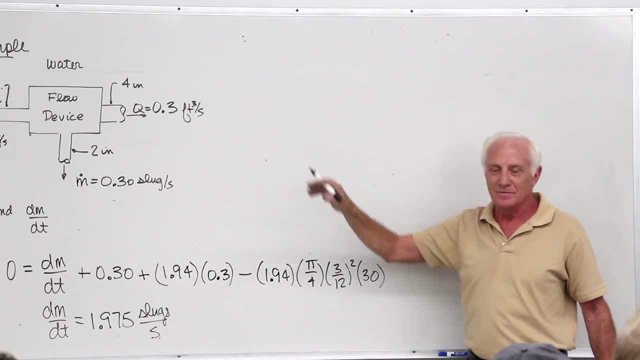 Water starts to go in. guess what Water won't go out for a while. After a while, what happens? The sponge gets real wet. Water starts going out. Is there more mass stored in this with time? Oh yeah, The sponge is heavier and heavier. 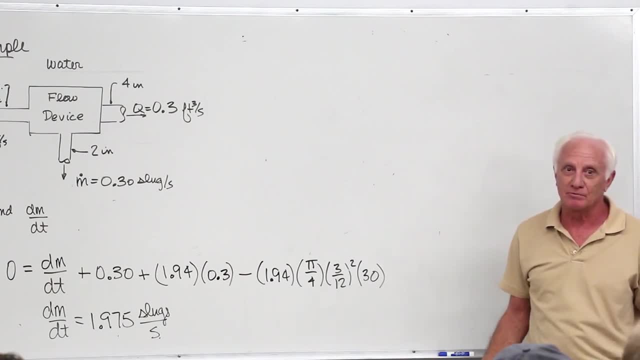 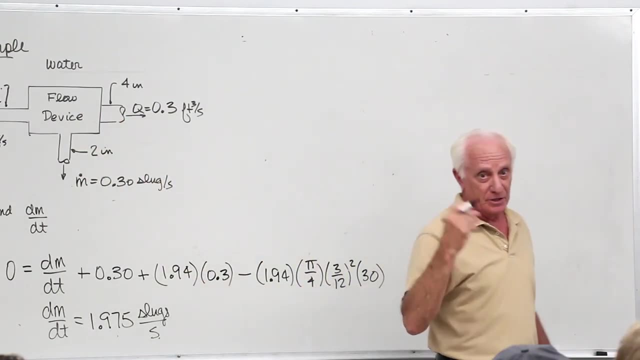 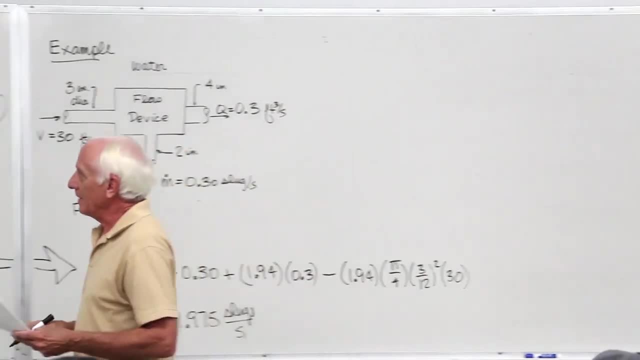 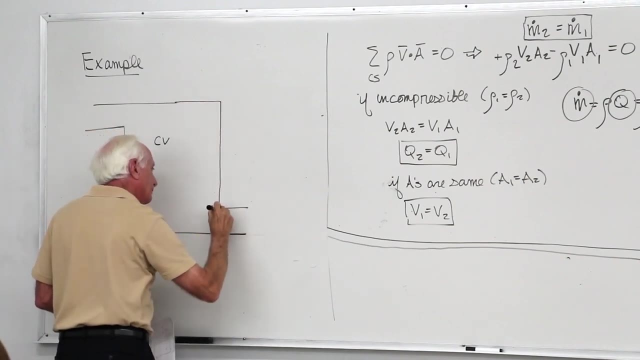 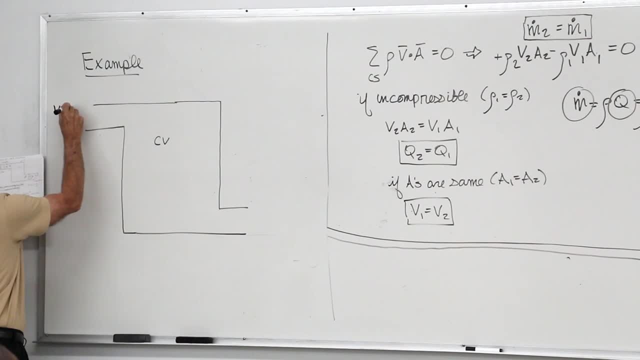 You're not. Well, I appreciate the input. It's really good. Well, All right, Okay, Thank you. Thank you all for steaming up, Okay. Okay, of water goes out here. Let me just change the slide for a second. The other side, Okay. 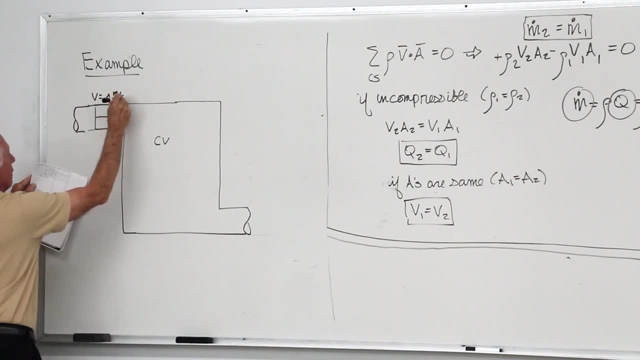 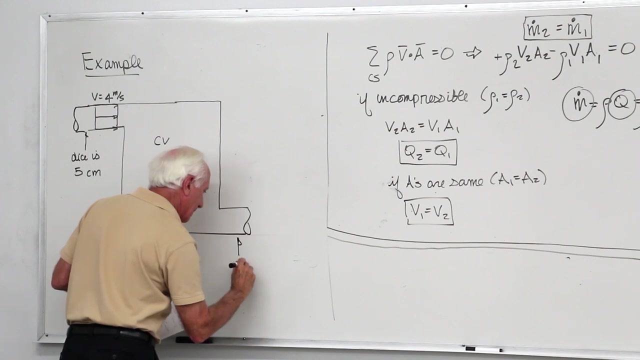 velocity is four meters per second. The diameter here is five centimeters, The diameter here is eight centimeters. Flow comes out, but it comes out. Make more room here. It doesn't come out uniform. This is our first example of something where the flow is non-uniform. 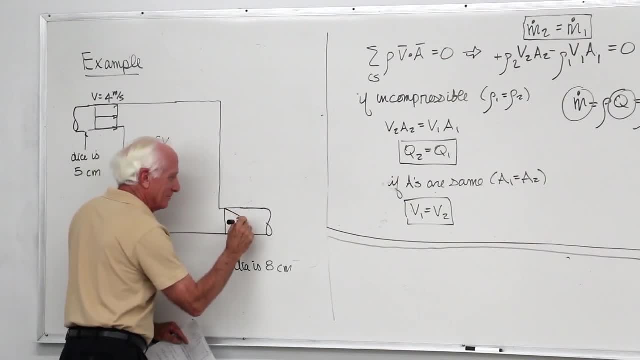 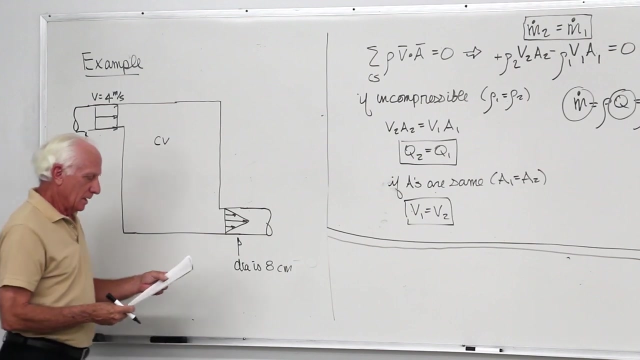 When the flow comes out. this is an approximation. It comes out like this: It's linear. It's linear with the distance from the center line to the outside of the pipe wall. there The middle velocity is V naught, The center velocity V naught. It means that's where the radius. 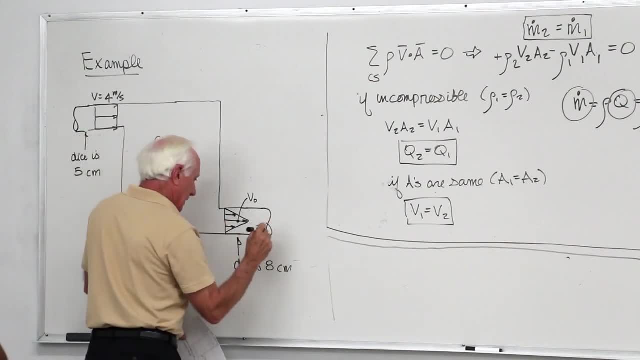 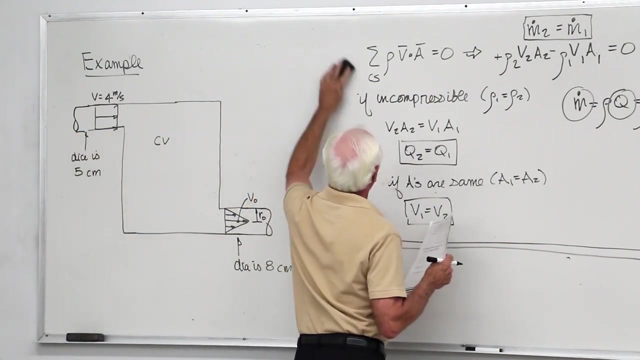 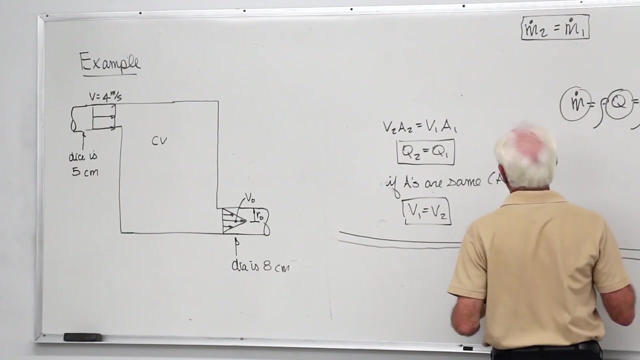 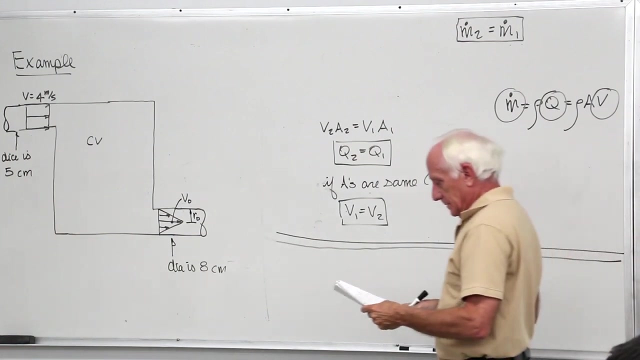 is zero. That's where the V naught comes from, And we know that the radius is four centimeters. We call this R naught. We measure the radius, of course, from the middle. Okay, Let's see here. Oh, let's see, We're close to find V naught. Okay, find V naught. Conservation. 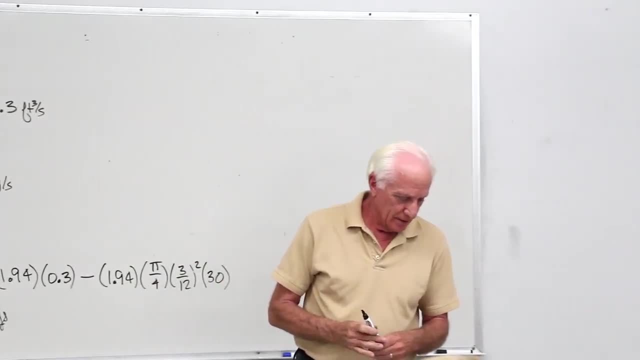 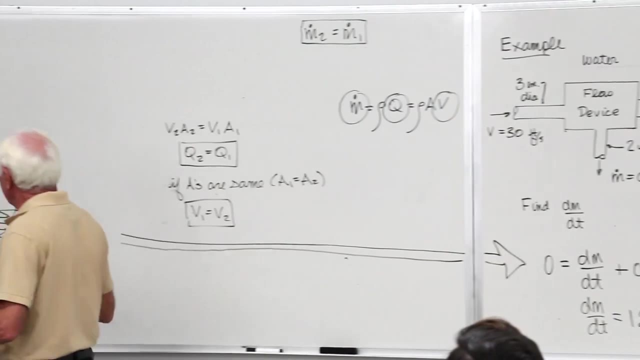 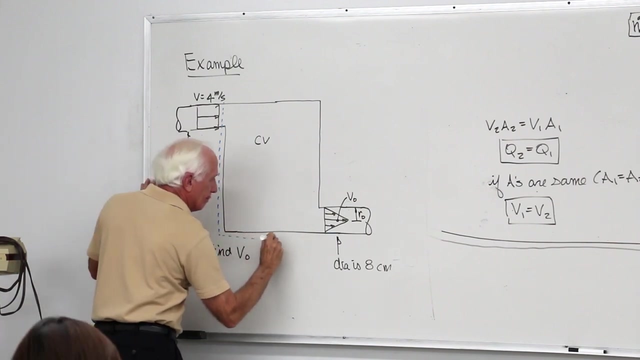 of mass. Okay, When you do that, you always have to define a control volume. So obviously I'm going to take my control volume here. This is my control surface. I'm going to take my control surface, Okay, Okay. 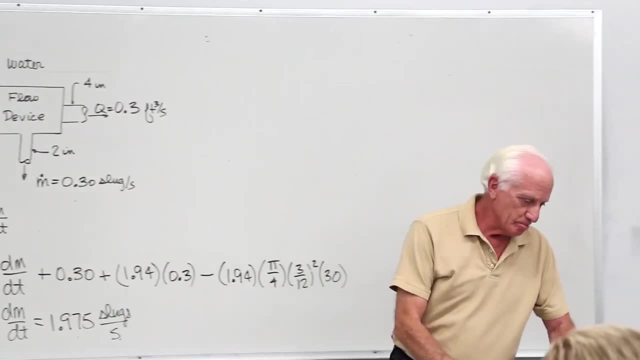 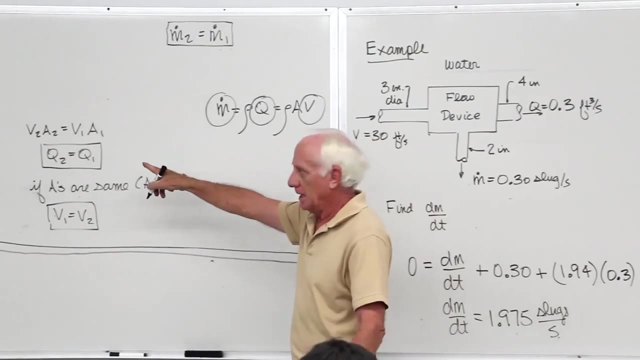 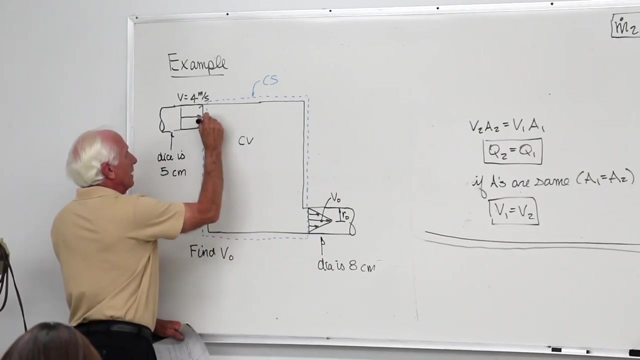 Okay, Okay, Once you do that, you've always got to put some numbers on it, Identify things. Okay, I told you. One is normally where the fluid comes in. I'm going to call that 0.1.. And two: 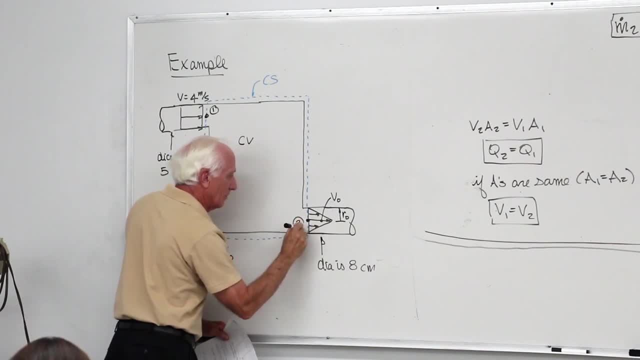 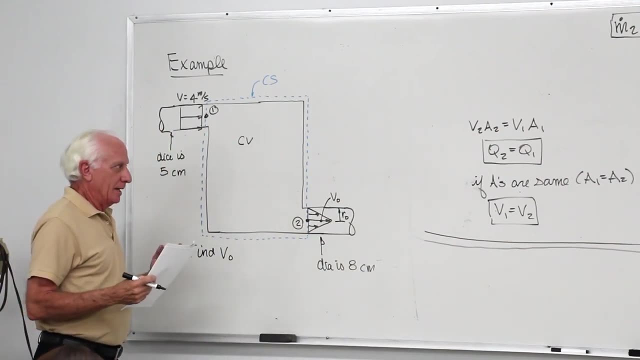 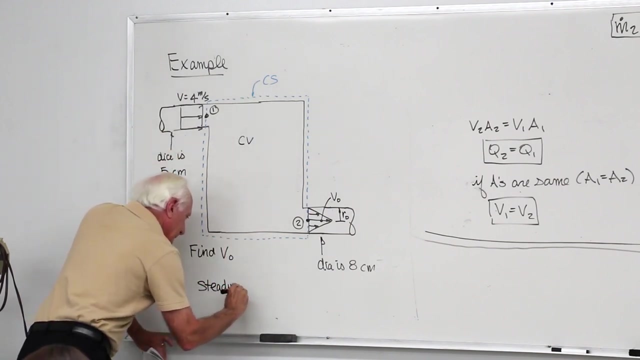 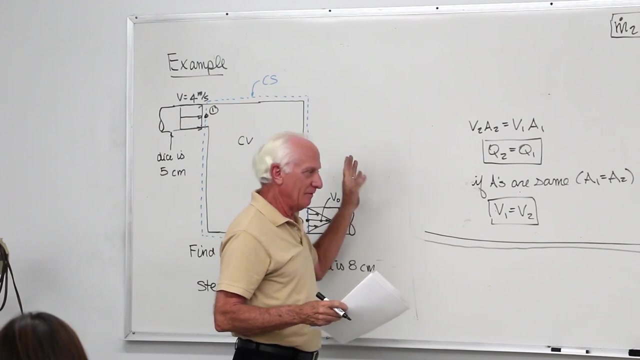 is where it goes up. I'm going to call that two: Okay, Okay, Okay, Okay, Okay, It's steady-state. Okay, steady-state means that left-hand side goes to zero. nothing in the period of time, nothing here. This term goes to zero. Okay, it goes to zero. 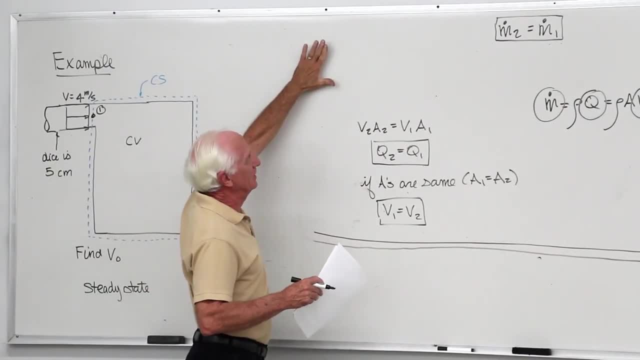 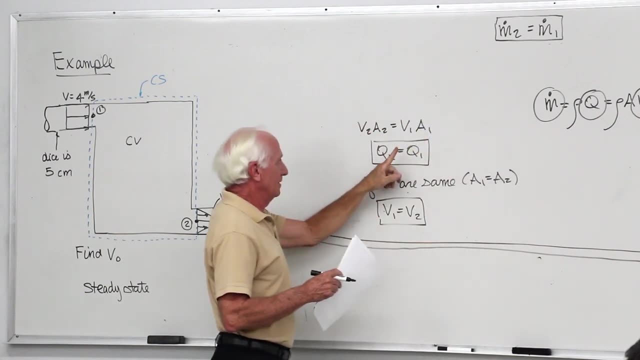 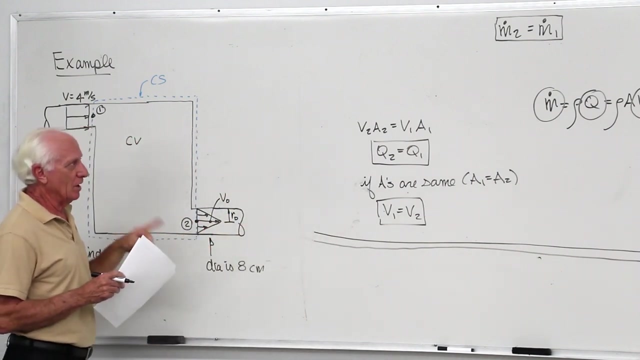 I erased it here, but that's what I said. I said, if it goes to zero, what's conservation of mass or continuity? That one. What if it's incompressible? This one. What if it's the same area? This one. But I said that's only for uniform flow. 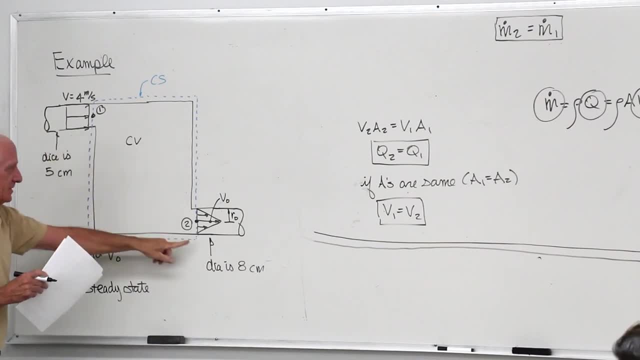 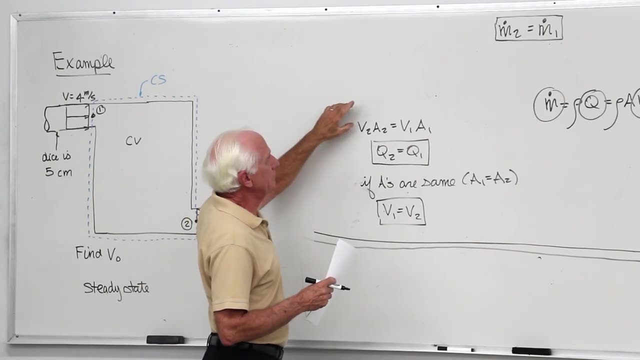 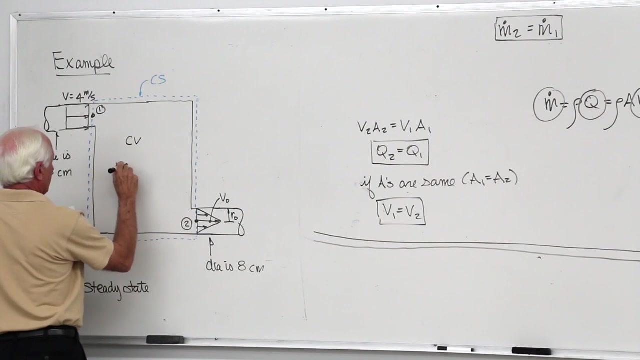 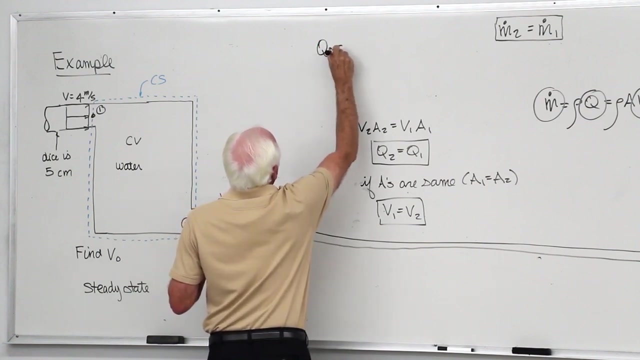 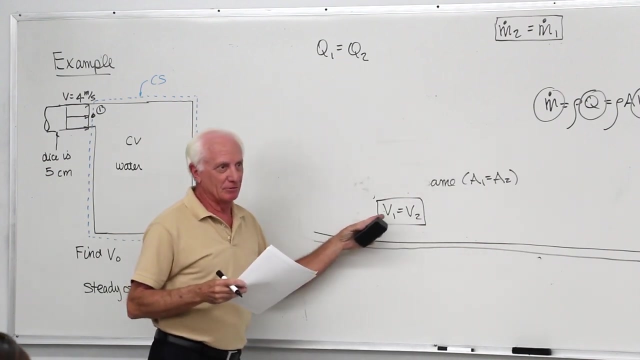 Uniform flow. This is uniform. This is not Okay. So for this problem: it's steady. Okay, It's incompressible, It's water. Okay, There it is. Q1 equals V2.. Okay, Obviously V1 is not equal to V2.. 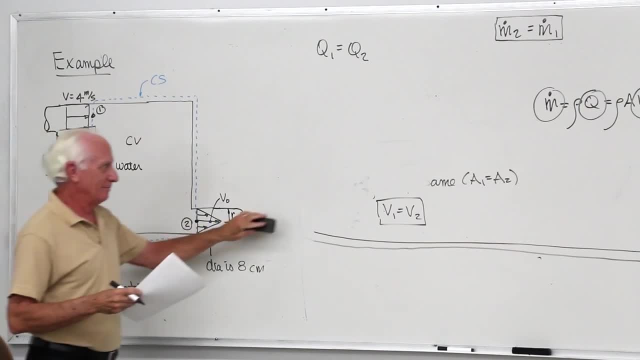 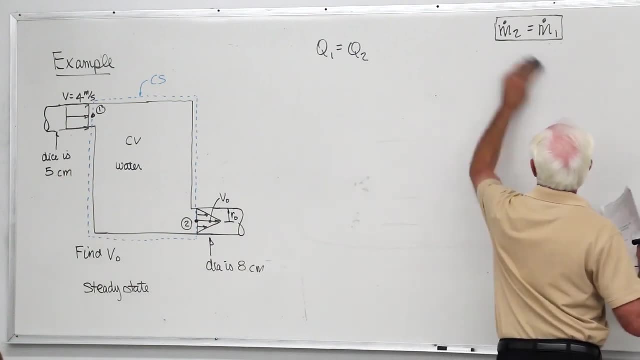 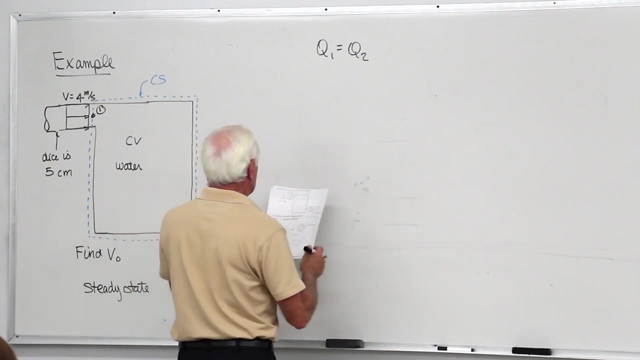 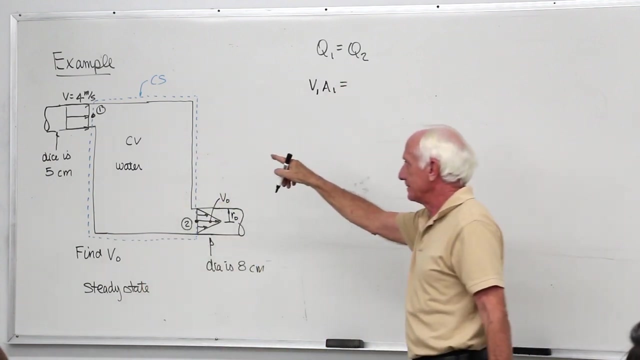 Look at that picture. No, they're not the same. What is V2?? V2 is the average velocity, And you can find the average velocity. Yeah, we'll do it this way, Okay, Okay, So let's go ahead and Q1 is V1A1.. Why is it that simple? Because it's a 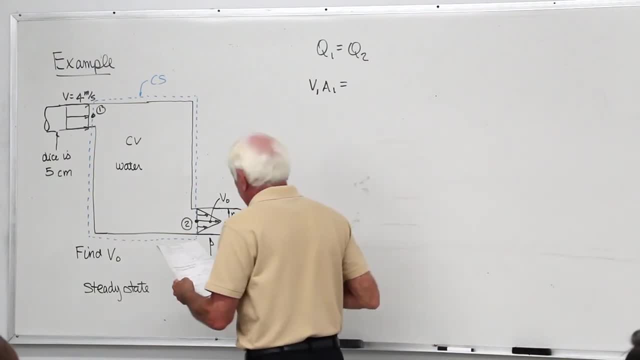 uniform profile. That's equal to Q2.. Okay, Q2.. Integral Vr. 2 pi r, not Vr. That should be 2 pi r, I think. Yeah, 2 pi r, not R0.. 2 pi r. 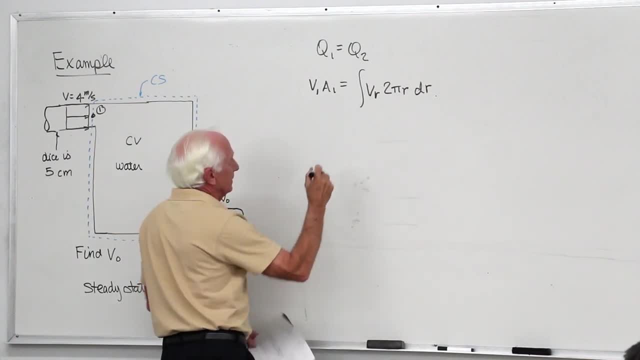 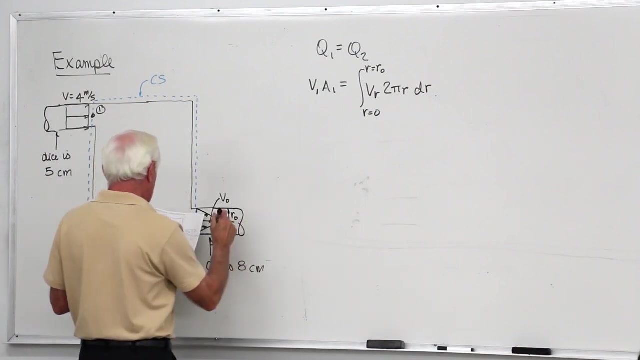 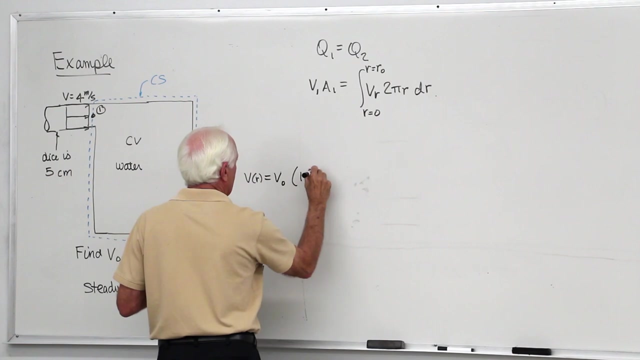 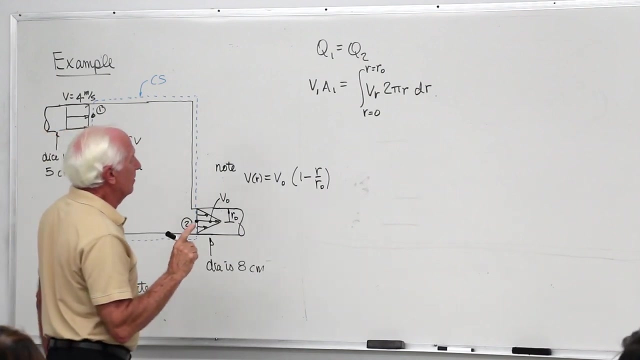 Okay, This is from R equals 0, to R equals R0.. And let's put the velocity down here: V as a function of R0 equals 0.. V as a function of R0 equals 0.. Okay, of R is equal to B knot 1, minus R over R knot. Now let's first of all find out why this integral. 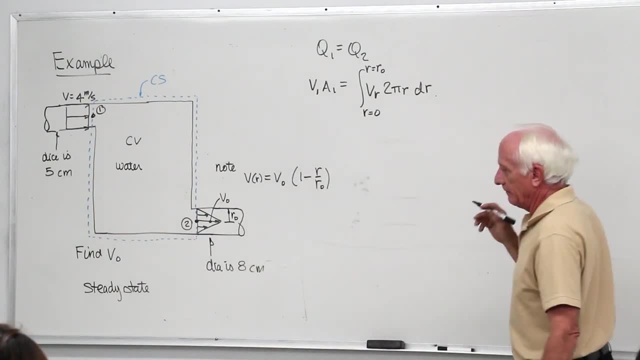 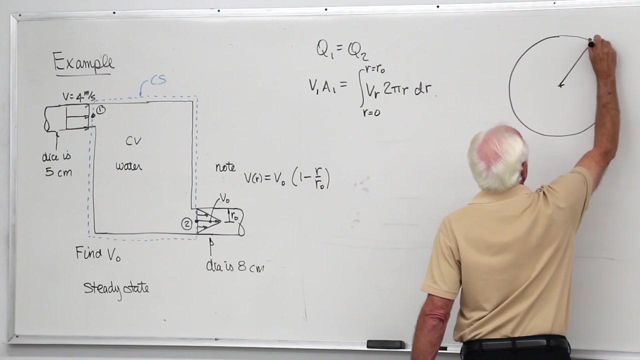 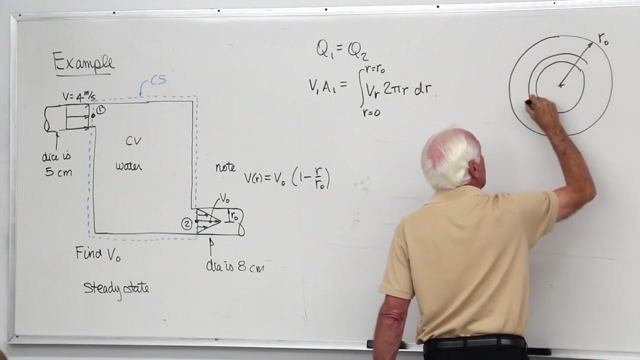 is Q2.. What is Q2?? Volumetric flow rate. What does that mean? Multiply a velocity times a differential area. Here's the pipe. Here's R knot. I take a small differential area like this. I'm going to look at the flow through that small differential area. 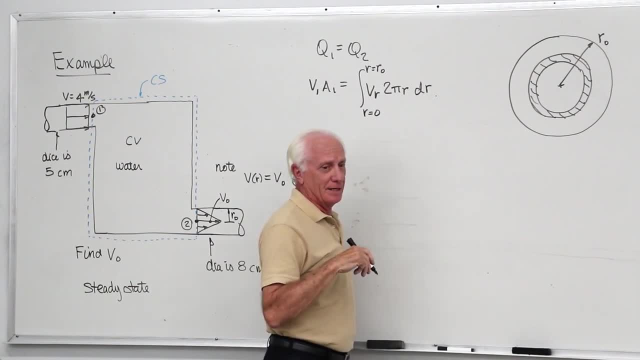 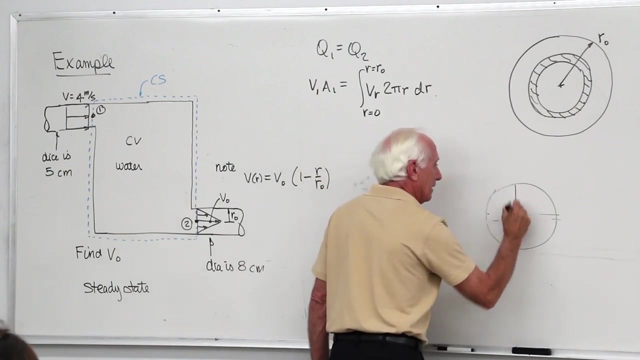 Why do I draw a shape? Because it's a natural shape, It's a cylindrical object, It's a pipe. You wouldn't. you would say, well, I'll take my differential area like that. Oh, I hope not, Man, that'd be tough to do. Or I'll take it and I'll make it a strip. 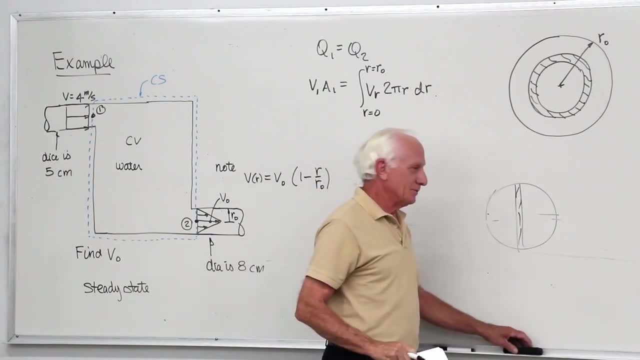 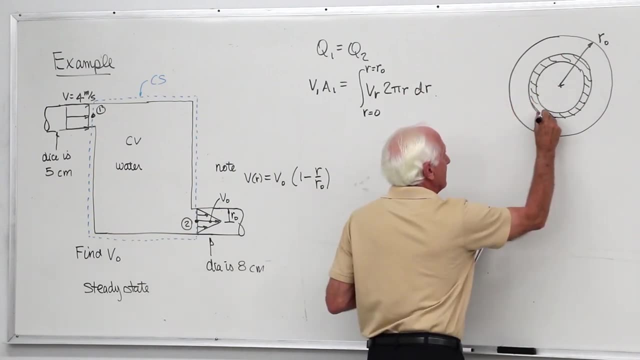 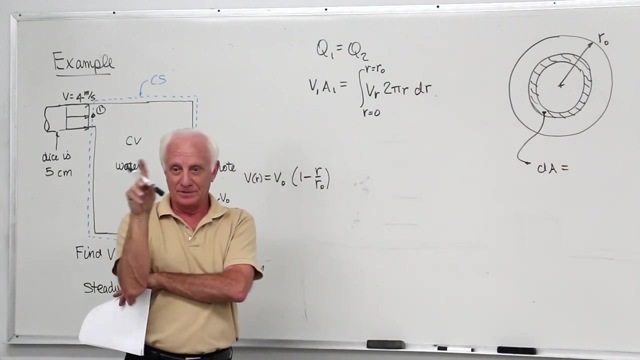 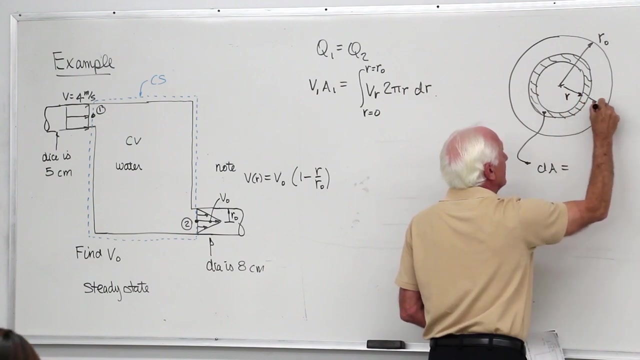 like that. No, no, that's not the right way to do it. Do it the natural way. If it's cylindrical coordinates, like a pipe, then take your little differential area DA like that. What is that? DA? It's the circumference times. how thick is it? Now here's R, The 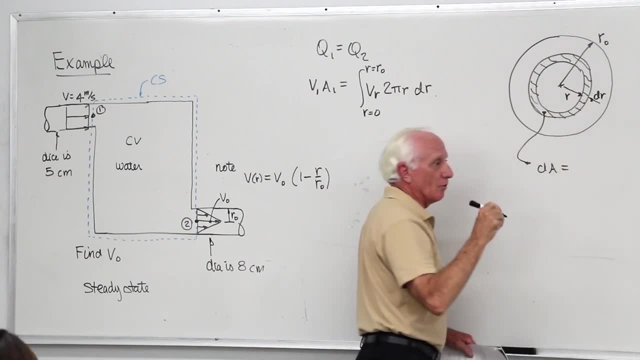 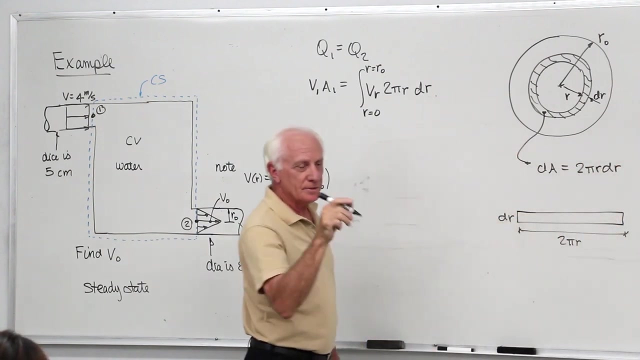 thickness is DR. So circumference is what. 2 pi R Thickness is what DR. You want to pretend it's a strip like this. It's DR here by 2 pi R here, So 2 pi R DR Question. I think I answered it. R, is R a row or R naught Outside radius? 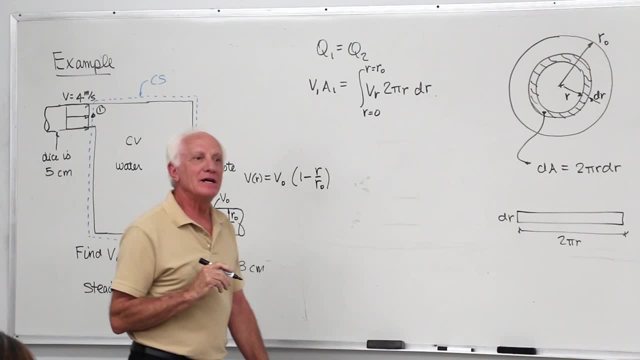 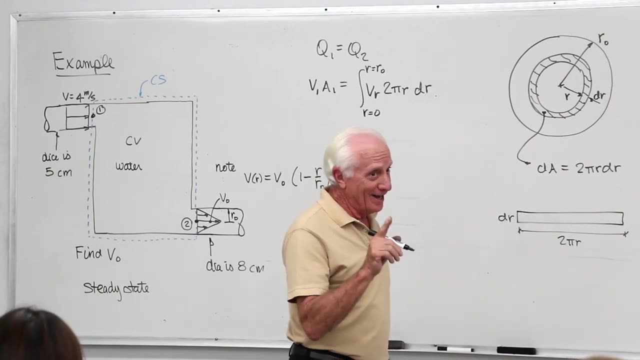 It's from the center And R is just a value that we kind of. R is a general value. You give me R. R is a tenth of an inch, I'll point it. R is a quarter inch, But R naught is 4. 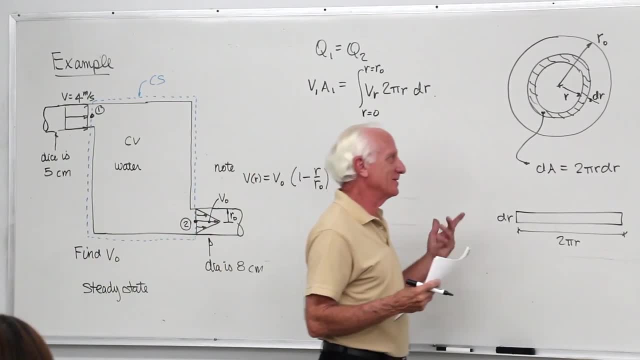 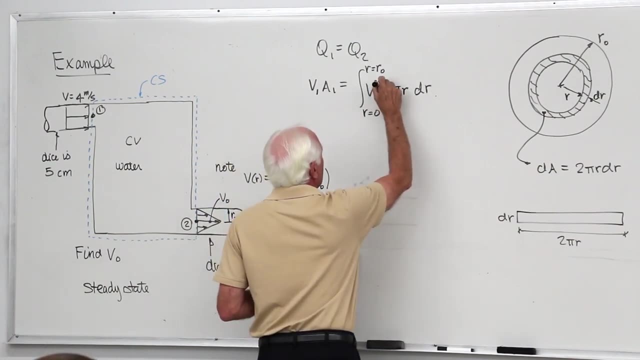 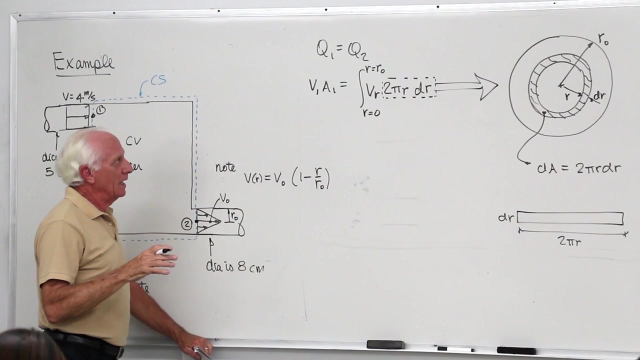 centimeters, Right, Okay, The limits of integration are going to be from 0 to 4 centimeters, So that's where this thing came in. So multiply an area by a velocity and you get a volumetric flow rate, And then 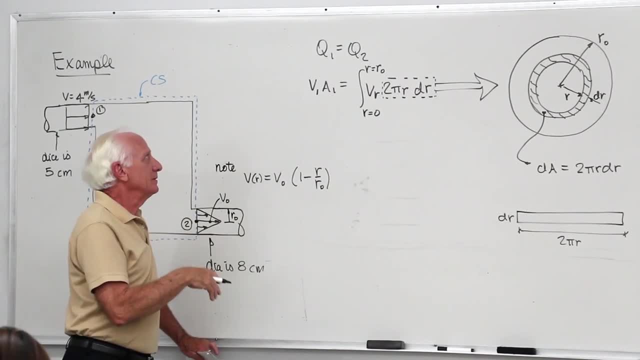 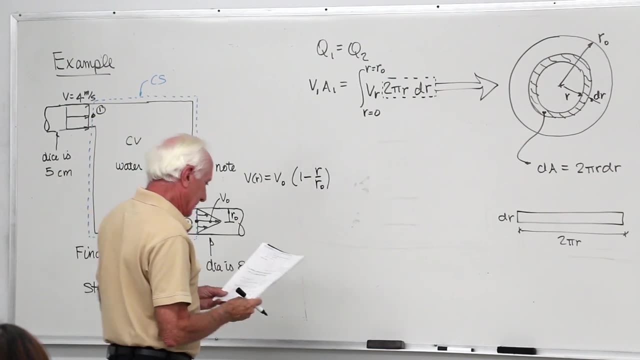 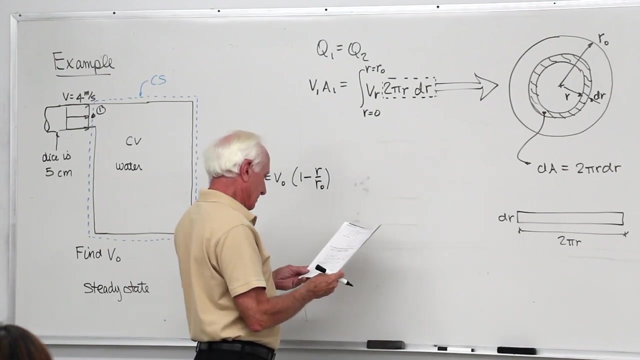 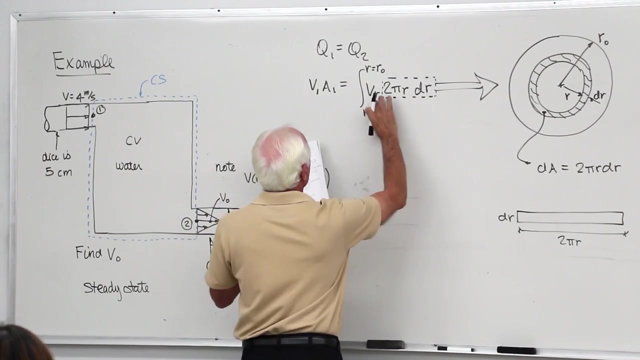 you integrate it from the center line- R equals 0, to the outside radius, R naught. Okay, I think that was the main point I wanted to make: how you treat non-uniform areas, Just so you know when you're done. this is V, This is dot, dot, dot, dot dot 2 pi V naught. 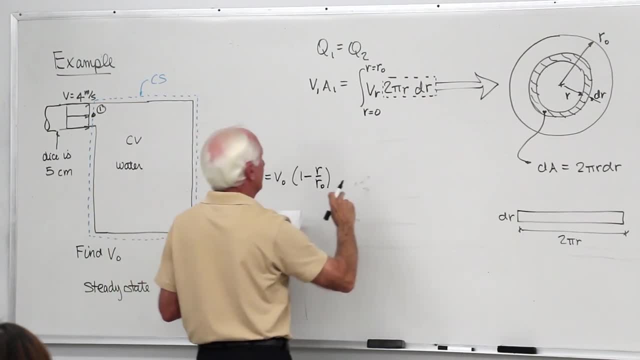 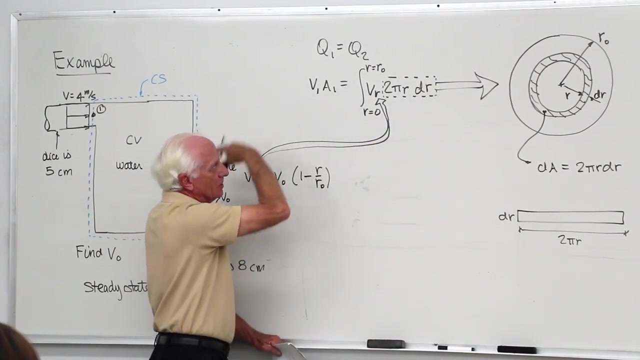 That's V naught right there. V naught dot, dot, dot dot. So I put this V? R up here And I've got that guy there. There's an R, There's an R D R, The rest of it All constants go. 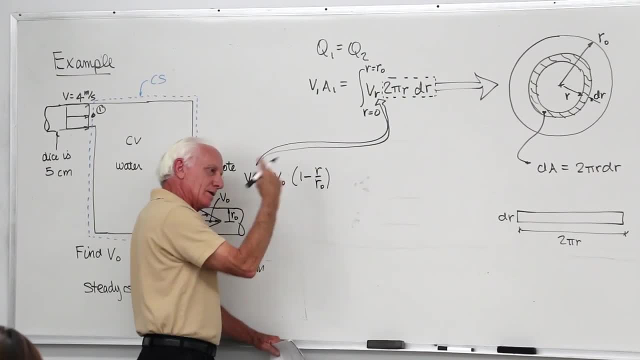 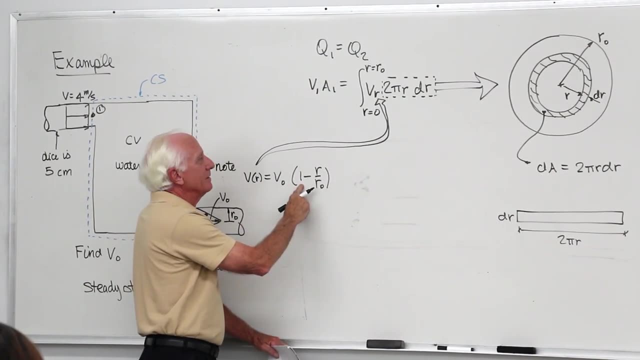 outside. 2 pi comes outside, V naught comes outside. Integrate R squared D R for this guy. Integrate R D R for this guy. Plug the limits in R equals 0 to 0.04 meters, 0.04. 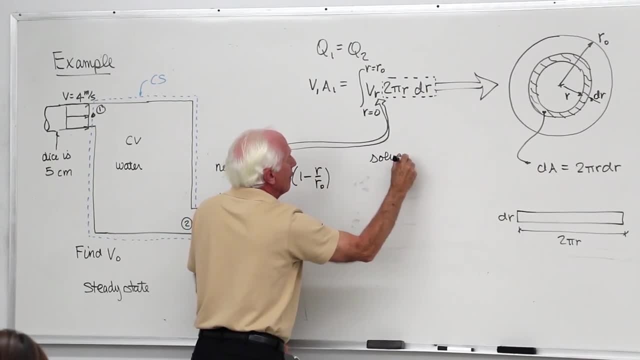 meters. Okay, So that's how far V naught. 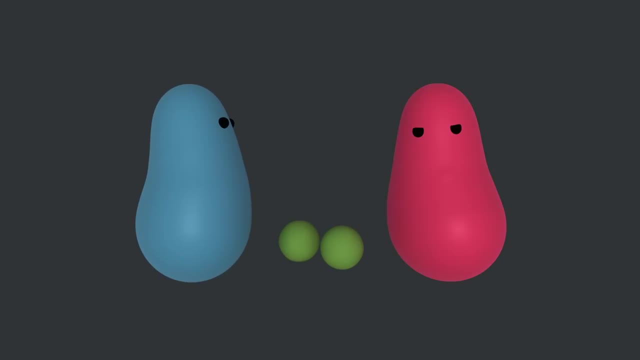 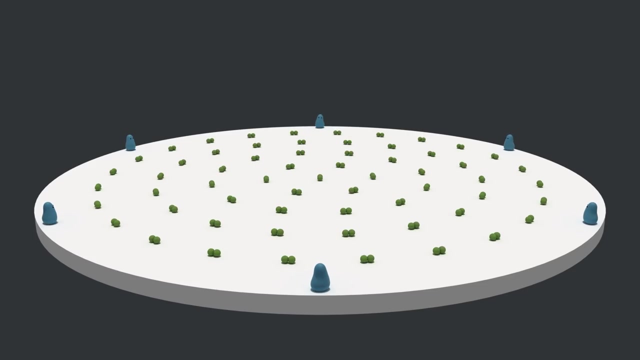 In this video we're going to start exploring conflict between creatures To try to build some understanding. here we're going to use some simulations and some ideas from a field of math called game theory. Okay, so in our simulation, food will appear each day and then blobs will appear and go. 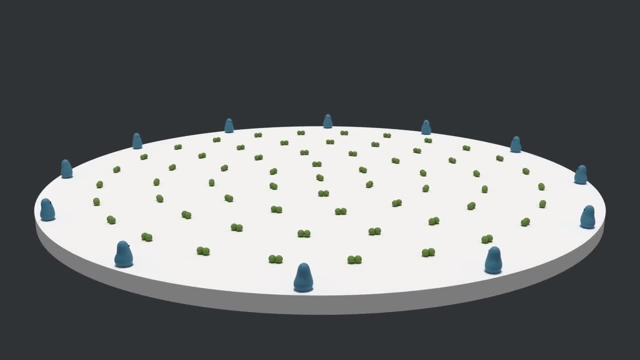 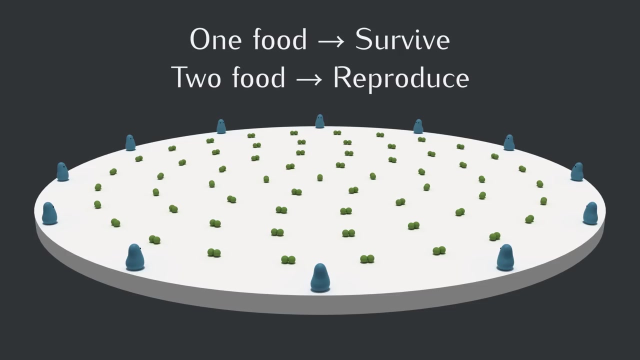 out to eat the food. We'll use the same survival and reproduction rules as in previous videos. Eating one piece of food lets a creature survive to the next day, and eating two pieces of food allows a creature to both survive and reproduce. What's different in this simulation, though, is that food will come in pairs- Each creature